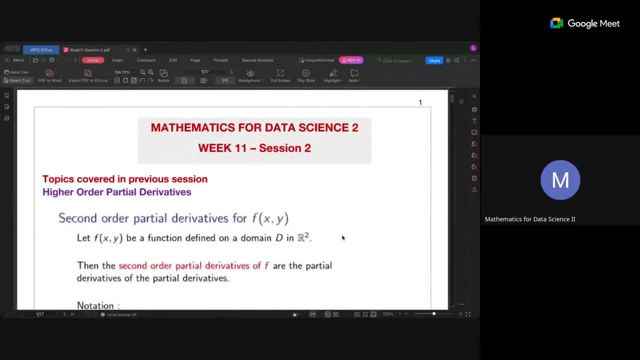 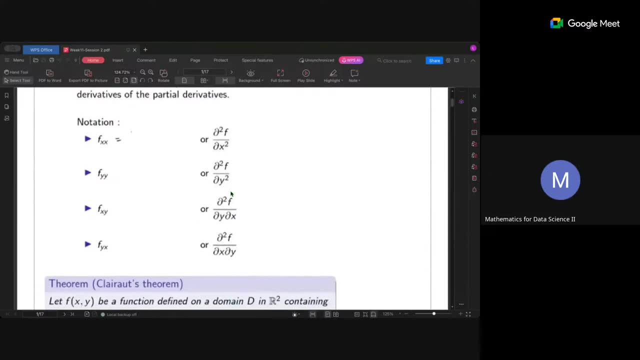 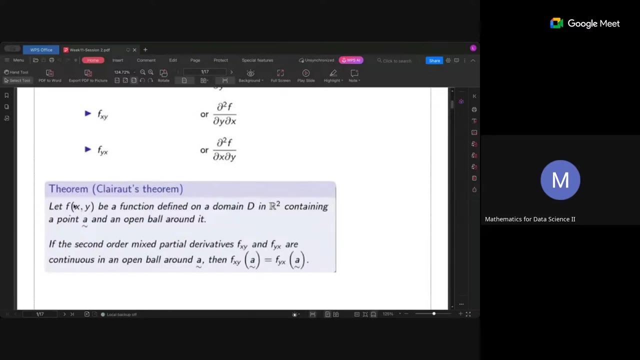 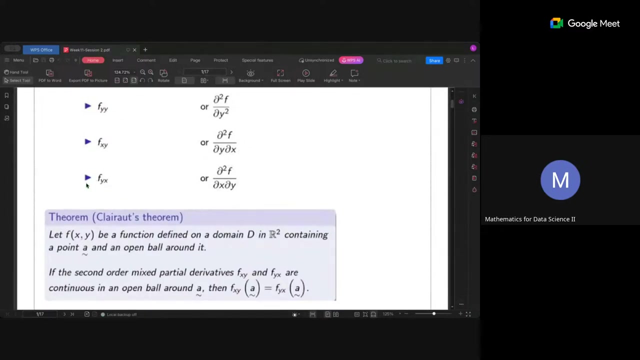 Yeah, So you have these different types of representations for mentioning the higher order derivatives. And what does Clorid's theorem say for higher order derivatives? So suppose you are having. so these kind of derivatives are called mixed derivatives, right? So these are mixed partial derivatives. So Clorid's theorem is mainly about this mixed partial derivatives. 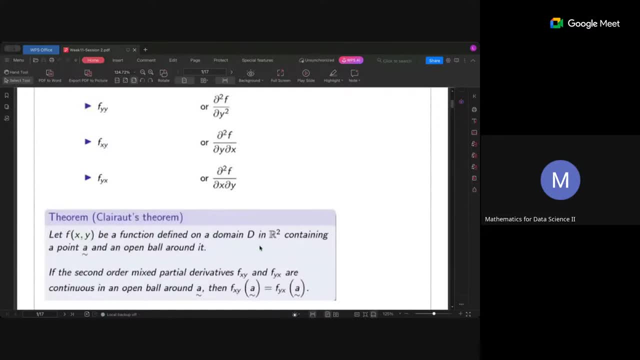 So if you have a function of two variables on a domain D in R2, containing a point, a tilde and an open ball around it, Okay. So if you have the mixed partial derivatives fxy and fyx continuous in an open ball around a tilde, then fxy at a tilde is equal to fyx at a tilde. So usually we you might have noticed in several functions you can interchangeably use fxy and fyx. you in general assume that. 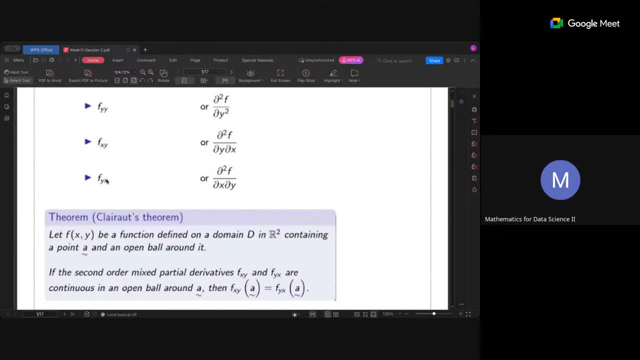 they are equal. but you have to be careful, mainly when it is in the case of piecewise functions. So there you have to be more careful. So in those scenarios you may have a situation where the fxy and fyx need not be continuous in an open ball around it. In that scenario, you see that the mixed partial derivatives may not be equal. at that point, Okay. So in general, the continuity of fxy and fyx. you might have a situation where the fxy and fyx need not be continuous in an open ball around it. In that scenario, you see that the mixed partial derivatives may not be equal. at that point, Okay. So in general, the continuity of fxy and fyx. you might have a situation where the mixed partial derivatives may not be equal. at that point, Okay. So in general, the continuity of fxy and fyx. you might have a situation where the mixed partial derivatives may not be equal. at that point, Okay. So in general, the continuity of fxy and fyx. you might have a 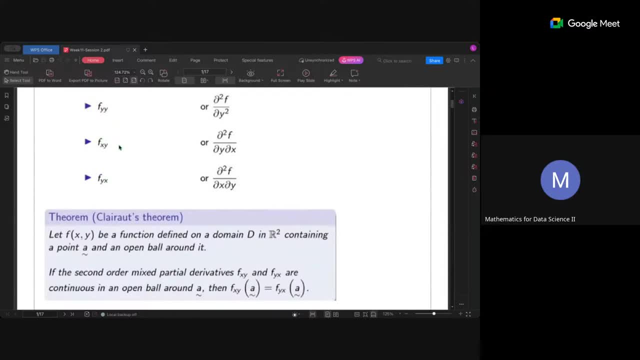 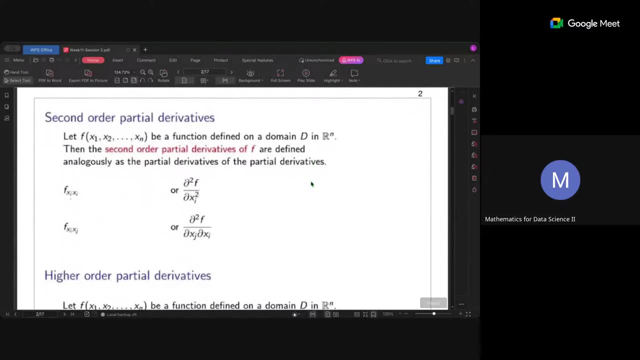 x at a point guarantees the equality of the mixer partial derivatives at that point. ok, So this is for functions of two variables. So the same can be extended for functions of n derivatives, n variables. ok, So if you have a function of n variables, you know. 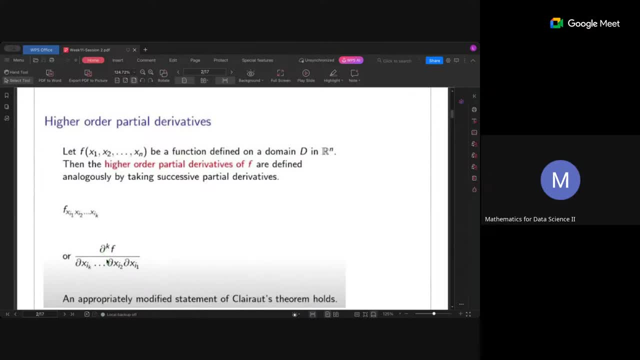 you can keep on doing the partial derivative and get higher orders of partial derivative. So as appropriately modified statement of Claret's theorem whole it means what? so in that case maybe, for example, if there is three variable, then you have to say f. 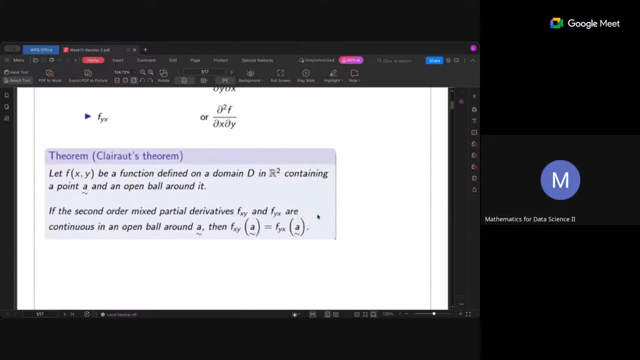 x, y z, f y, y, x z, and maybe one more term, maybe f, z, x, x, y. So like this, all of them should be continuous around the open volume so that they all are equal. So, like this, you have to write the appropriate terms, because there will be several terms which 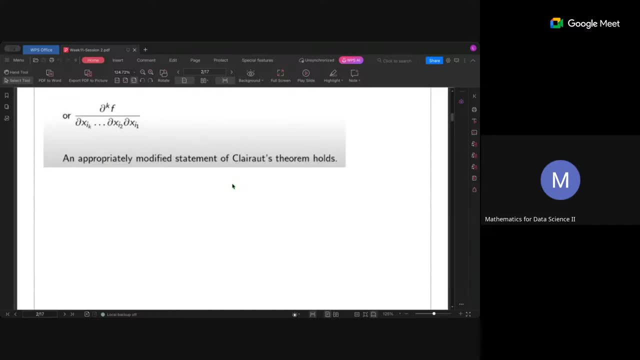 are equal at that point. So you have all those terms. you have to identify and see if they are continuous at that point to give the equality. ok, fine, So this is the general introduction to higher order partial derivatives. So, using this, you have to do the Hessian. 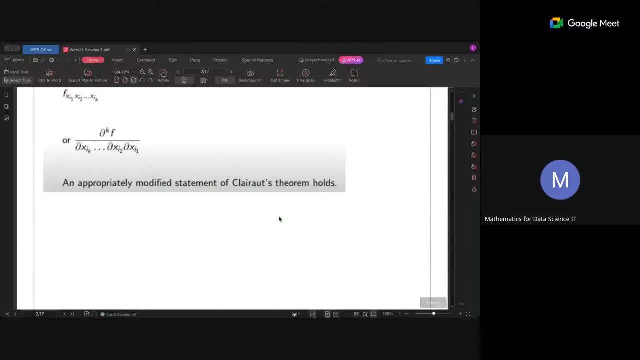 interest. What is the purpose of this higher order derivatives? now, We have seen in the previous lecture, we have seen that the higher order derivative test is a very important thing, right? So, finding absolute maximum or absolute minimum, the global extrema part. 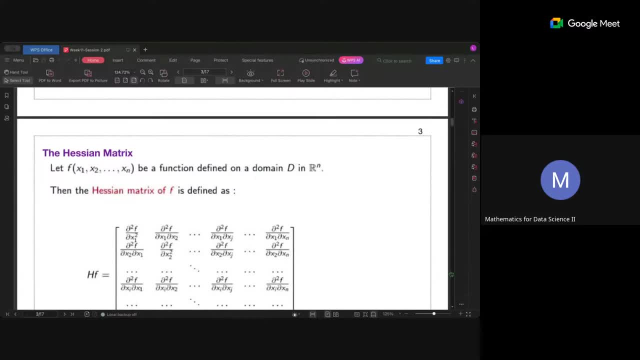 is something completely different. But when it comes to local extrema, classifying the critical points is a very involved task. It is not difficult, but it is quite involved, right? So how to do that? We have seen how do we do that. second order derivative test. in the case of 1,, 2,, 3,, 4,, 5,, 6,, 7,, 8,, 9,, 10,, 11,, 12,, 12,, 13,, 13,, 14,, 14,, 15,, 16,, 17,, 18,, 19,. 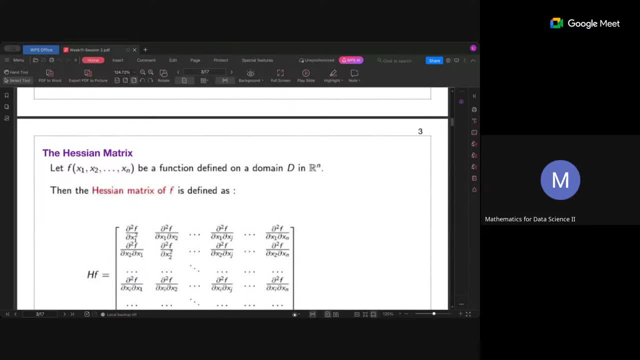 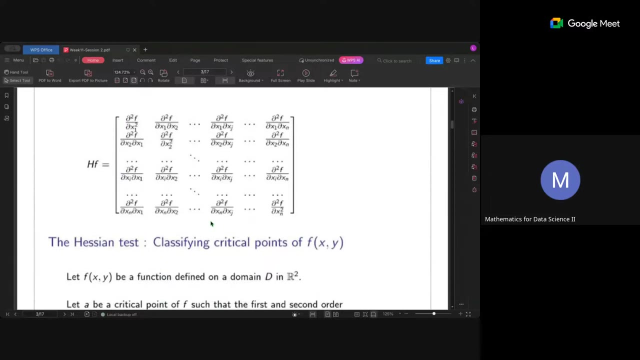 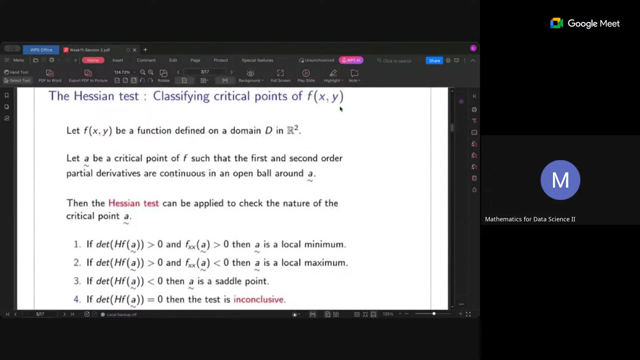 20,, 21,, 22,, 25,, 26,, 27,, 28,, 29,, 30,, 33,, 34,, 35, 36.. There is a part of the derivative aspect called sudahção. 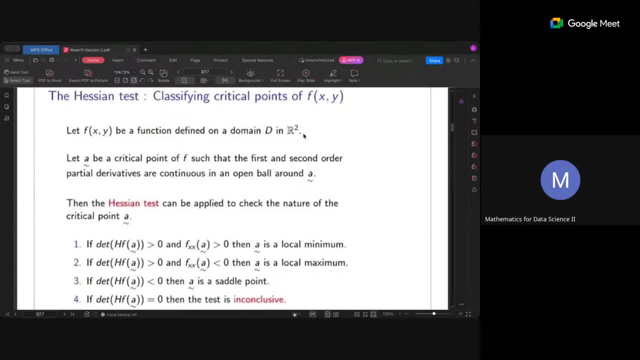 a two variable function f on a domain d in R2.. If a is a critical point of f, such that first and second order partial derivatives are continuous in an open pole around a, okay, So then what do you do? You first have to construct what is your Hessian matrix? So, what is your Hessian matrix? 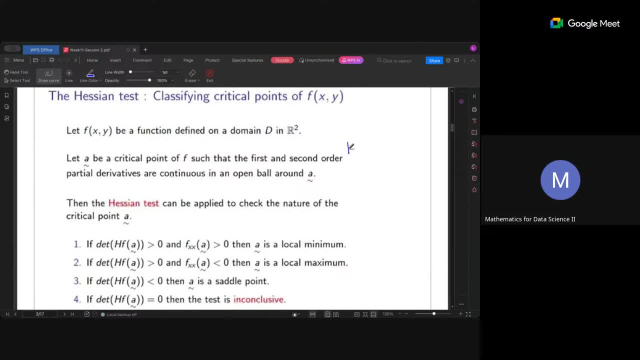 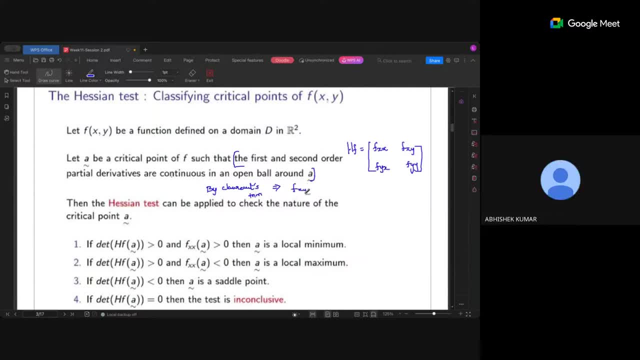 the second order partial derivatives are continuous in an open ball around a till. Okay, So now one condition is given to us: that the second order partial derivatives are continuous in an open, So for at a tilde. you can use this interchangeably, So you don't have to. 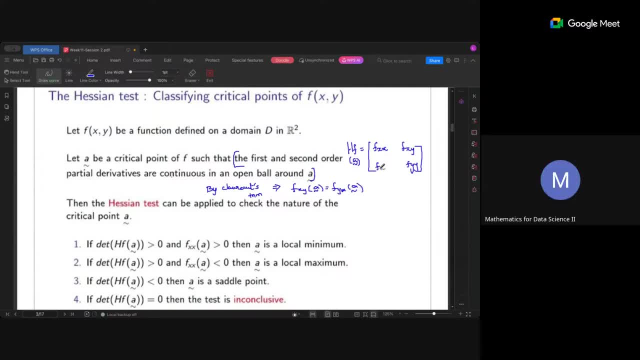 And you, diagonally, are the same, Yeah, So you have x1 here, Okay, And all of them are at a tilde, So you write it like this: So now you see that. what is the special property about this matrix? now, Symmetric. 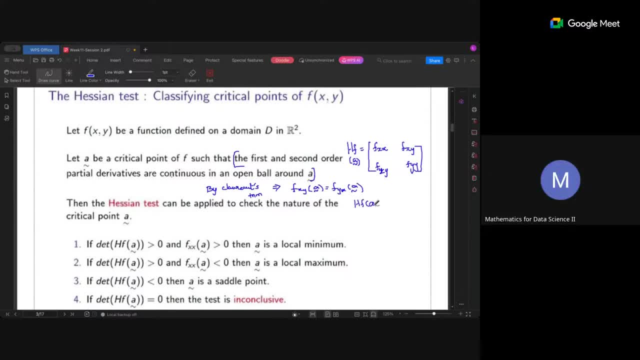 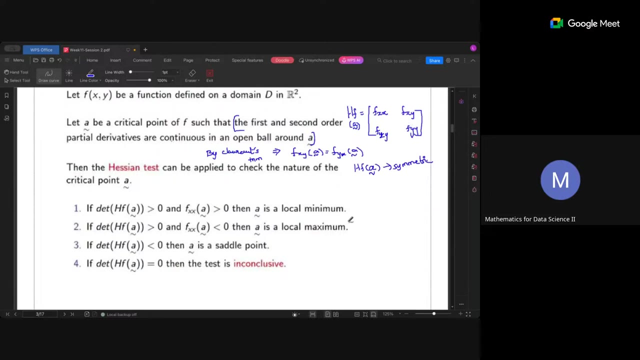 HF of a? Yes, So you should note that HF of a tilde is a symmetric matrix. Okay, Fine, Okay. So then what do you do? You find the determinant Right. So what is the step 1? 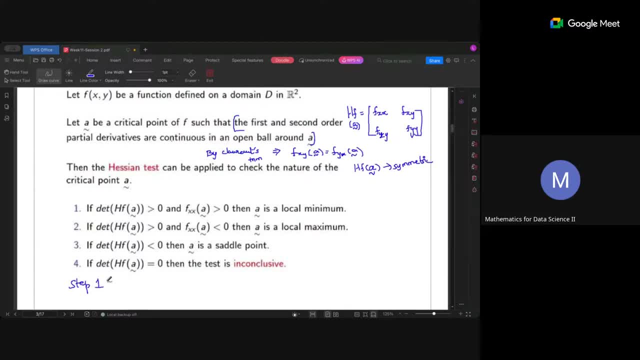 here, Step 1. First you take the determinant of the symmetric matrix. Yeah, First you have to find HF of a Right. So, after finding HF of a tilde, what is that you do? You find the determinant, Determinant, Determinant of HF of a tilde, Right. So if 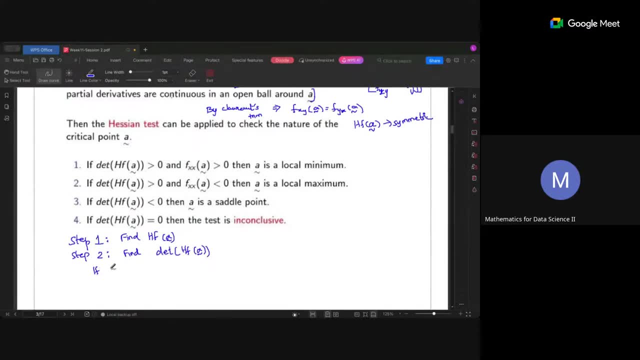 HF of. if this determinant, HF of HF of a tilde is 0, then Inconclusive, For says test is inconclusive, Inconclusive, Right, And if the determinant is negative, then Sadder point. 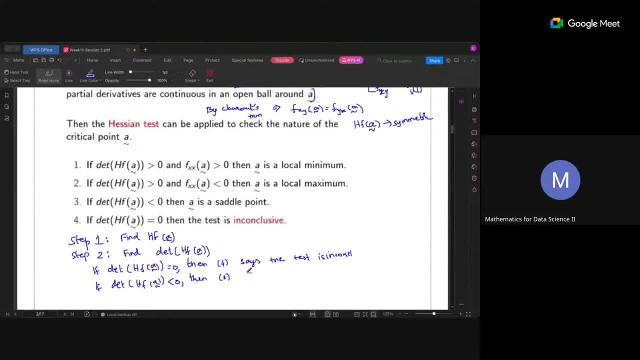 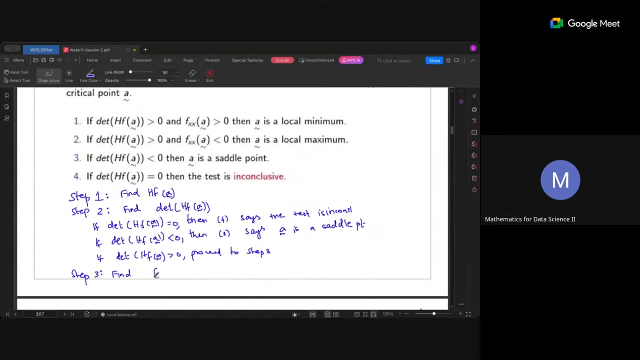 Yeah, Three states. a tilde is a saddle point, And if determinant is positive, then you proceed to step 3.. Proceed to step 3.. So what is step 3?? Step 3. Find Fxx at: 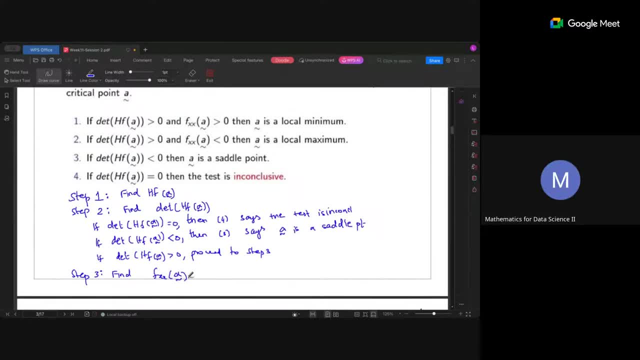 A tilde. Okay, So if it is positive, then A tilde is a Local minimum, Local minimum, And if it is negative, Then A tilde is a minimum Minimum, Maximum. Right, So these are the steps involved in classifying the critical points of a function of two variables. 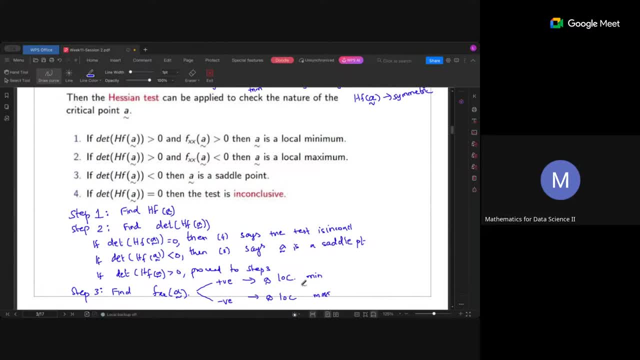 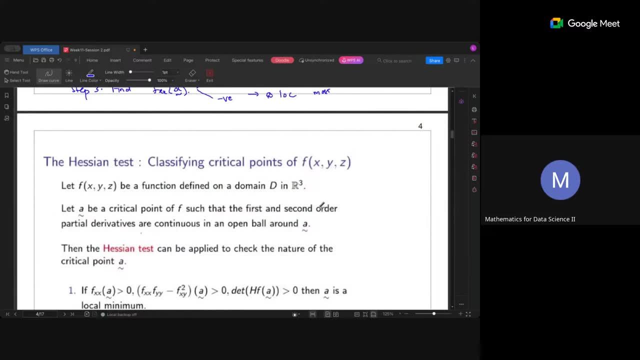 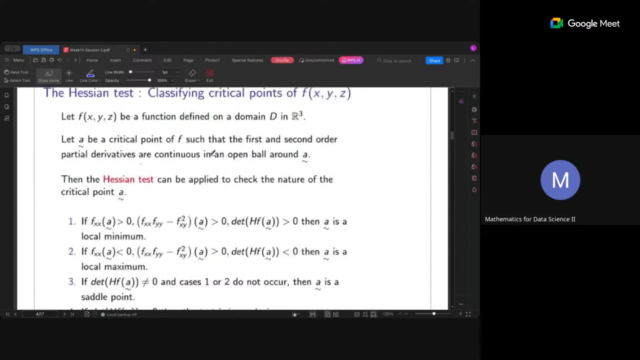 Alright, So you have three steps here. So you have seen examples for this, And now we are going to see similar process For classifying critical points for functions of three variables. Alright, Okay, So let F of be a function defined on a domain B in R3.. Let A tilde be a critical point of F, such that Legitimate ad souvent dance to the fraction given by mads, cioè府 and subkalements to a subordinate 스메 and related adversities. Let A tilde be a critical point of F such that the first and second order partial derivatives reflect the term對啊. participants are supposed to have only one particle, while adjoining the particle and collective addition in the derivative. 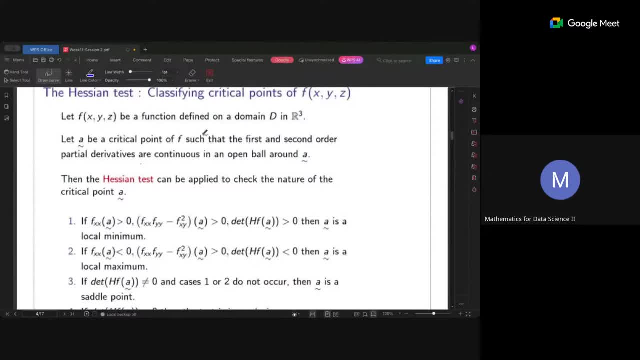 So you have three steps here: partial derivatives or continuous in an open ball around A. So here also we are having the assumption that you have the mixed partial derivatives, that those pairs, So for example fxy and fyx, are equal at A tilde. Similarly fxz and fz. fxz and zx are equal, then fyz and fzy. 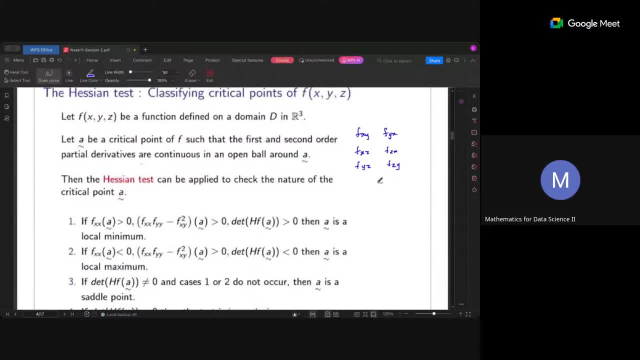 So these kind of pairs you can pick and see that they are equal right. They are equal at A tilde, Not in general, at A tilde they are equal right. Okay, So now here, what is the Hessian? 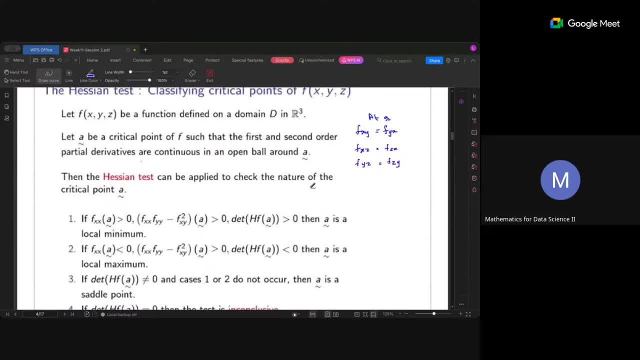 matrix. Before this, let us write: what is the Hessian matrix now? So what is the Hessian matrix at the point A tilde, Can you tell xx, f of xx, then f of xx, then f of xx. 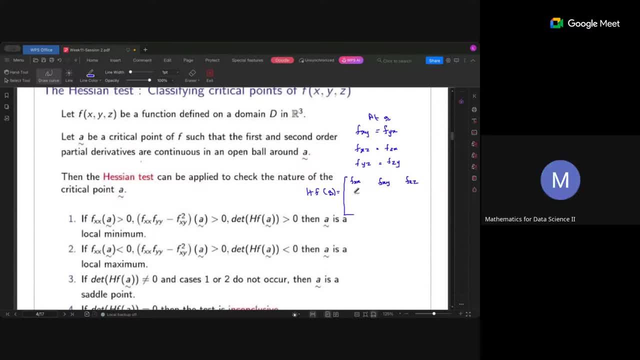 f of xy, then f of xz and yx, f of yx, f of yy, f of xy, Which is same as f and xy, right, Because we have the continuity condition. Yes, ma'am, Yeah, And here yy, f of yz. 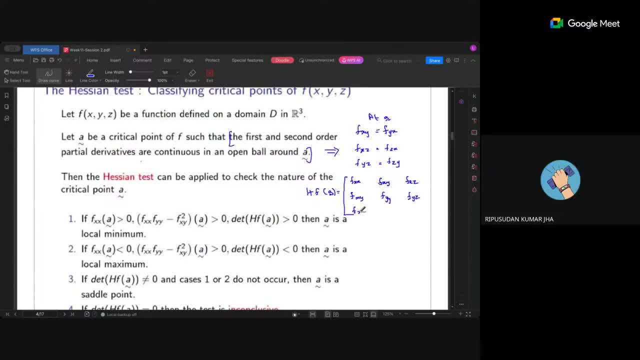 yz, And here f of yz, f of xz, Which is same as xz, And here zx is same as yz. yz, then f of zz. Yeah, So this is the Hessian matrix you are going. 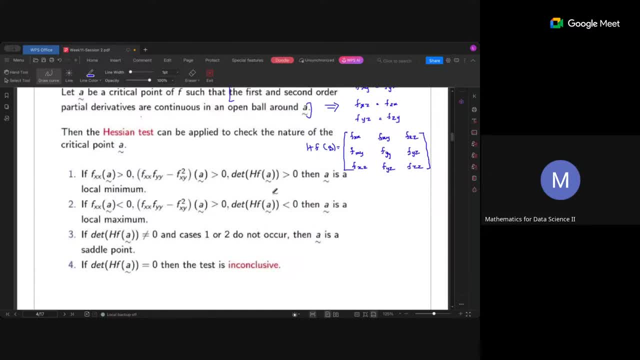 to consider right. So now, maybe we will give some variable, maybe like alpha, maybe this we call as beta and this as gamma. Okay, Just for convenience, instead of writing the entire term, Okay, Just let us give some variables for each of these. So let us give some variables. 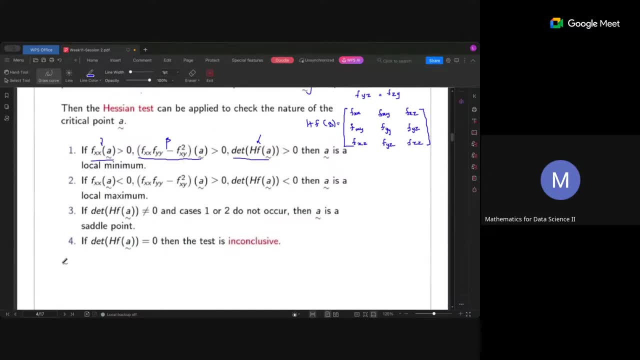 for each of these. So let us give some variables for each of these. So let us give some variables for each of these terms, so that it is easier to write the steps. So what is your step one? as usual, Find the Hessian matrix, first of all, Right. So once you find the Hessian 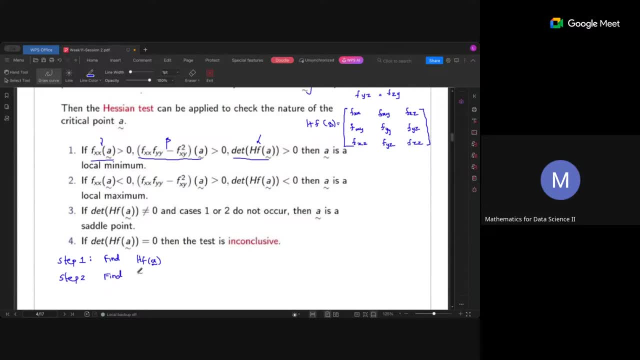 matrix, you have to find alpha right. So if alpha is 0,, the test is inconclusive. Yeah, This is alpha. determinant of hf of a tilde. Okay, The test is inconclusive. Now, if alpha is non-zero, you proceed to step 3.. Okay, So if alpha is non-zero, you proceed. 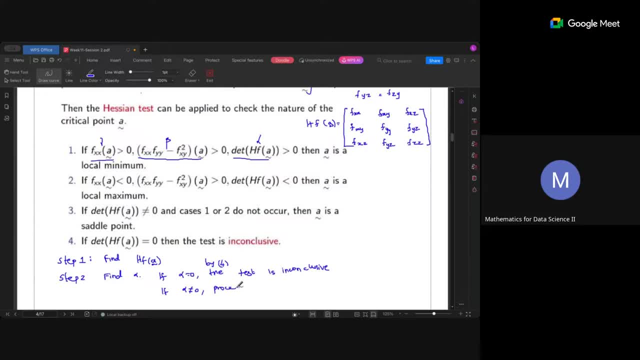 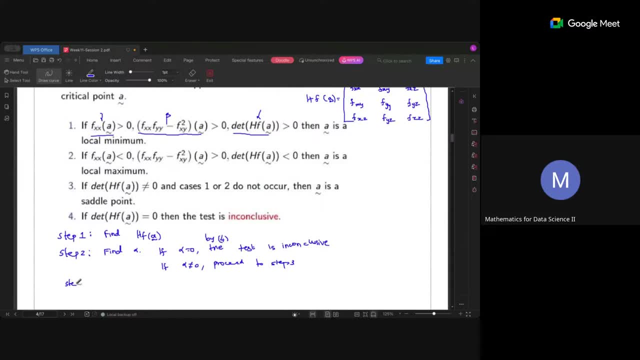 3. Okay, Then what do you do? You have to find what In step 3, you find beta, Right, So you find beta. So if beta is less than zero, then what happens? Only when beta is. 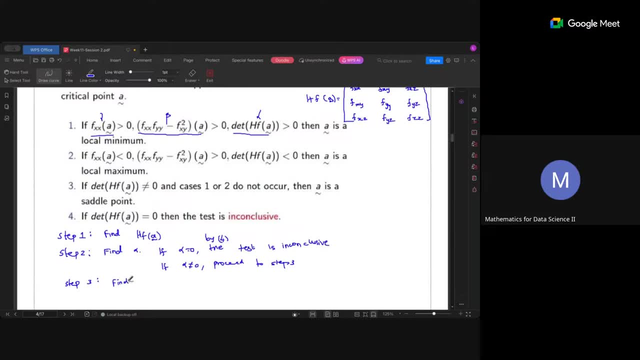 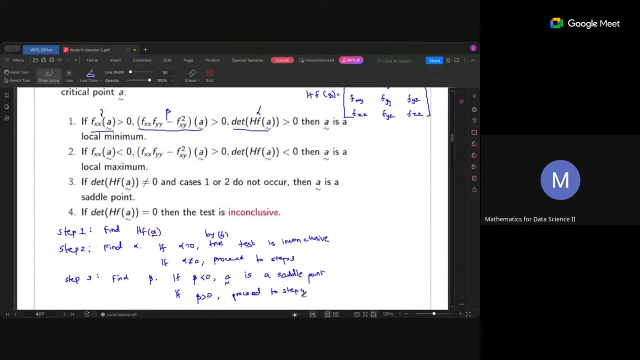 positive. you see that you have a local minimum, or local maximum. So if beta is 0,, then what will happen? a tilde is a saddle point right, and if beta is positive, then proceed to minimum. yeah, then we do the step four. we find what is gamma. 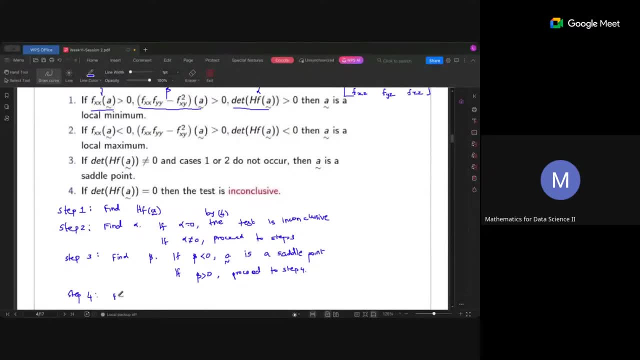 so you find gamma, which is fxx, at a tilde right. so if gamma is positive, then you have a tilde to be a local minimum and if gamma is less than zero, then a tilde is a local maximum right. so we have very less number of cases here. so if you have alpha beta gamma, so what is alpha beta? 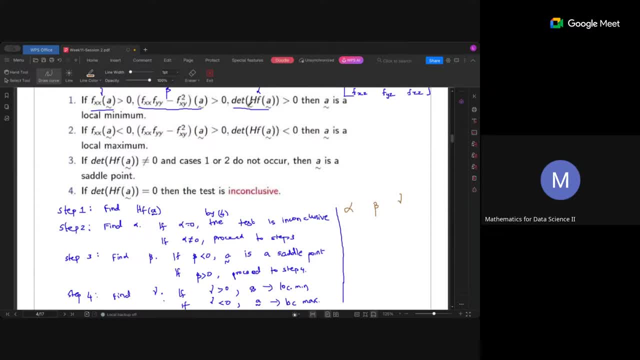 gamma. you just see here, don't think that it is something new. so just these things i have written shortly, right? so what are the only possible cases? first of all, so if this is positive, and this is positive, then you have a tilde right? so if you have alpha beta gamma, then you have a. 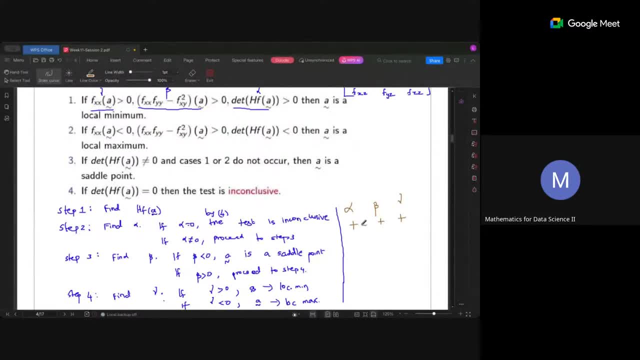 tildeays, also positive, акку company positive and beta vegan. then you have alpha thetaeneca, Viktor, this is also positive, and this is also positive. then what happens? if all of them are positive, then what is that? you get local minimum right. and if the determinant is positive- sorry, if the determinant is negative- 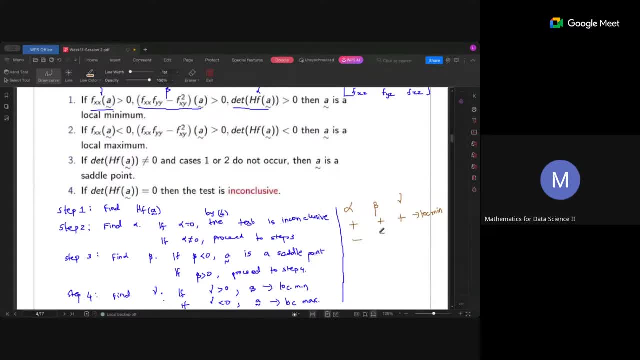 or determinant is negative. this value, beta here is positive, fxx at a tilde is negative. If this happens, then it is local maximum right And here, if determinant is less here positive, negative is fine. So here what happens? If either determinant 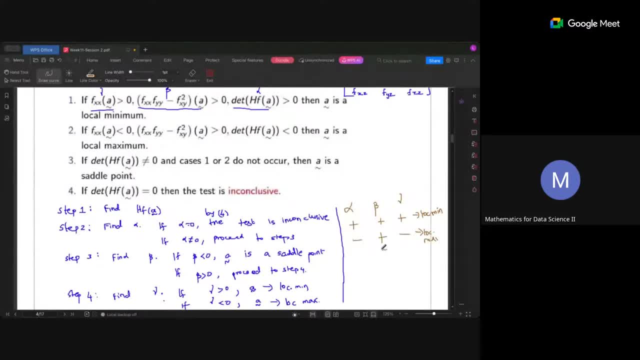 is positive or negative, but this is negative. If this is negative, then it is automatically a saddle point. So here, suppose this is non-zero and this is negative, then whatever is this, this does not matter. okay, It can be plus minus zero anything. Then you know that it is. 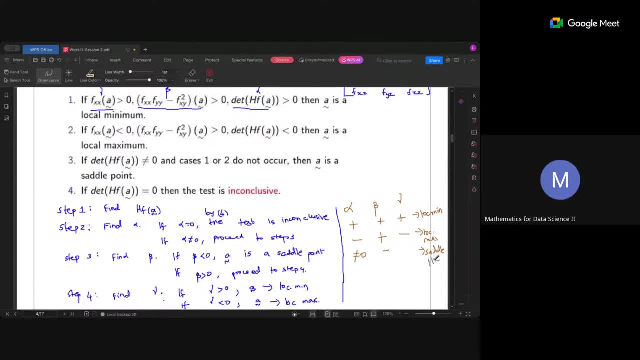 a saddle point. okay, So in all other scenarios this is non-zero and negative. then straight away you write saddle point. Only these three scenarios are there, right? So all other cases, what do you know? All other cases. 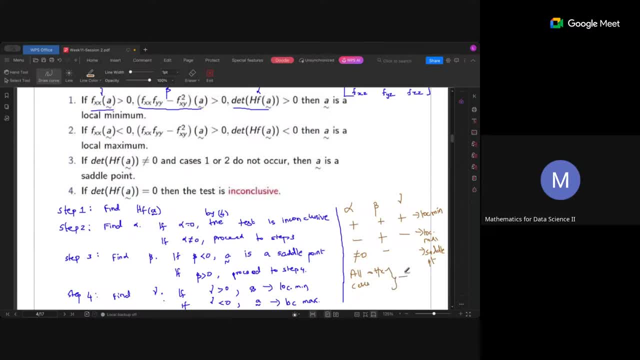 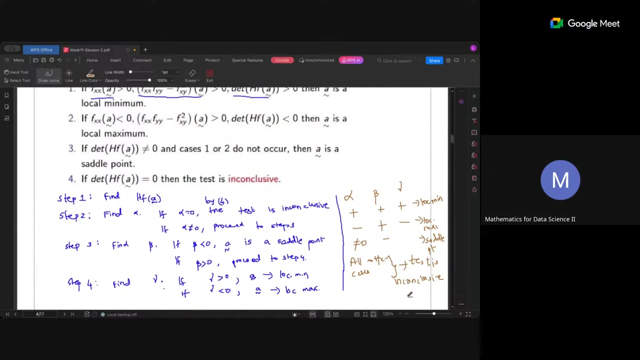 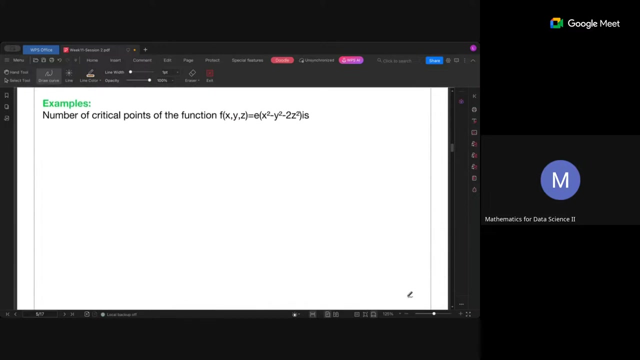 what do you know All other cases? what do you know? Test is inconclusive, Inconclusive, Yeah, Only these three scenarios you know: local minimum, local maximum or saddle point. Okay, Fine, Okay, So so with this let us now solve some problems. So first let us just find the critical points, then we will classify them later. 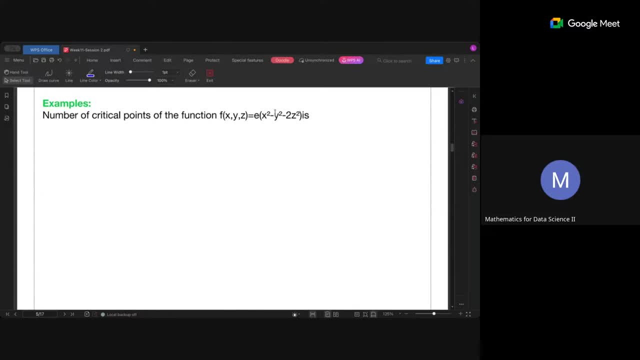 So how do you find the number of critical points for this function We can impact? yeah, Ma'am, where do we find? we have to find the gradient? Yeah, yeah, Yeah. So what is the Fx, Fy and Fz? we find What is Fx here. 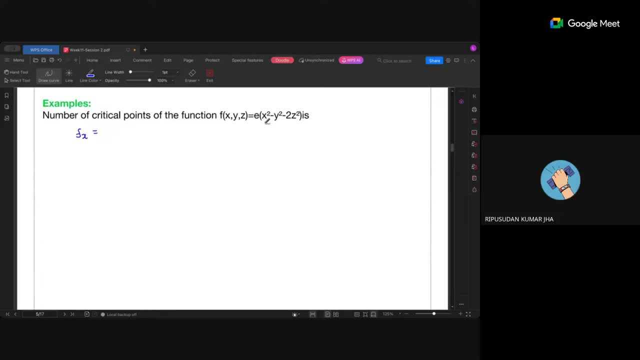 so here i guess it's e power. e to the yes, ma'am, e to the power: x square minus y square minus 2z square into 2x. oh, the question is into 2x, is there? just let me check the question once. no, ma'am, no. 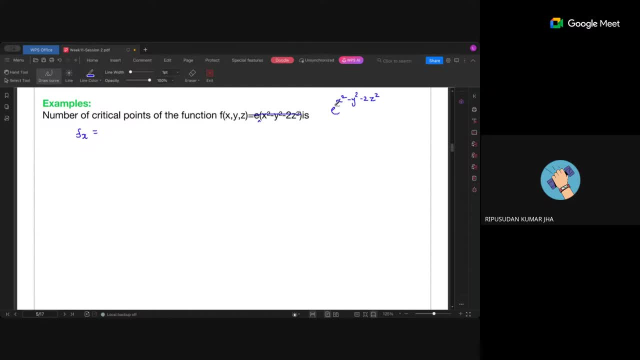 ma'am, partial derivative will be into 2x. oh yeah, telling the partial derivative, all right, let me. let me check the question also once. no, yeah, if there is a mistake here. so it is e power x into x square minus y square minus 2z square. okay, so this is the function. so now what is your fx? 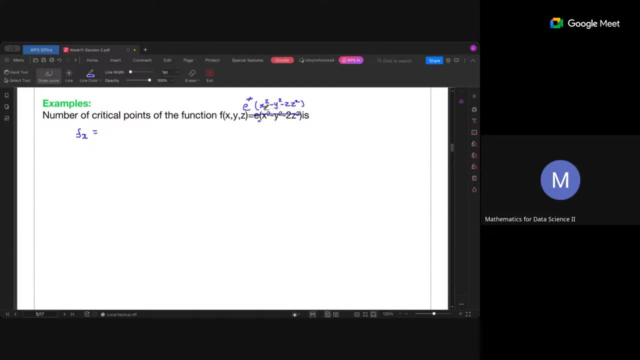 so you have to apply product rule, right? so if you apply product rule, so the derivative of the first term is the same. so you will get e power, x, x square minus y square minus 2z square. now, keeping e power, x as it is and differentiating this term with respect to x, what is that you get? 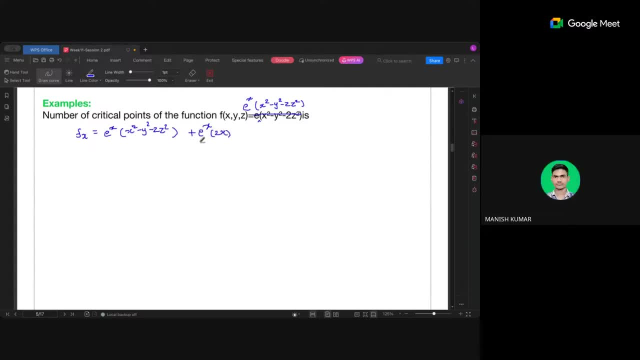 2x. okay, and now fy. the first term is going to be the same. what is the second term? minus 2, y. and what is the third term? the first, the first term is the same, minus 4, z, x, the power forward, x. okay, so the obscure one is to the do. and here is like a pickled coin, which is happening here? 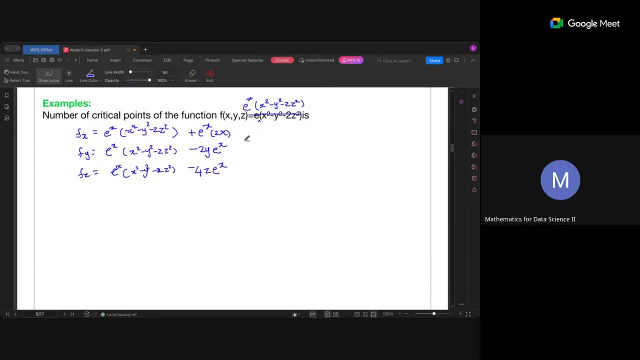 what we can do is this: first of all, let us be thank you so that we canhype out that computer. you know it will end up with something called 2005 f. okay, daniel, here is your question. so夫, these are your fx, fy and fz. so now you are: lf is equal to 0 implies fx, fy and fz are 0. 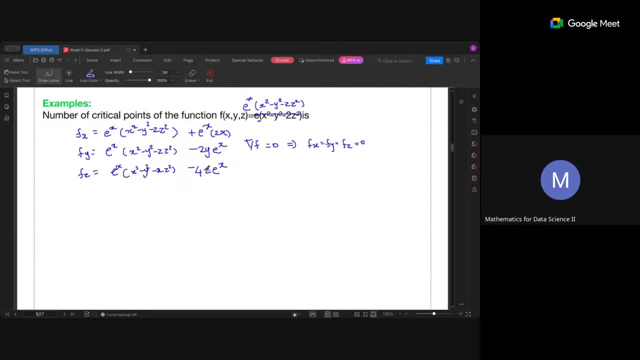 right. so by equating them to 0, what is that you will get? so first you see that you have: fx is equal to 0. so if fx is equal to 0, then you have some complicated terms. now what happened? okay, by the way, here e power x, here i made a mistake. so here e power x. what is the 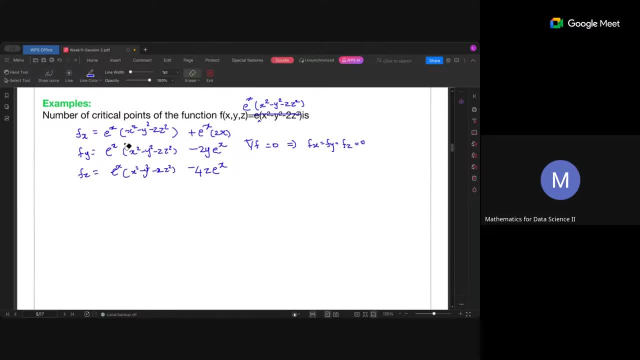 derivative with respect to y. what is the derivative with respect to y for e power x? so e power x. with respect to y, as well as with respect to z, it is 0, right, so here only you have these terms. so fy is equal to 0, implies you what y e power x is equal to 0, which means in fact minus 2, if you. 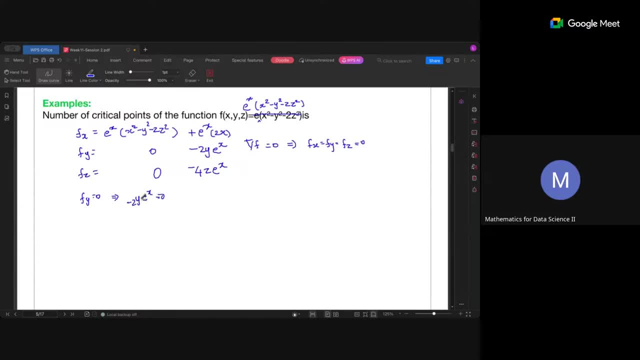 want. so e power x will not be 0 for any value of x, so you will get: y is equal to 0. similarly, what happens if fz is 0, z equal to 0? yeah, you get z is equal to 0. now y is equal to 0 and z is. 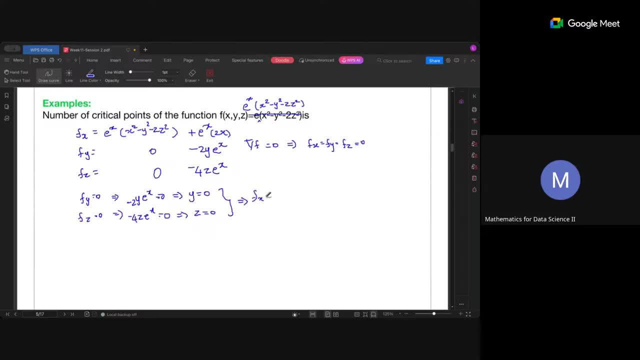 equal to 0. if you apply them, your fx, what happens? x must be 0, so you get e power x into x squared plus 2x. e power x is 0, which means now, if you take e power x commonly, you have x squared plus 2x is equal to 0. 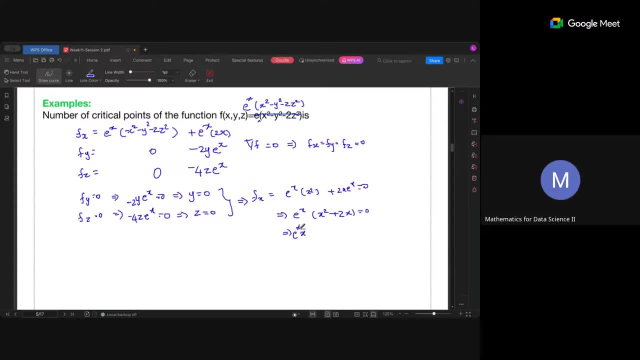 which means x times e power x, x times of x plus 2 is 0. so what are the solutions? right? so these are the values. so you have: y is equal to 0, that is equal to 0, and 2 values for x. so what are the critical points? 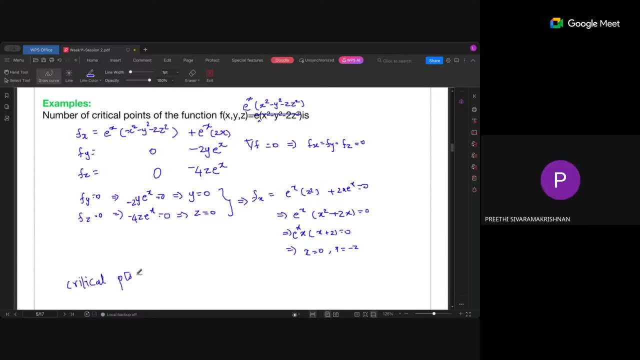 0 0 0 and minus 2 0 0 0 0 and minus 2 0 0. all right, is that clear? yes, ma'am. okay, so these. this is how you find the critical points for a function of three variables. now let us try. 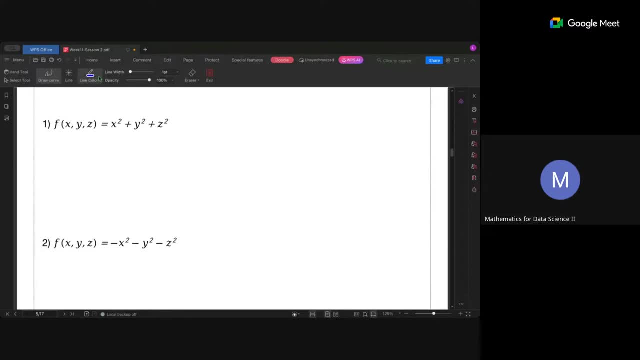 to do the classification of this critical point. so now for all the upcoming problems, we'll find and classify the critical points. okay, fine, so now for this function. first we have to find what are the critical points. now, what is fx, 2x, 2x, fy. 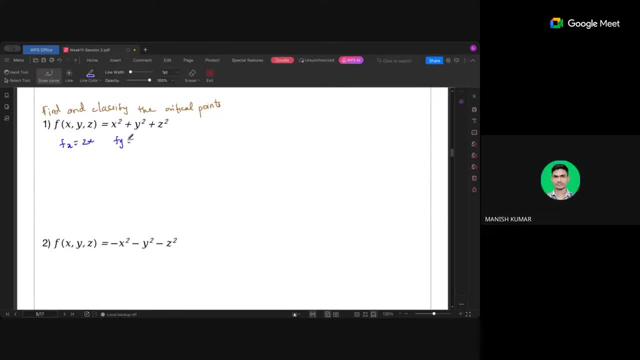 and fz is. so now, del f is equal to 0 will imply 0. what does it imply? all of them are becoming 0, yeah. x is equal to zero, y, fy is xyz. all of them are becoming 0, 0, yeah. so now, if all of them are 0, then what is the only critical point? 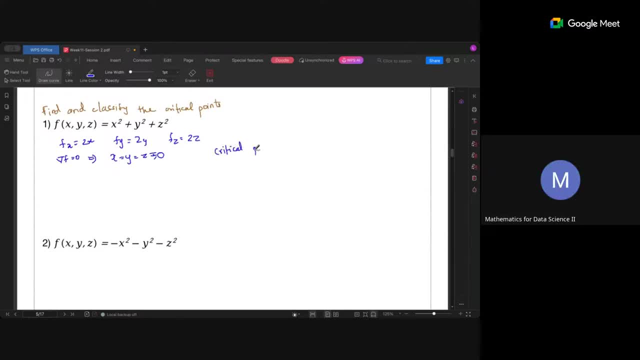 0. yeah, okay, so now we have to find. for hessian matrix you need to find all the second order derivatives. What are the second order derivatives? What is fxx, fxy, fyy, fzz? Now, what about fxy 0, 0? 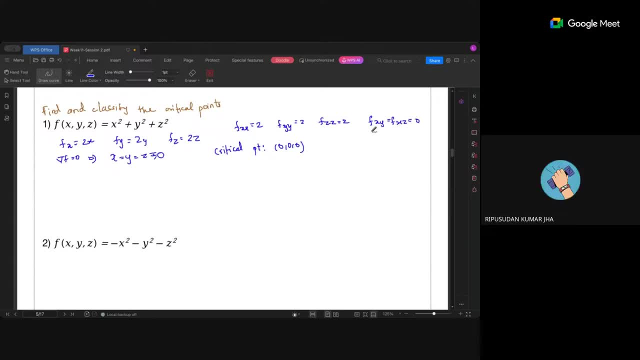 0, 0, fxx and fyz, 0 and fzx, and it is already covered in here, So that's all. So now we can write what is the Hessian matrix here? At the point 0, there is nothing to apply because there are no. 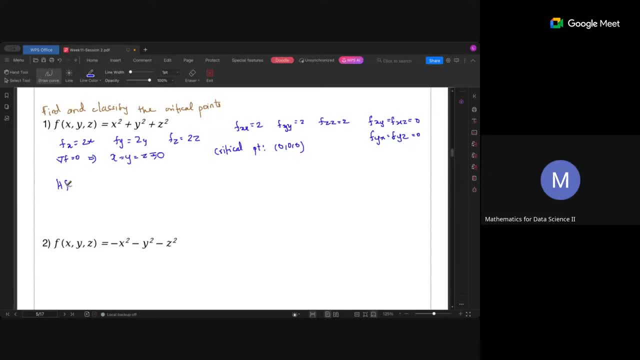 variables involved in the second order, partial derivatives. So straight away we can write: So this is your a tilde. now This is your a tilde. So at a tilde is, can you tell the matrix? 2 0 0 0. 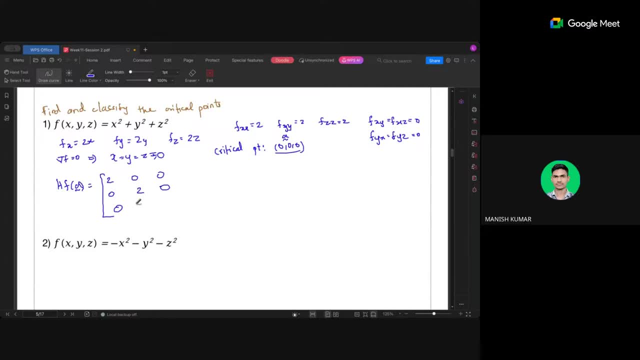 2 2 0 0. Someone is making a lot of disturbance in this class. Please mute yourself, Okay, 002.. Okay, So now what is your step 1? You find the determinant of this matrix. What is the determinant of this matrix? 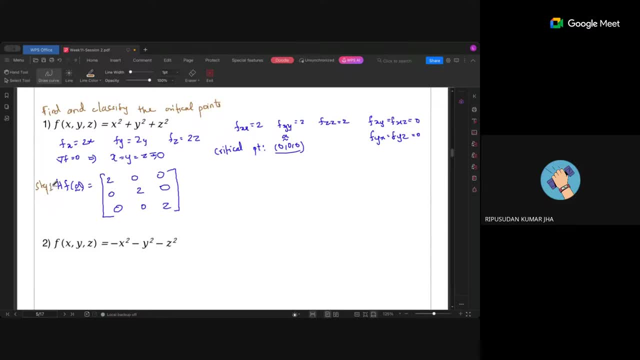 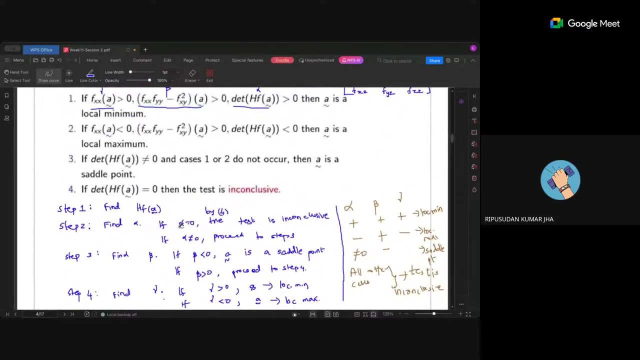 so this is one we have done. and step two, we find the determinant. so determinant of hf of a tilde is eight. so now this is a positive value, positive. so if this is positive then what is that we need to do? we should move to the fxx at a tilde. yeah, so we have a positive in a positive case. 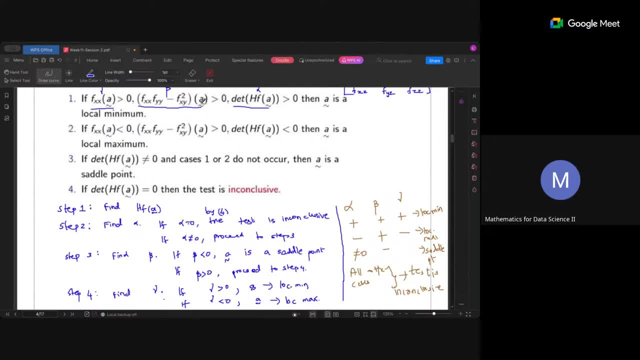 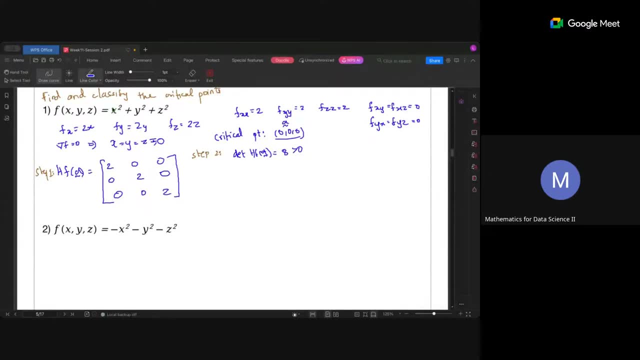 so next we have to see what is fxx fy y minus fxy square. so it means which part we are considering. we are finding we are in fact considering the determinant of this part. so the determinant of this part is nothing but fxx fy y. so 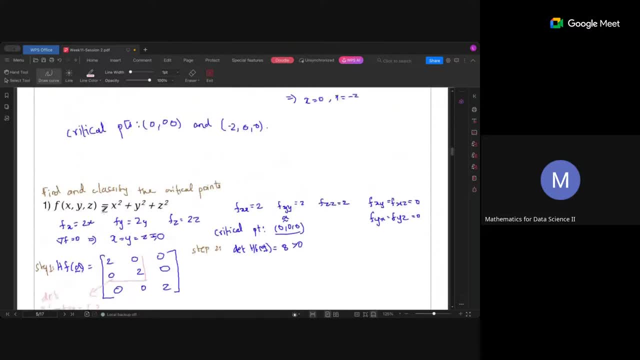 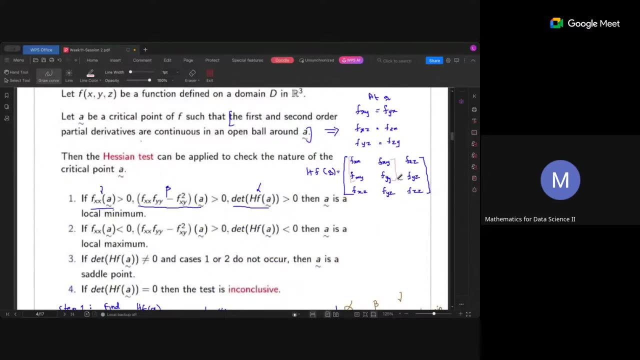 minus fxy square, correct. if you look at this hessian matrix, it will be more clear what is the determinant of this part: f of x y into f of y y minus f of x y square. so which is nothing. but this is your beta, actually correct. 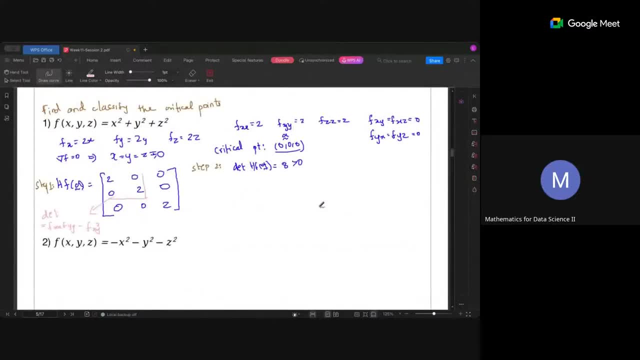 so you have to find the determinant of this part. so what is the determinant of this part? four, four. so you see that now the determinant that is fxx, fy, y minus f square, fxy, square, at a tilde, this is four and positive show. you see, this is positive and 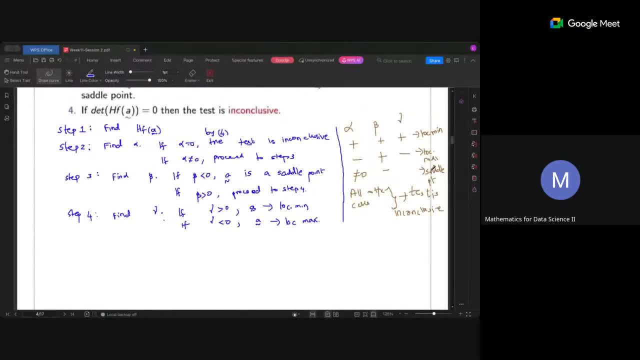 and this is also positive. So you have two positives. So it is not a saddle point definitely, because for saddle point only if it is negative, then you will have a saddle point. So now you have a positive value here. So now, if it is positive, then we are going to look at whether 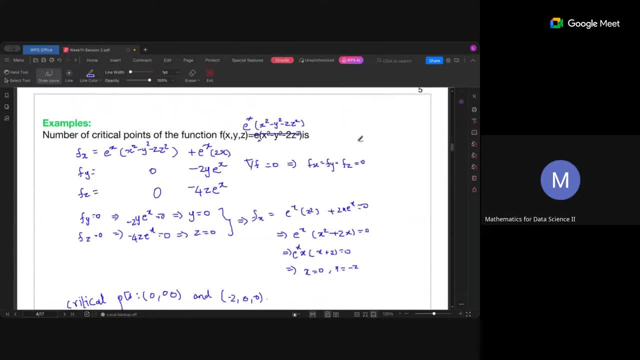 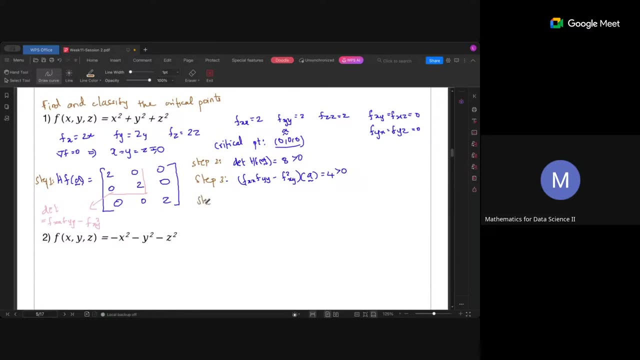 it is plus or minus right, This alpha. So alpha is nothing but the value of fxx at a tilde. Now what is your step 4? You have to find the value of fxx. What is fxx at a tilde? It is 2.. Now 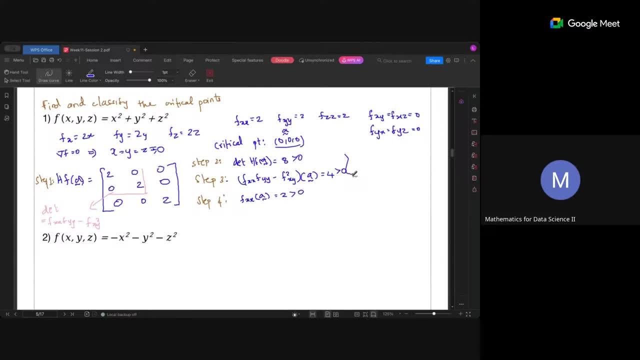 this is also positive. If everything is positive, all these are positive, then what do you know about a tilde Local minimum? Yes, it is a local minimum, Okay, clear, Ma'am. one doubt: Yeah, Ma'am, how can we immediately check that? if the higher? 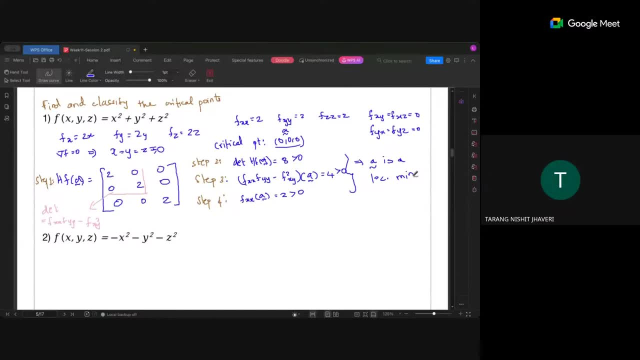 order. sorry, second order or the first order, derivative is continuous. This is a very straightforward case. Here you just have quadratic function, So polynomial function. So this is for other function, See usually in the cases when you have function, smooth function, 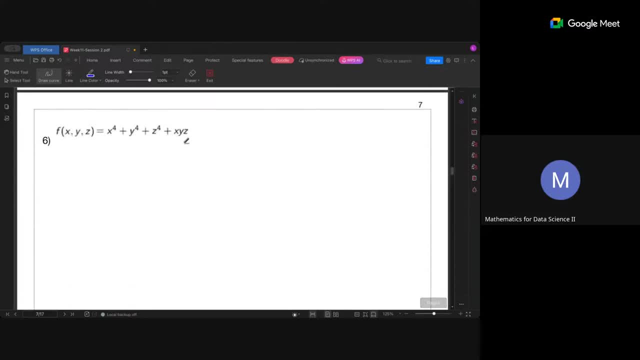 like you have like functions like this, there should not be any problem, while like polynomials like this. But when you have a piecewise function you have to be a little careful. Mainly you have to check the continuity at the points where the piece is occurring right. So, for example, I guess 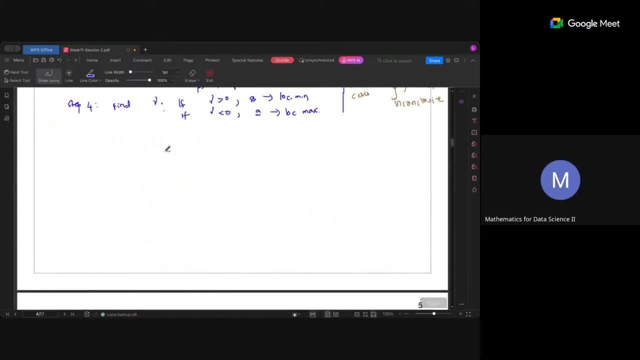 maybe in the lecture itself. there was one problem. If I remember correctly, it was something like this: f of x, y, x comma y is x, y x. I do not remember correctly. It was something like this: by x square plus y square and: 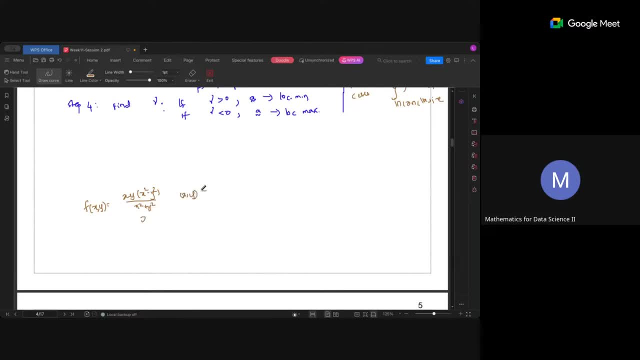 something like this. I am not sure exactly, All of it are variation of it. Sometimes they root in the denominator Yeah, something like this: Okay, So for this it was proved that the mixed partial derivatives was not continuous at the point 0 comma 0. So it is not continuous. 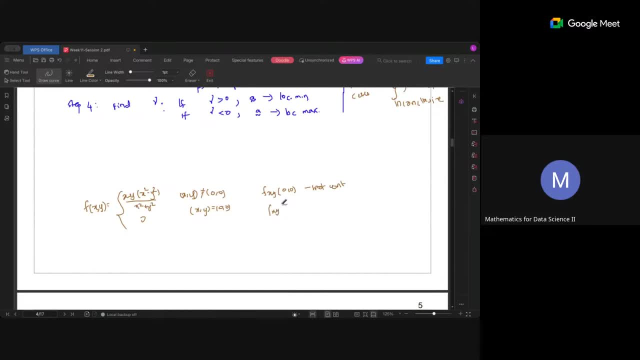 and hence you see that f x- y at 0: 0 is not equal to f y- x at 0: 0.. So it means at this end points you have to check first of all, particularly when you have this kind of piecewise function you have. 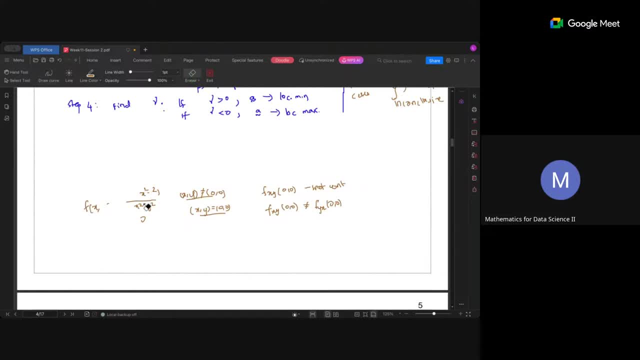 to be careful. Otherwise, usually, whenever you are given some polynomial functions like this, it should not be a problem at all, You do not have to worry anything. Polynomial exponential. So for such things you do not have to worry anything. So for such things you do not have. 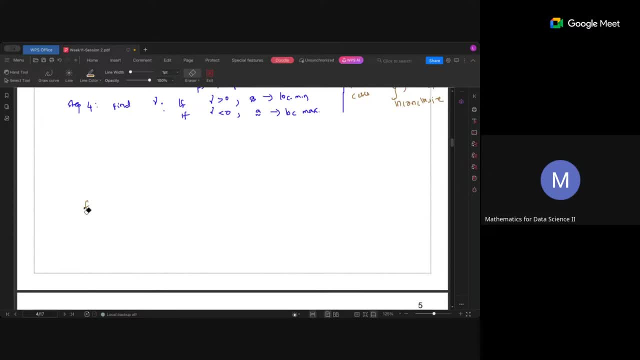 to worry, Okay, Okay. So let us do similar process for this function as well. Now, what is your f? Critical point is 0.. Sorry, Critical point is 0.. Yeah, yeah, Critical point is 0.. 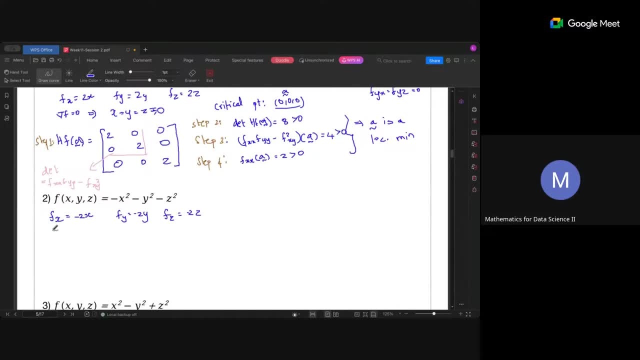 Critical point is only 0. So now, del f equal to 0 implies x equal to y, is equal to z equal to 0. It means the only critical point we are having is 0, 0, 0. Right, Okay, So now. 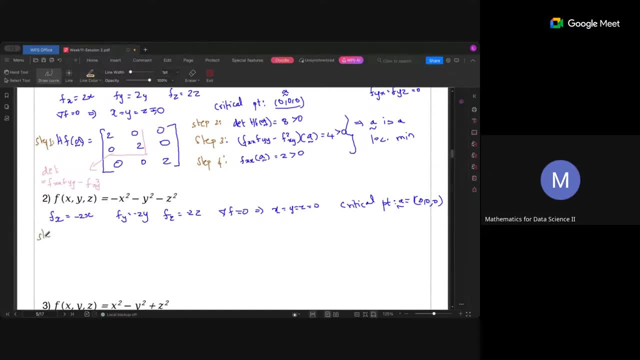 what is your step 1?? As usual, find the Hessian matrix. So what is your Hessian matrix here? So you need what is f x x? What is f x x here Minus 2.. What is f y y? 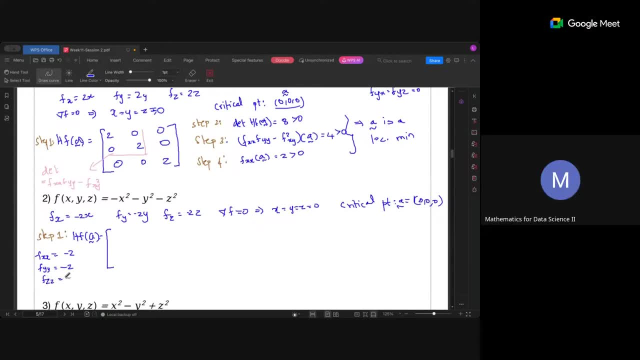 Minus 2.. And f z z is also Minus 2.. And what is? f x y Minus 2.. And f y z? Sorry, f x z Minus 2.. They are 0.. Similarly, f y x, y z and f um f. what else is there? 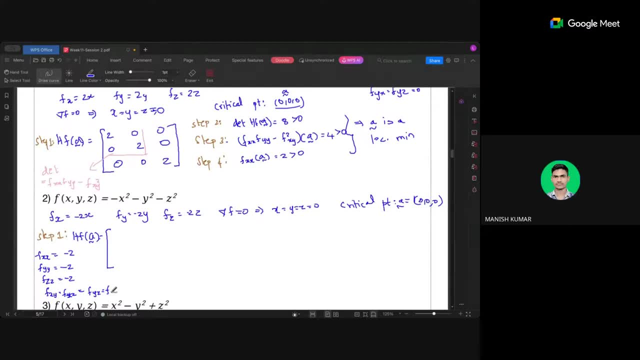 Z y Minus 2.. y, z and z y, they are same. I guess that is it. So all these are again 0. Right? So it means what is this Hessian matrix now? Diagonals are all minus 2 and the. 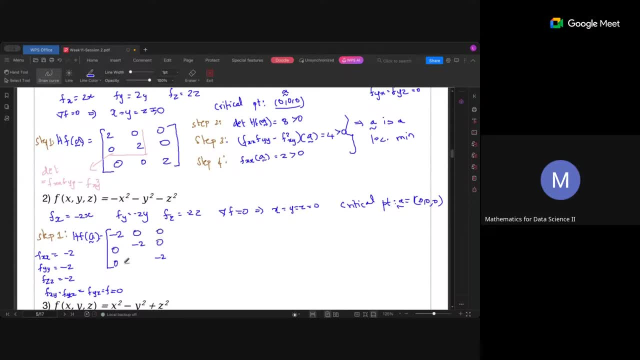 remaining entries are 0.. Right, Okay, So now you find what is the determinant of this matrix. So what is the determinant of this matrix Minus 8.. Yeah, So now this is less than 0. So you will not have case. 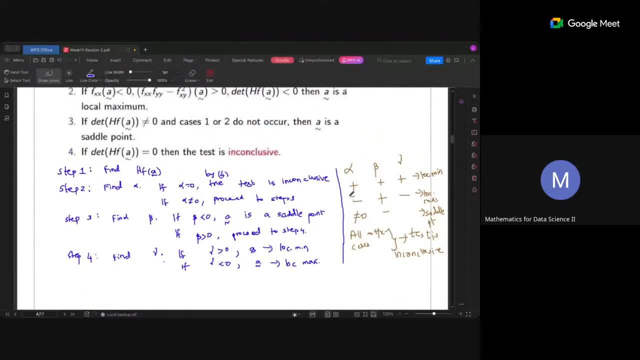 1. Case 1 is not possible, Right? So you have case 1, case 2, case 3 and all others are case 4.. Okay, So case 1 is not possible. Now let's look. 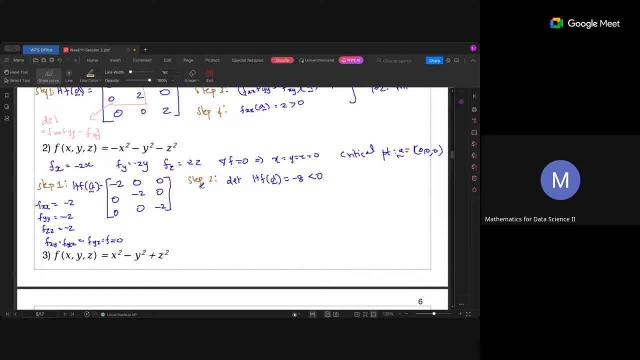 at step 2.. No, sorry, Step 3.. So what is your step 3?? You have to find the determinant of which part, This part. So now, what is the determinant of that part Which is fxx, fy, y, minus? 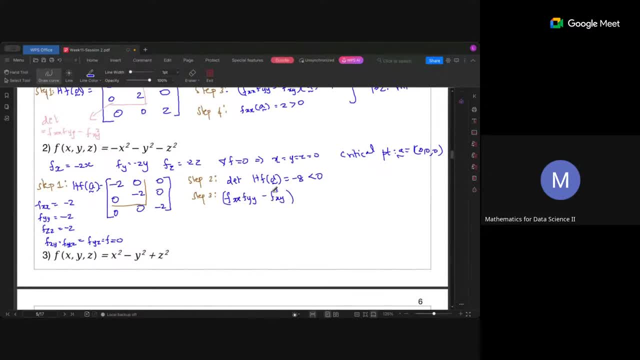 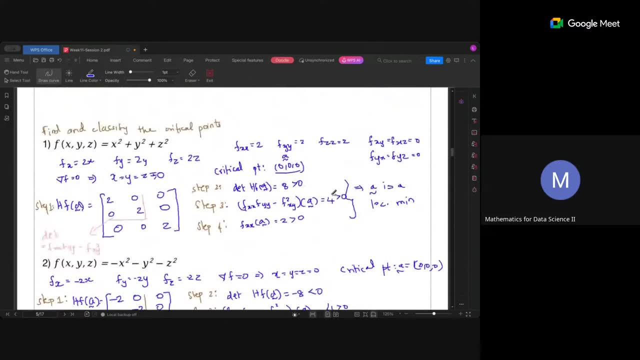 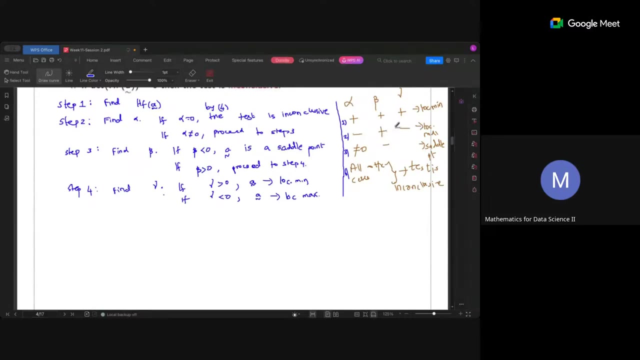 fxy square at a tilde Which is 4.. Now this is positive. So you have: alpha is negative and beta is positive. Alpha is negative, beta is positive. So we have to now check what is the last quantity. So let us. 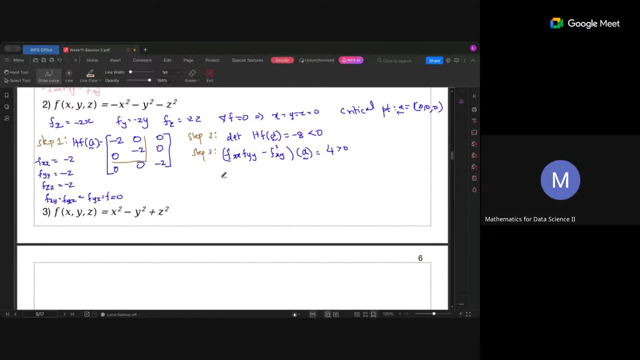 look at step 4.. So step 4. You have. you should check what is fxx at a tilde. What is fxx at a tilde? Minus 2. Minus 2, which is again less than 0. So now, this is which case. 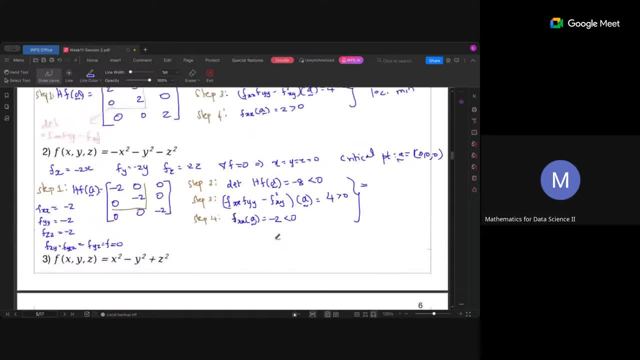 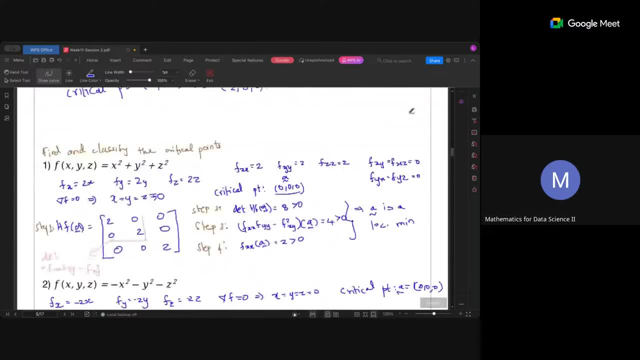 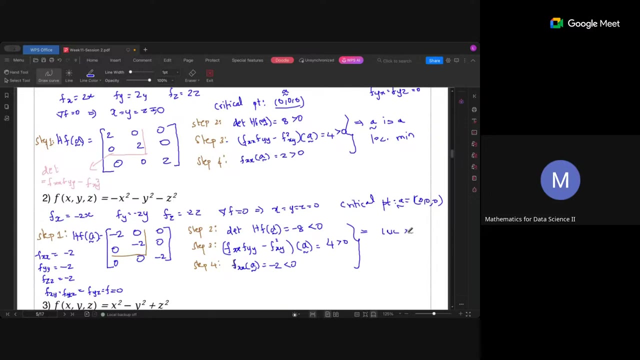 Negative, positive, negative. So which case? Negative, positive, negative. So which case? It is case 2, right, Yes, ma, So this is case 2.. So case 2.. You see, You have a tilde is a local. When it comes to the corner it does not work. 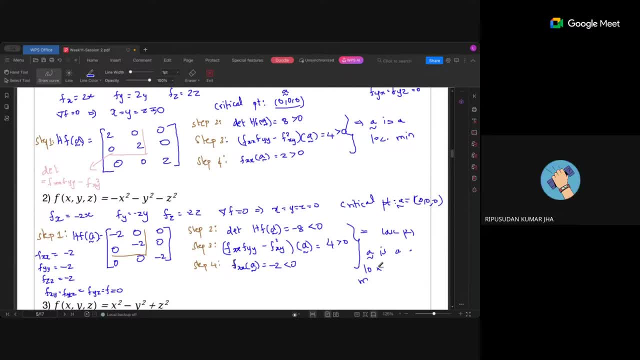 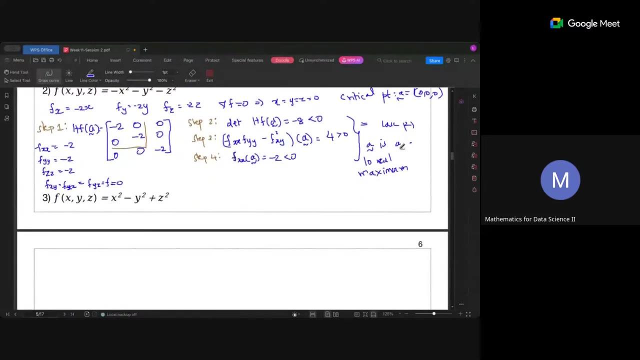 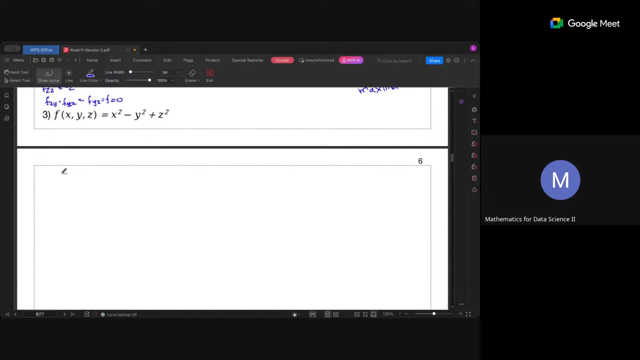 local maximum. right, okay, so we have seen one example for local minimum and local maximum. now let's look at this problem and do the same process again, finding and classifying the critical points. now, what is fx, 2x, fy minus 2y, fz, 2z? so it is: 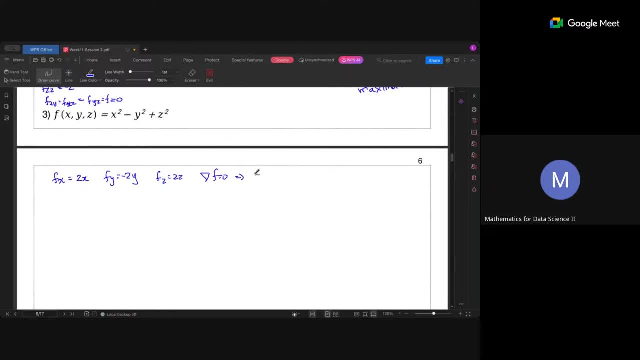 obvious that what is the only critical point again? yeah, so the only critical point you are having is a tilde is equal to 0, 0, 0, right, and now you have to find the hessian matrix. so for finding the hessian matrix, so let's write step 1, so you have HF at a tilde. shall we write the matrix? 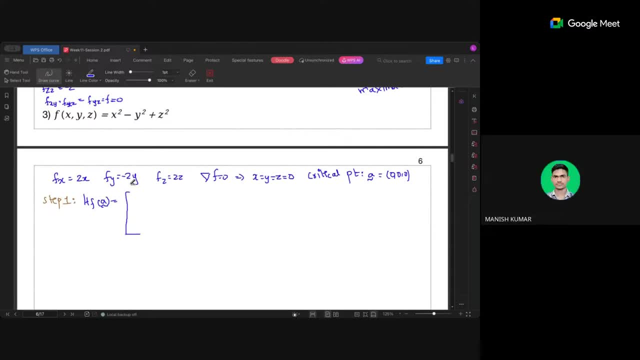 straight away, now, straight away, now, straight away now. what is fxx? what is fxx? what is fxx? fxy 0, fx z 0. what is f? y x 0 and f y y and f y z 0? so, since it is a, f x y 0, f x z 0 and f y y and f y z 0. so since it is a f x y 0, f x z 0 and f y y and f y z 0, so since it is a symmetric matrix, you know. 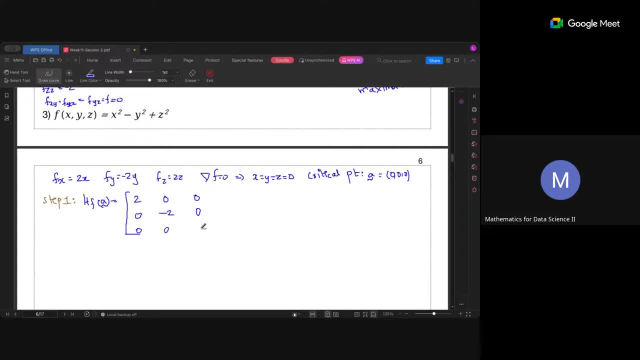 symmetric matrix. you know, symmetric matrix, you know, these two entries must be 0. and what should be fzz? these two entries must be 0. and what should be fzz? these two entries must be 0. and what should be fzz. okay now, okay now. 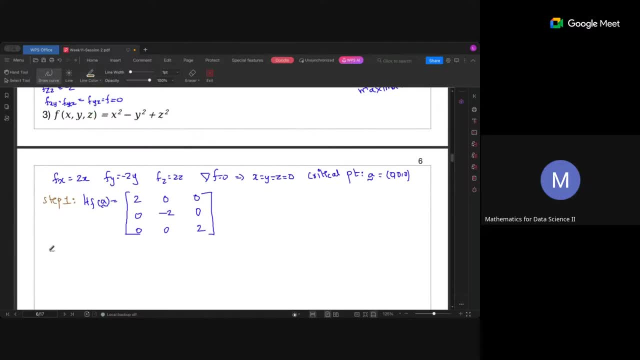 the next step is to find the determinant. Now, what is the determinant of this Hessian matrix Minus 8. It's minus 8.. So case 1 is not going to be possible. So we have to see whether it is case. 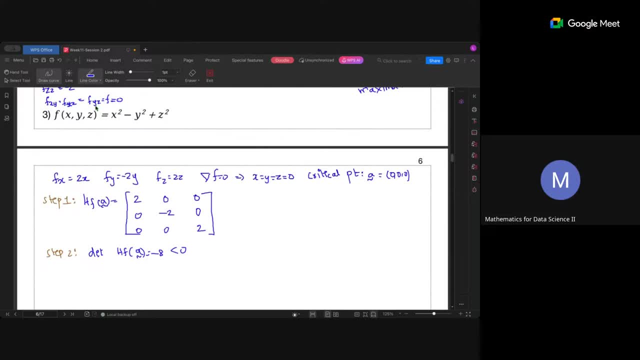 2, case 3 or the other one. So let's see step 3.. So in step 3, you have to find the determinant of this part. So now, what is the determinant of this part, Which is nothing but f, xx, f, y, y? 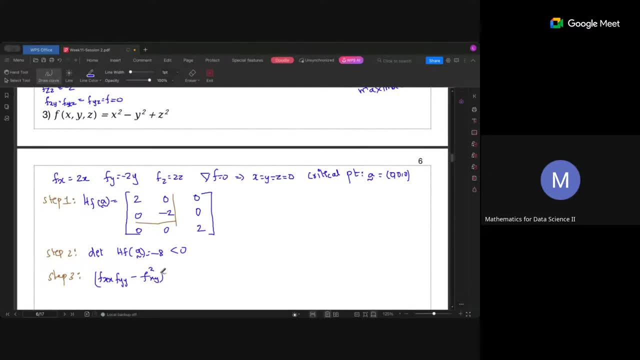 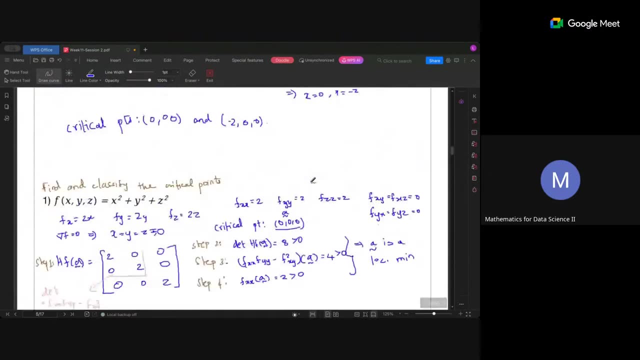 minus f, xy, whole square at a till. What is that? It is minus 4.. So two negatives, Which We don't have, two negatives in case 1 or case 2, right, So in case 1, either 2 positive or case 2, 1 negative, 1 positive. 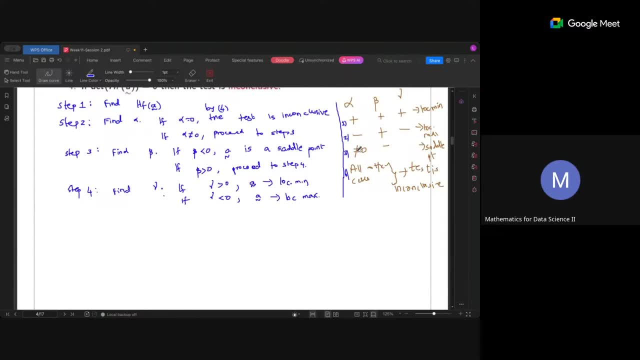 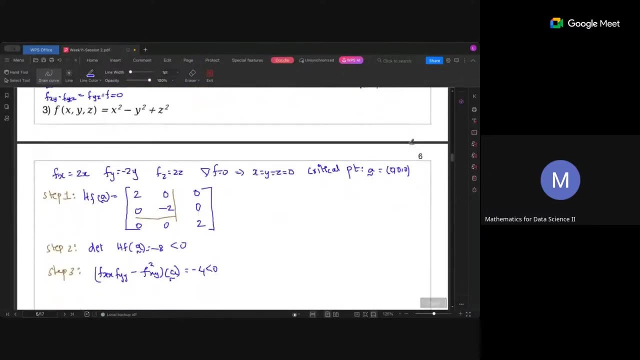 So these two cases are not there. So which case does it go to? So you have a non-zero determinant and you have this also negative. So you have to now look at what is the gamma value. So you have to see whether you have the third case. 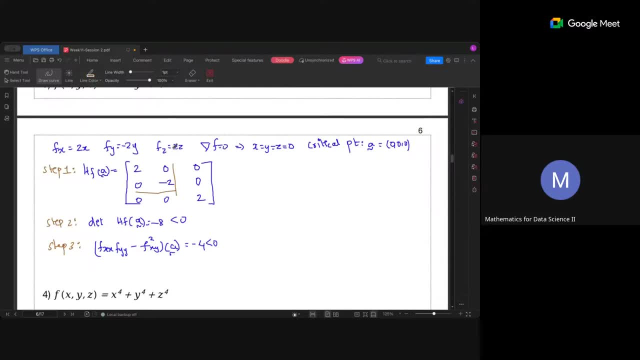 So now, what is your step 4?? What is it you need to calculate in step 4?? Step 4, you find what is fxx at a tilde. So fxx at a tilde is 2.. Now your 2 means this is a positive value. 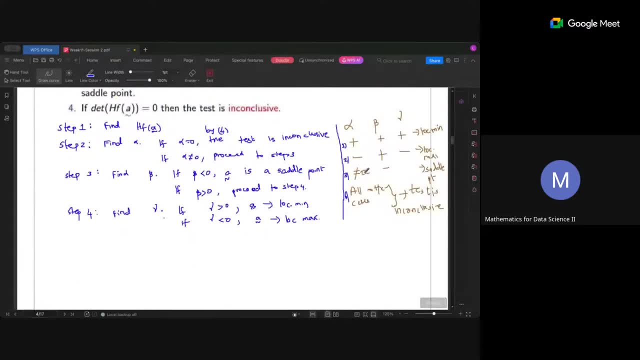 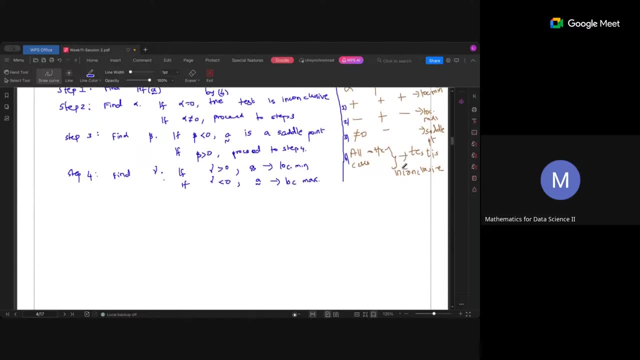 So now you see that here, if it is non-zero negative here, whatever is the value, it is going to be a saddle point. So you don't even have to find this straight away. You can in fact write that this is a saddle point. 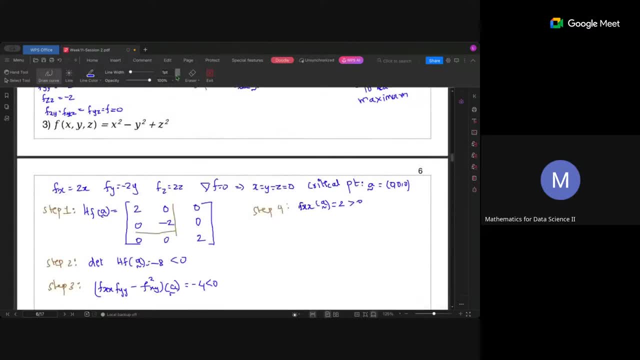 Sorry, You don't even have to do this step 4. It is not necessary. Straight away we can write that this is not necessary, So I am removing it. So straight away we can conclude that. So from this itself we can conclude that a tilde is a. 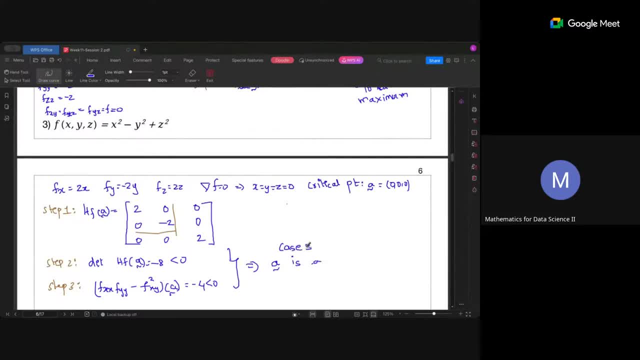 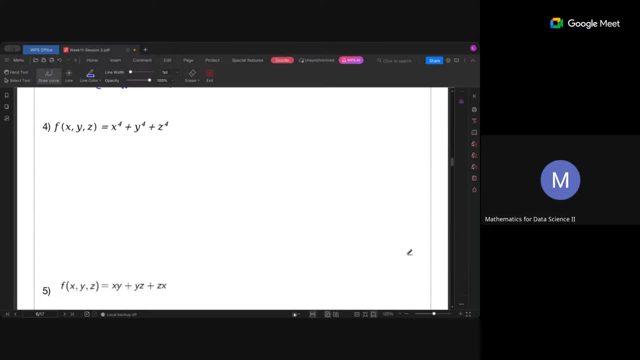 So now let us look at another problem. So now for this problem. what is your del f? 4x cube, 4y cube. So if del f is equal to 0, you get. So what is the only critical point? 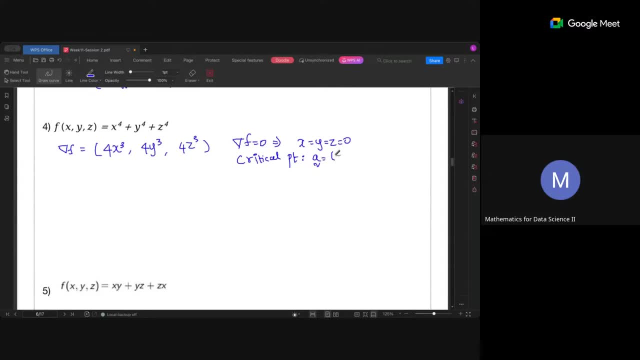 0, 0, 0.. Yeah, Okay, So now you have Step 1, the construction of Hessian matrix. So you have hf at a tilde. So what is fxx? What is fxy? 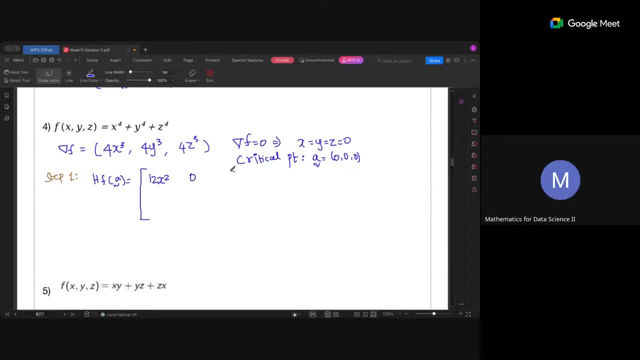 0.. And fxz 0.. 0.. And f. So this is symmetric matrix, So this value is 0.. So what is fyy? 2 and y Square. 2 and y square. 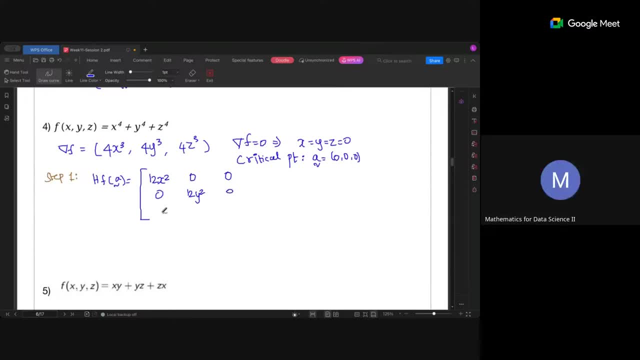 And here what is? fyz 0.. 0.. And symmetry 0.. So here these are 0.. And here you have 2 and y square 2 and y square, Right, Okay. So the next step? you have to find the determinant. 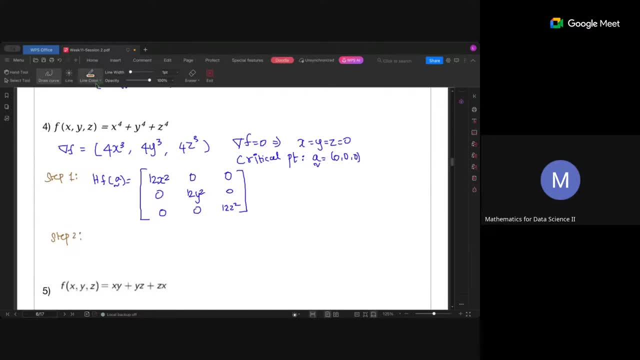 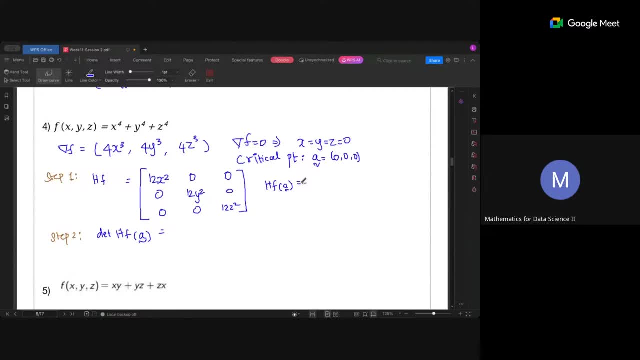 What is uta? Yes, I am curious. Yeah, Yes, We have 8.. We have all right. Yes, Yes, Yes, 1, 7, 28.. Yeah, Hold on. So this is just hf. Now, what is hf of a tilde? 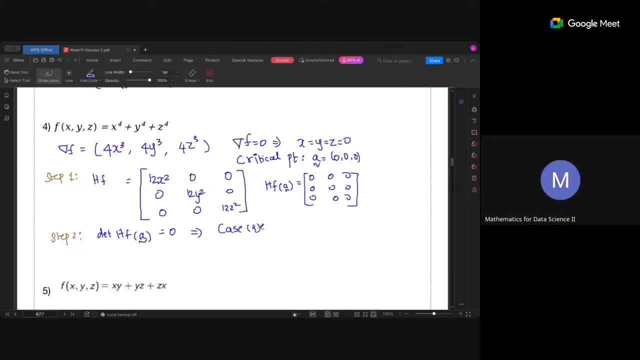 0, matrix inconclusive. yeah, the test is inconclusive. all right, okay. so we have seen all possible cases, so let's see what happens now. so now, what is your gradient function? what is your gradient function? what is fx here? yeah, y plus z. and what is fy z plus z, z plus x. and then what about f, z x plus x plus y? 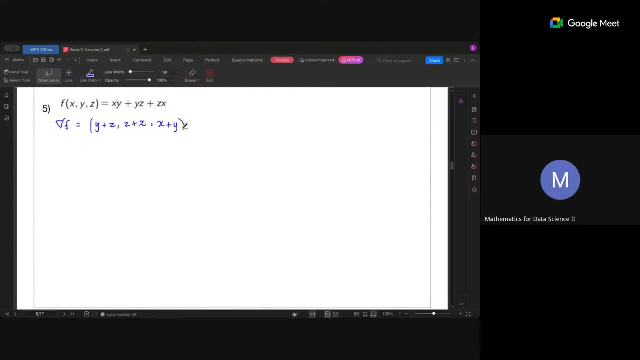 okay, fine, so now del f is equal to zero will imply y is equal to minus x and x is equal to minus y, right? so now you see that you have minus y is equal to x and x is equal to minus z. so from z equal to y. 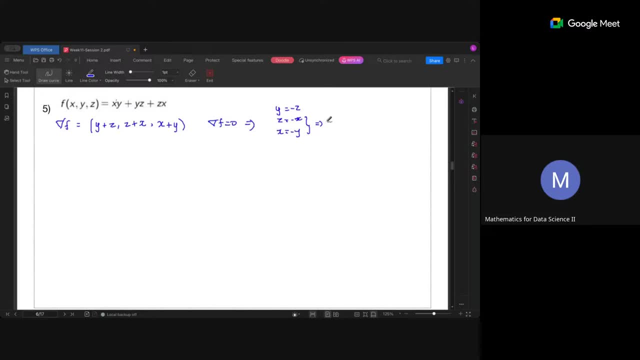 yeah, from this two you can see that y is equal to z. Did I write it correctly? Let me write it properly, maybe step by step. Okay, So you have already: y is equal to z, Now y is equal to minus z. So from this you have y is equal. 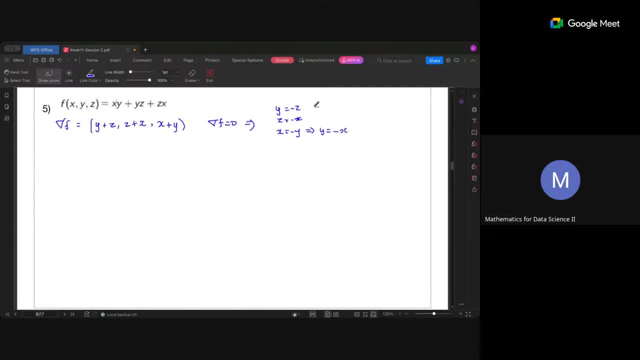 to minus x. So maybe we call this 1, 2 and 3.. So from 1 and 3, what do you get? You get: x is equal to z, Correct, Y is equal to x, right, And equation 2 is given: z equal to. 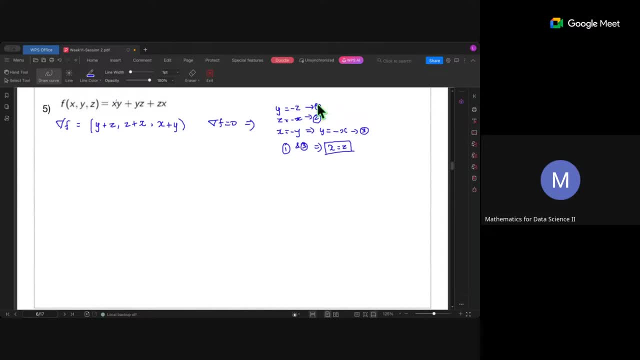 minus x. Yeah, you get all sort of combinations but you can just randomly choose any 2.. So if I am picking 1 and 3, I am ending up with x is equal. see, both the left hand sides are y, so the right hand sides are equal, so x is equal to z. So if you are picking 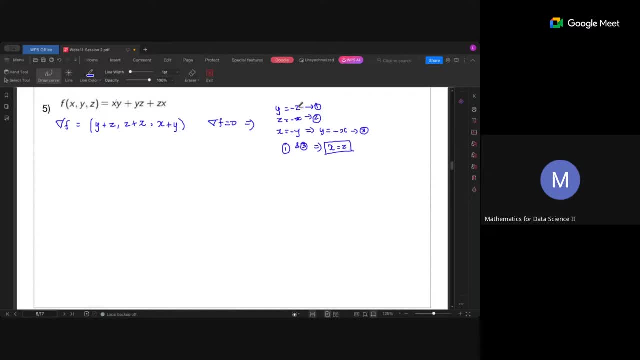 1 and 2, then you will get that z is equal to minus y and z is equal to minus x. so x is equal to y. So, anyway, you are going to get everything. See now what is happening: z is equal to minus x and x is equal to minus z. So now what is happening? Is there any? 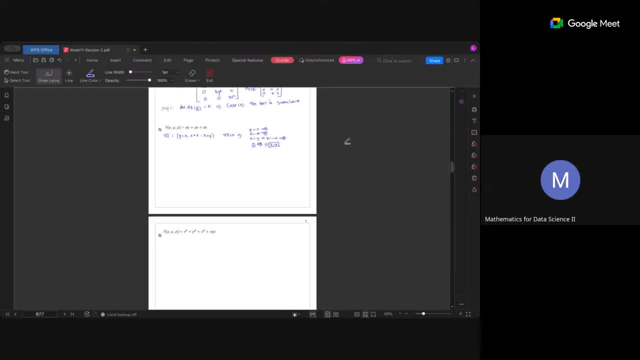 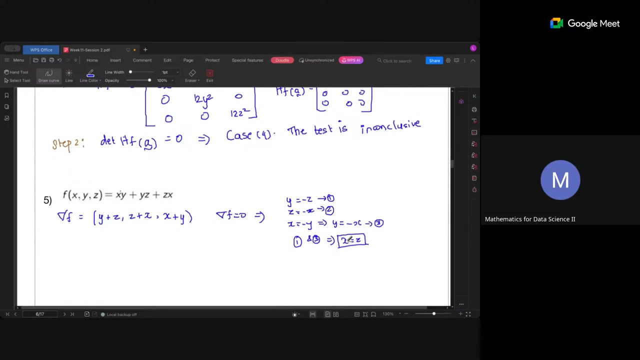 clash going on, Right. So now, what is happening? Is there any clash going on? when does this happen? When does this happen? What happened? I zoomed in, So now let's call this 4.. So now, from 2 and 4, what do you get? You get: x is equal to z is equal to 0. So 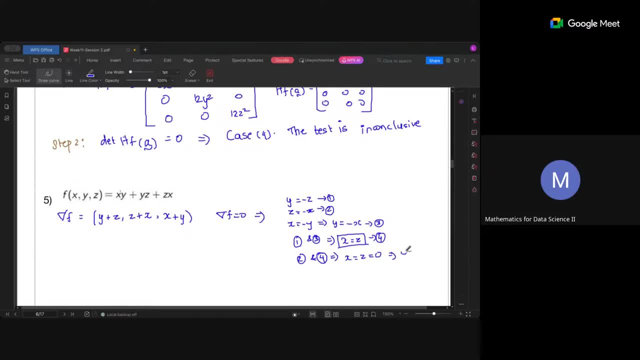 now x is 0, that is 0. So this should imply y is also 0. So now again, you are going to get the only critical point as 0, 0, 0.. Okay, Fine, So now we are going to find what is. 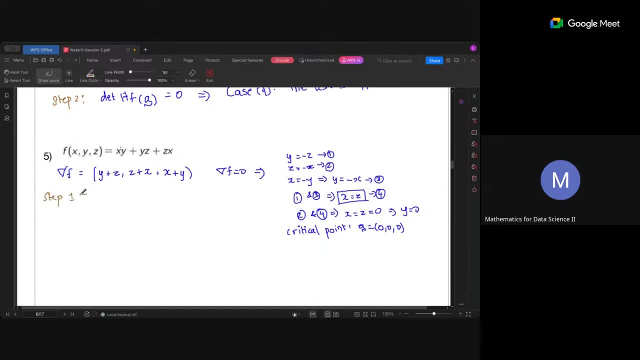 your Hessian matrix. So your Hessian matrix is: so: add a tilde. what is your matrix? 0, 1, 1.. Okay, So what is f x x? What is f x x, 0.. Similarly, what is f y, y, 0. 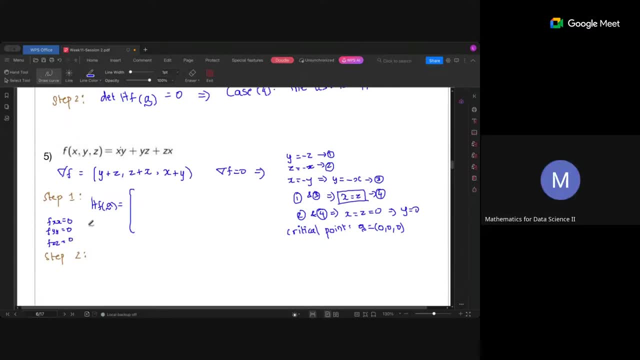 f z z 0.. What is f x y, 1.. And what is f y z 1.. And what is f z x 1.. So all of this are 1.. So it means all the diagonal entries are 0 and all diagonal entries are 1.. So this: 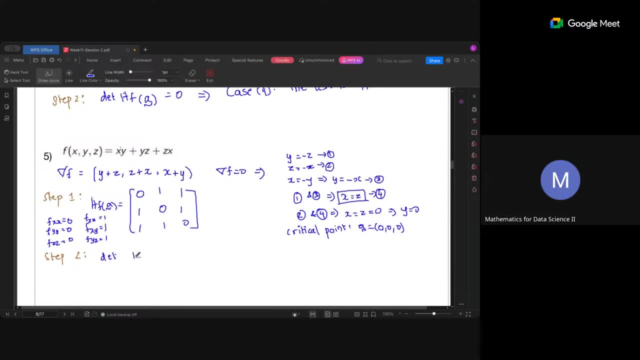 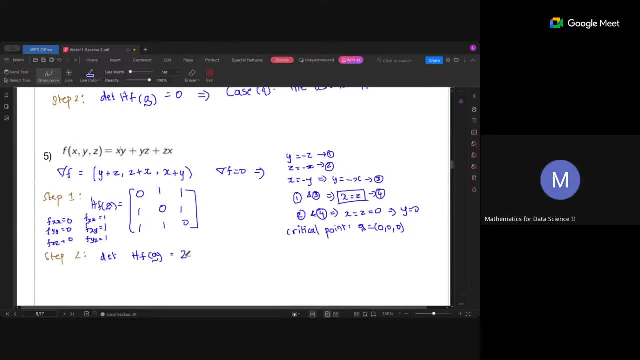 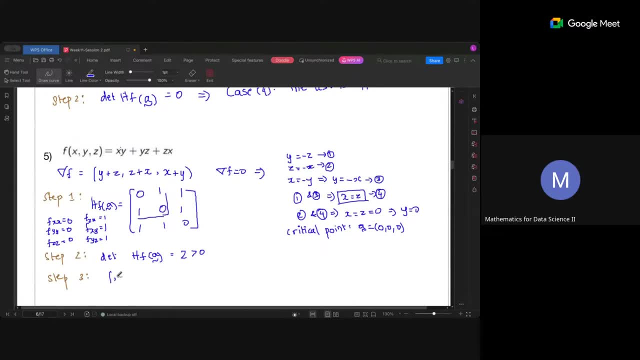 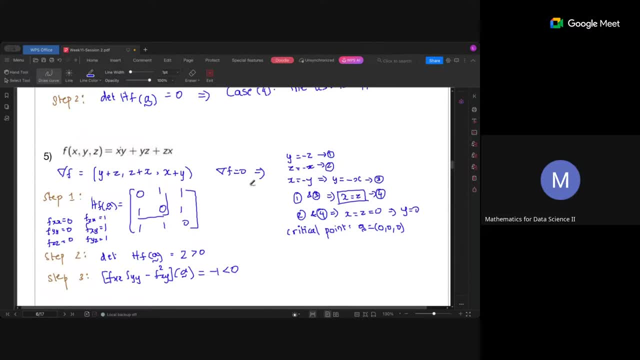 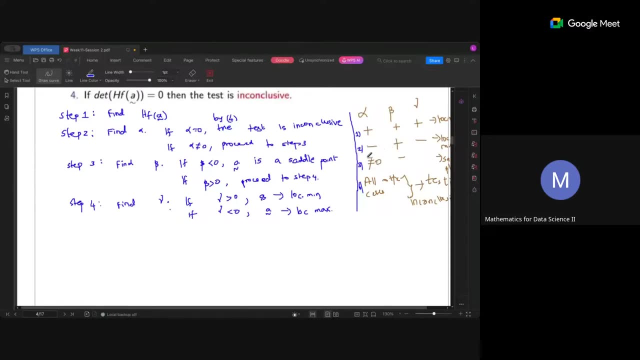 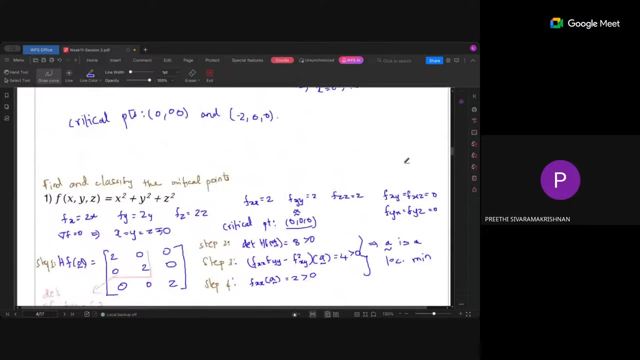 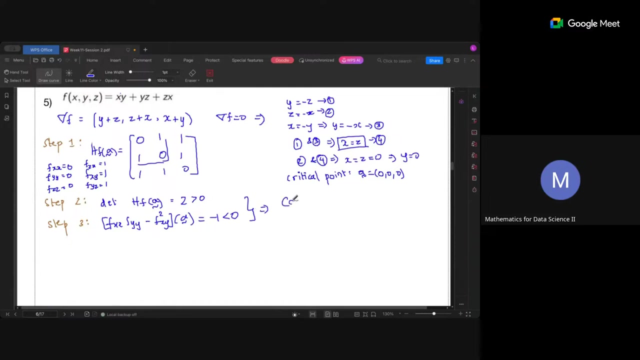 negative, Positive and then negative. Does this scenario happen in case 1 or 2?? No, right. So it means: which case does it go to? if you have some value or non-zero value and a negative case here, then it is case 3, right? Yes, ma'am. So now from this you know that we are in case 3.. 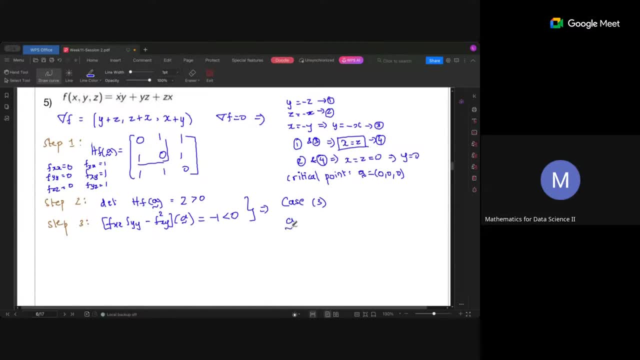 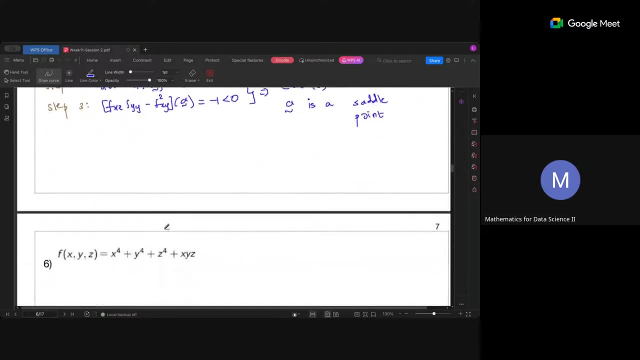 It means a tilde is a saddle point. All right, Okay, So let us do one more problem of this type. So now, what is your gradient function for this? 4x cube plus yz, 4y cube plus xz, 4z cube plus xy. 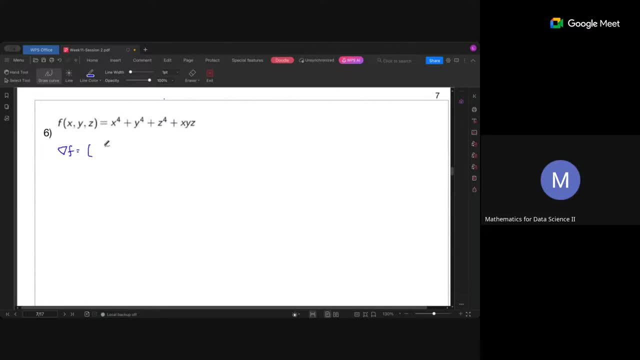 Okay, This one maybe is a little lengthy. So 4x cube plus yz, 4y cube Plus xz. 4z cube plus xy. All right Now your del f is equal to 0, implies 4x cube plus yz. 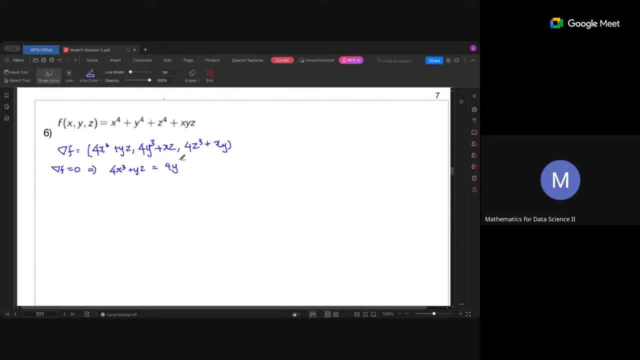 equal to 4y cube plus xz equal to 4z cube plus xy equal to 0, right, Okay, Now, from all these things together, what you get? You get 4x cube equal to 4y cube equal to 4z cube, equal to. we are multiplying a 4 here, So we are multiplying, if you are. 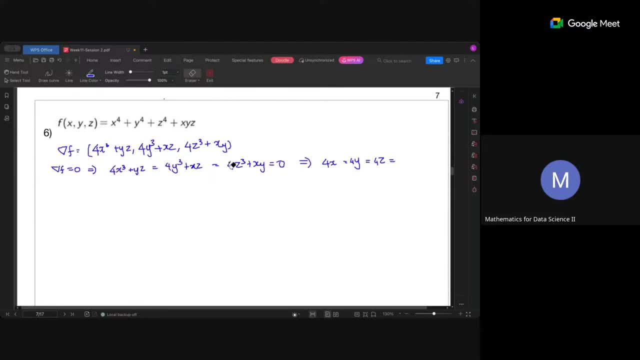 multiplying. let us say x to this term, y to this term and z to this term. Then what is that? you are going to get? 4x cube, 4x power 4, 4y power 4 and 4z power 4.. What are they equal to? Can you tell me? 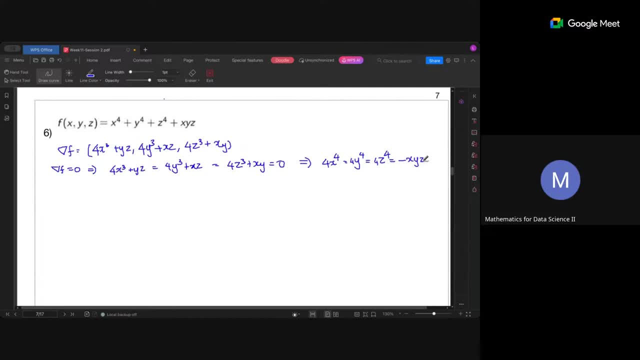 Minus x y z. Yeah, Minus x y z. Okay, So now x power 4 equal to y, power 4 equal to z. power 4 will imply: This will imply x is equal to plus or minus y. So this is what we get from here. And then now, if x fx is equal to 0, specifically we: 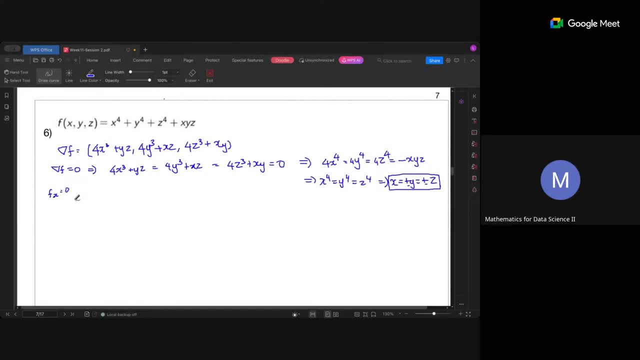 are considering you have 4x cube, And then what is yz? now, y into z is in terms of x, Okay, Okay, So there are two possibilities, right? What are they? Tell me, See, if x is equal to y, plus or minus y and plus or minus z. 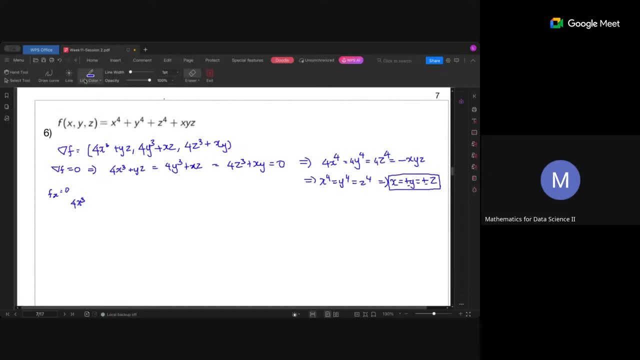 So same sign for y and z. So case 1, you have to consider So y and z having same sign. If y and z are having same sign, then what is y and z In terms of x? Yeah, 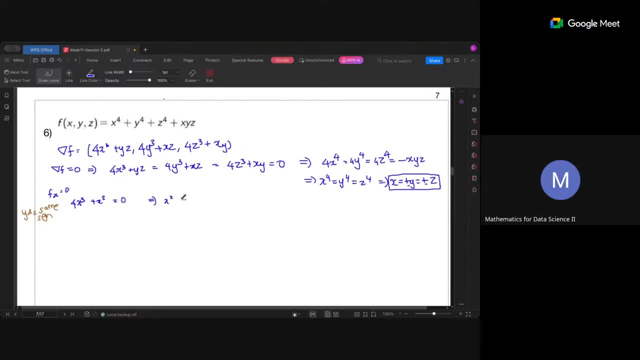 So now you get x square into 4x plus 1 equal to 0.. So what are the values of x? you are getting x equal to 0, or x is equal to Minus, 1 equals to 4.. 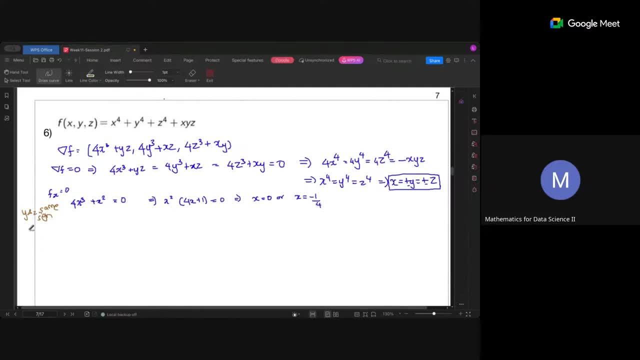 Okay, Now suppose you are having- You are having different signs for y and z, Then what else that you will get? 4x cube here, in case of y is a minus x square, right, Okay, So now what are the values for x? 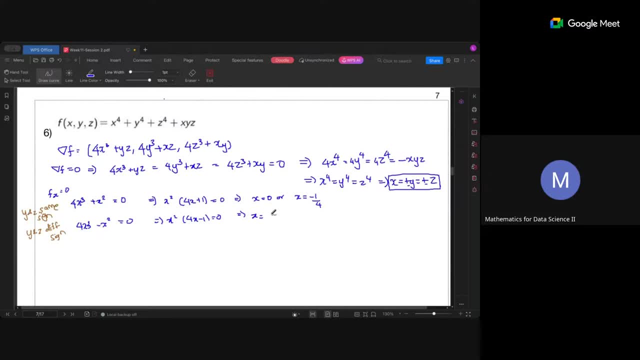 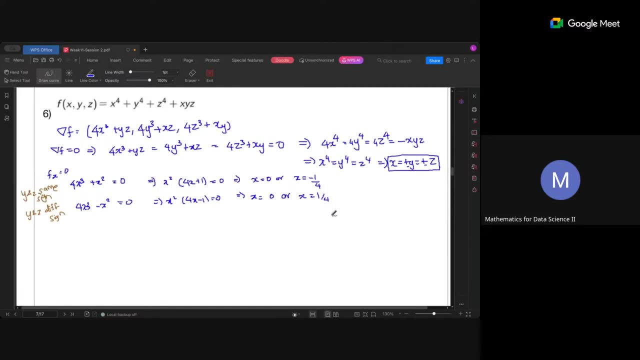 x is equal to 0.. Or x is equal to 1 by 4, right Now, similarly, you have to do this for fy is equal to 0.. Now, for fy is equal to 0, you have 4y cube plus xz is equal to 0. 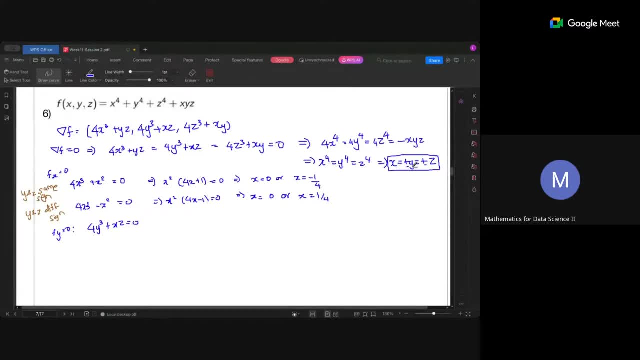 Now again here. if you take Now, you have xz, right. Yeah, So here also you are going to get different values for y. Y is plus or minus 1 by 4 and z also you are going to get plus or minus 1 by 6, right. 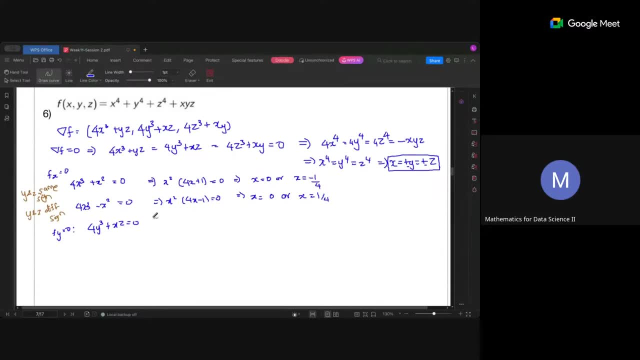 So, depending on the signs of so similar to this case, you are going to get either y is equal to 0, y equal to minus 1 by 4, or y is equal to plus 1 by 4, correct. 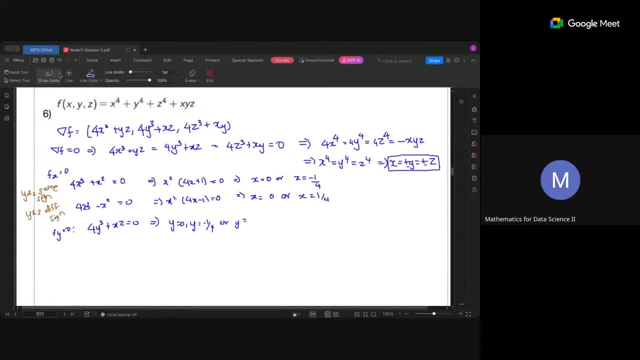 These are the scenarios you are going to end up with. Is that fine? Yeah, Yes, ma'am, Okay, Okay. Now, if you take, fz is equal to 0. again, again, the same scenario is going to happen. So here also, you are going to end up with these possibilities. 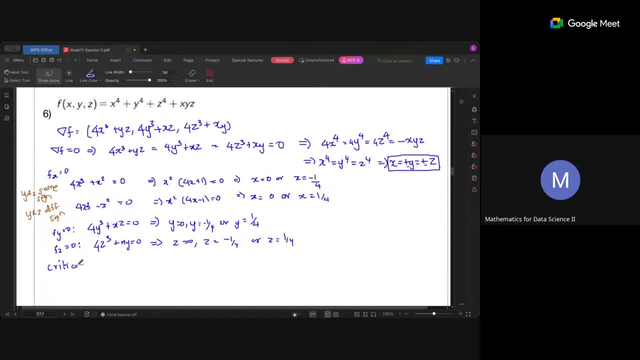 So now, from these values, can you tell me what are the critical points? How many critical points? What is the first one of the obvious critical point? 0. 0. 0? 0. 0. 0. Yeah, 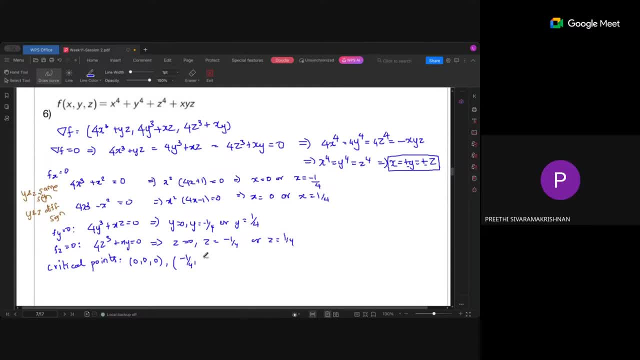 And then Minus minus 4, 1 by 4,, 1 by 4.. Okay, so you can put minus 1 by 4, 1 by 4,, 1 by 4.. And then 1 by 4, minus 1 by 4, 1 by 4.. 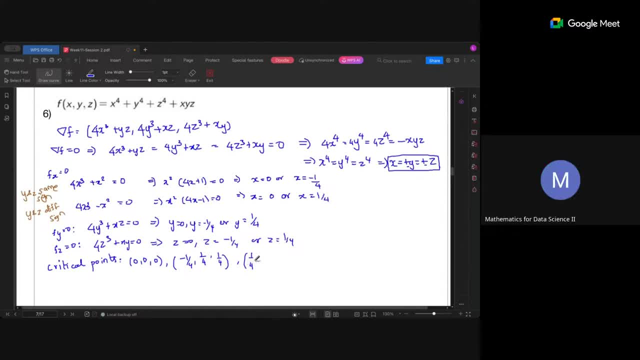 1 by 4.. Minus 1 by 4,, 1 by 4.. And then minus 1 by 4, 1 by 4, ok. and then you have 1 by 4, 1 by 4, minus 1 by 4, ok. what? 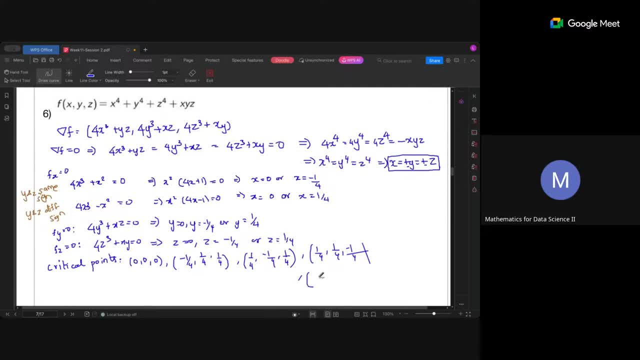 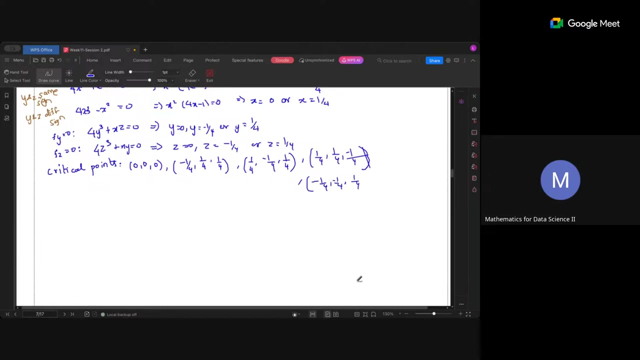 happened, and then you have minus 1 by 4. minus 1 by 4. yeah, so you have these five critical points here, right? ok, so now, for each of this critical point, we are going to verify whether you you are going to have a local maximum, minimum or saddle point, or the test is inconclusive, like this: 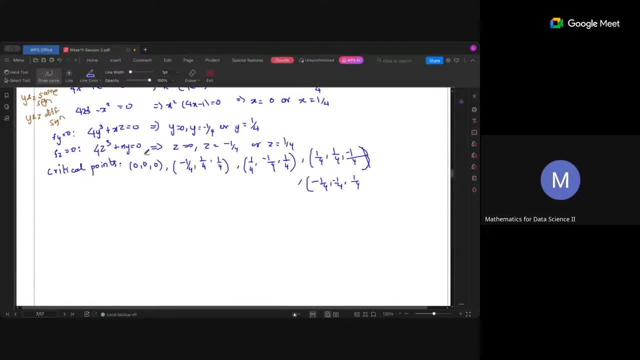 you have to check for each of this critical point, ok, so maybe we call this a 1, a 2, a 3, a 4 and a 4. ok, so now let us do it for a 1. so first let us write the general step, the step. 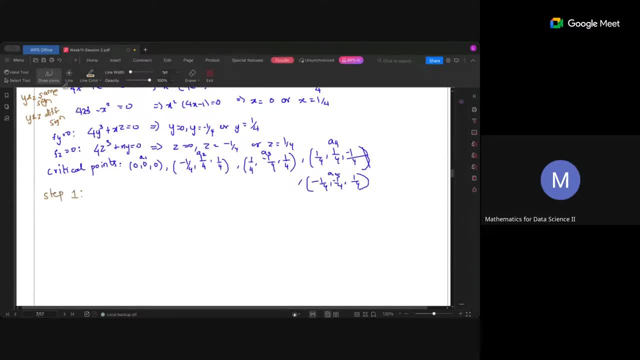 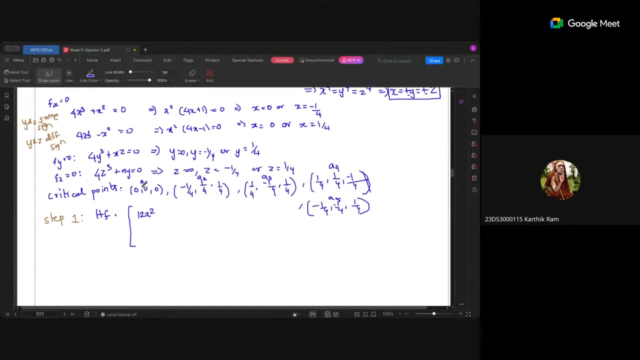 one is common for all the metrics. let us simply write what is HF. it's not right. HF of a tail, what is HF? yeah, so let's write what is HF of a tail? what is HF? so sorry, you cannot. you are saying X is equal to, Y is equal to. you can equate it. 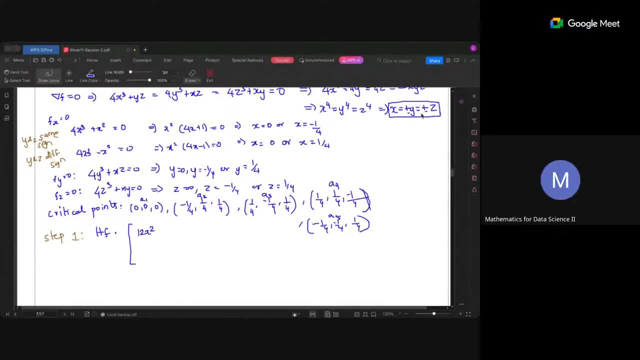 to K right, and then I get to two. they are not equal. they are plus or minus. Y right, they are not all equal. ok, when you do that, it you get 0, 0, 0 minus 2 minus 2. HF of a tail is not all equal. you have plus or minus here, Okay. Okay. So here, fxx is 12x square and 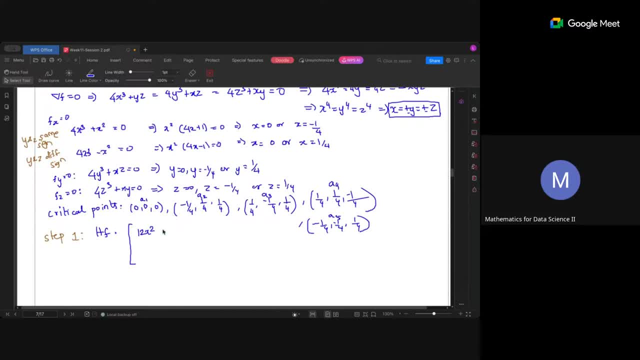 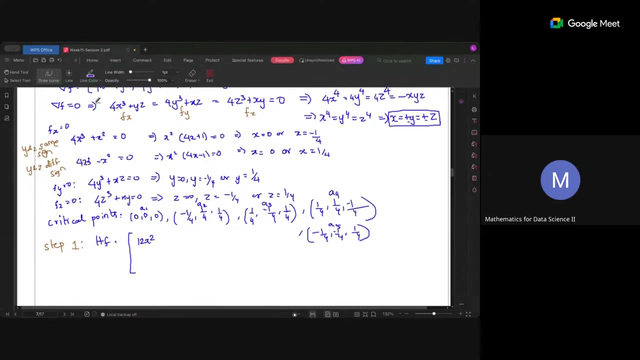 what is fxy? 0, 0.. Careful, What is fxy? This is your fxx. What is fxy Z? Yeah, So this is your fx, fy and fz. So from this you can tell me: So you have, fxy is z and what is. 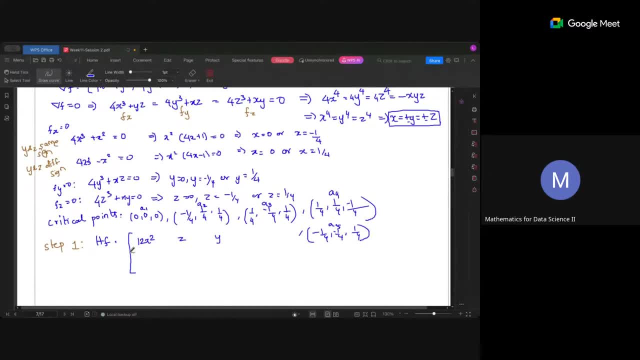 fx Z, Y, Yeah. And what is fyx? It is going to be same z. And what is fyy? 12y square. And what is fyz? X, Yeah. So now, since it is a symmetry. 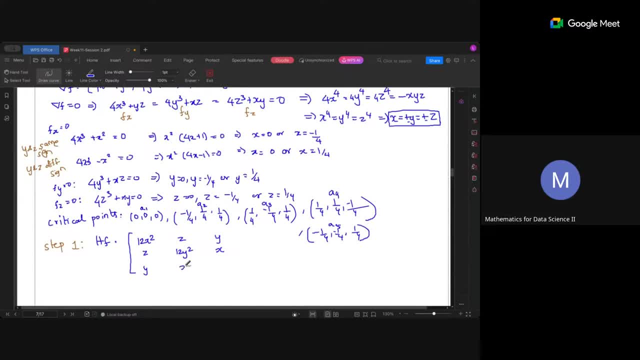 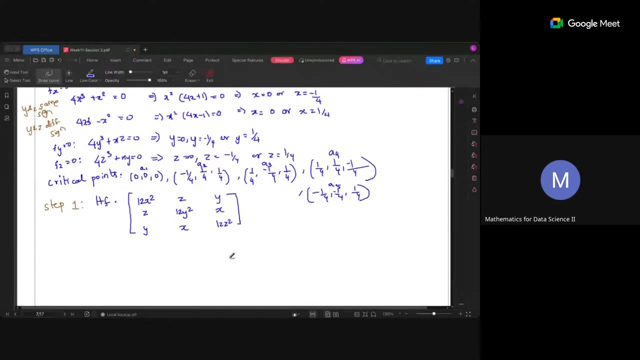 matrix: this is y and this is x. Correct, And what is fzz? 12z square, 12z square. Okay, So now we have to find the determinant at each of these points. Okay, Fine, Let us do. 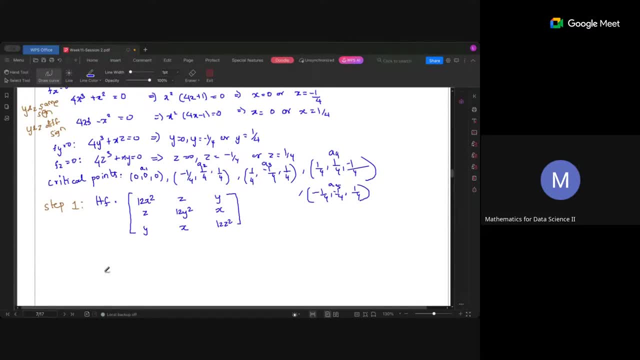 it step by step. Okay, So step two: Calculate and tell me the determinant of hf of a at each of these points. What happens at 0?? 0. 0. So if it is 0, what can you say For a1?? Which case? Inconclusive? Yeah, The. 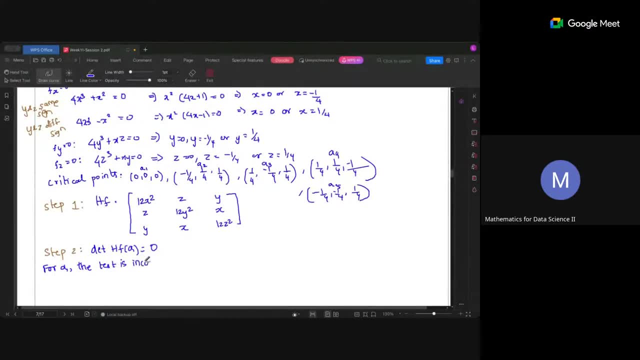 test is inconclusive. What about for determinant of hf at a1, a2?? Calculate and tell me, Minus 1 by 4, 1 by 4, 1 by 4.. What is the determinant? Calculate and tell me. You just have to tell me. 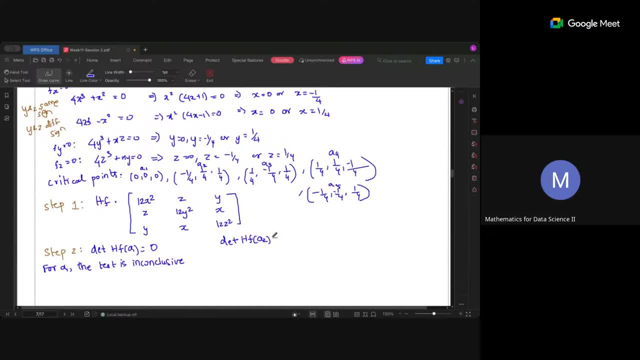 the sign. that's sufficient for us. value is not important, so it is positive, right, okay? what is the value for determinant of hf at a3, positive or negative? 1 by 4 minus 1 by 4. 1 by 4. so it is again. it is positive, right, yeah, so now this is also positive, okay, good. 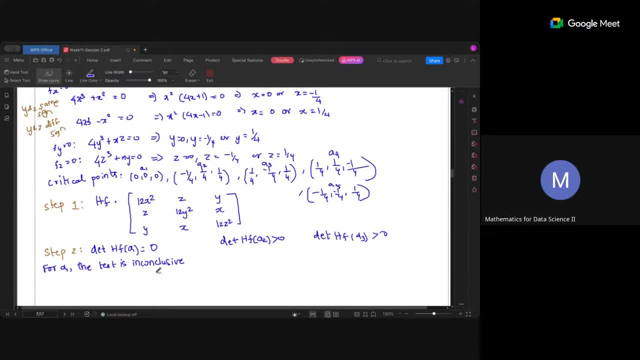 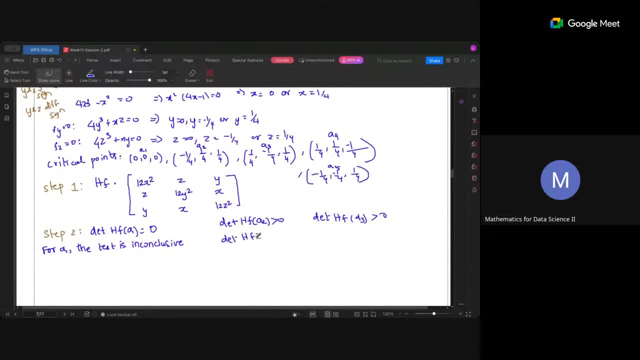 so now these two are positive, so we have to move to the step three for the other two. but anyway, let us finish this determinant of hf of a3 and a4 before step. what about? these two verify this as well. so this is a only a4. 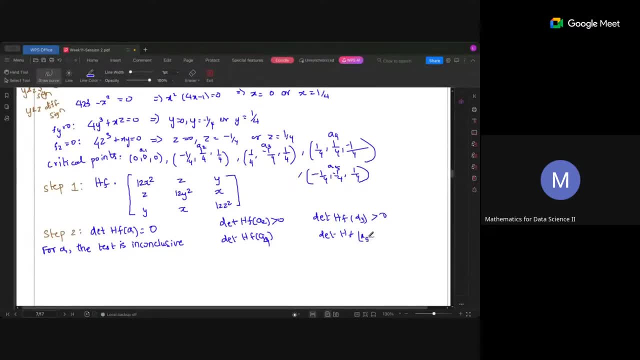 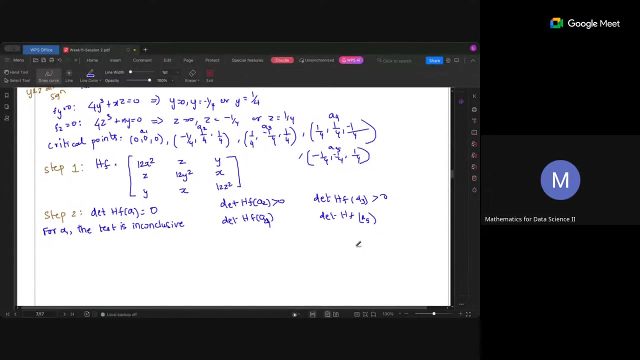 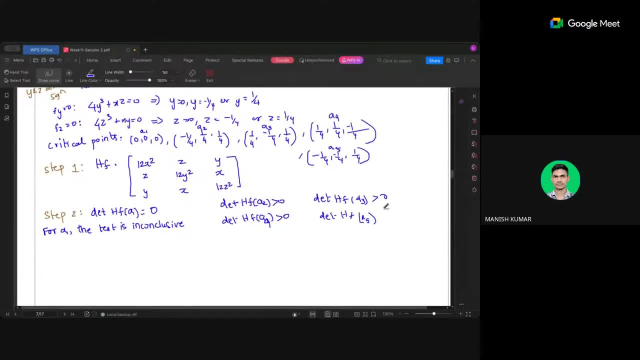 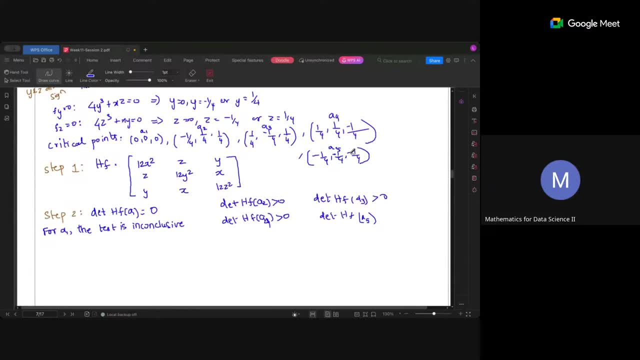 z. sorry, Thank you, Thank you. So now what is step 3?? You have to find what is the value of fxx, fy y minus fxy, whole square at a2, similarly at a3, a4, a5.. 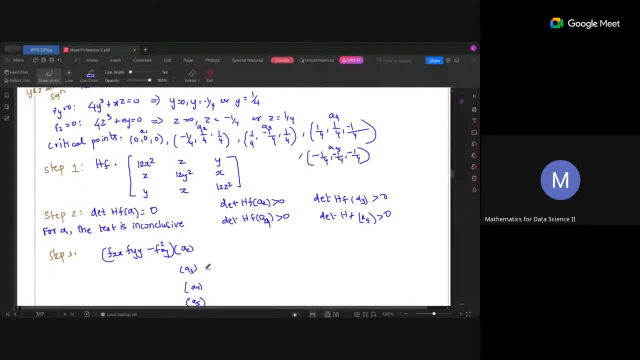 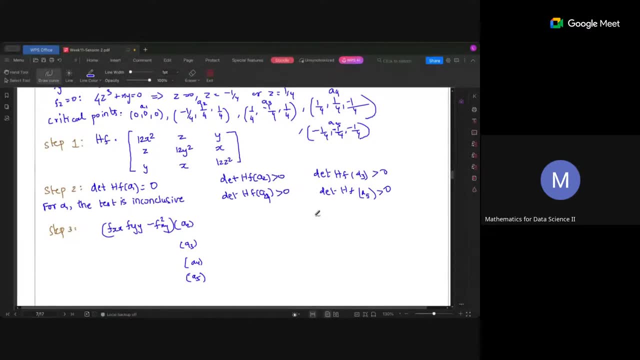 For this you have to calculate, find the signs. So what is fxx, fxx, fy y minus fxy square in general? So it is 144x square, y square minus z square. So this is your fxx, fy y minus fxy square. 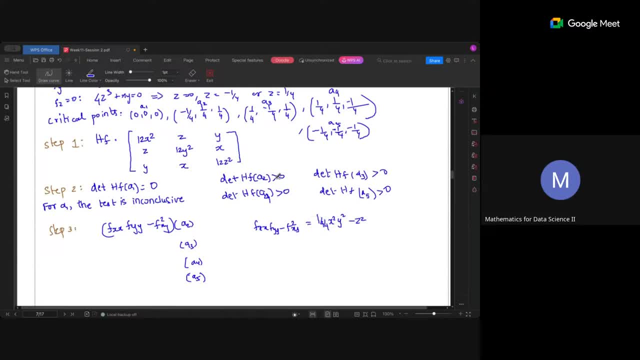 So now calculate the value of this at a2, a3, a4 and a5 and tell me the signs, Since there is a square, irrespective of the sign, this term is going to be some positive term And you have a very huge number here. 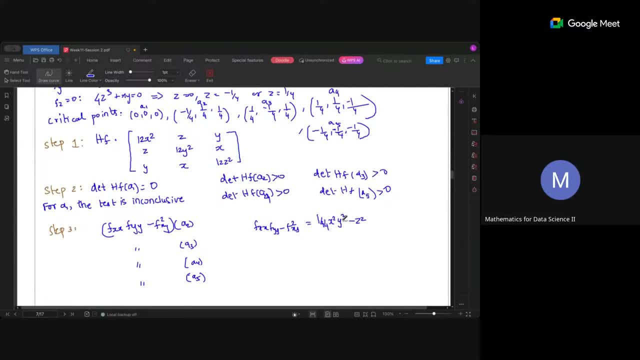 So automatically, can you guess what is going to be the sign? always Positive. Yes, You can easily guess that it is going to be positive. You don't even have to calculate Because you see you have a very large number here And all the numbers are just 1 by 4, 1 by 4.. 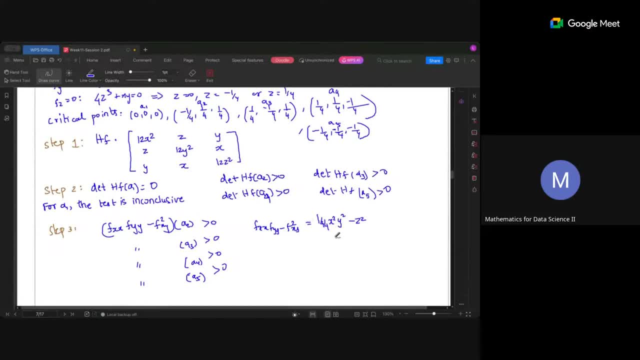 Because there is a square, it is going to be 1 by 16, 1 by 16.. So here you are having a huge number against just 1 by 16 here, Right? So what is going to be the answer? 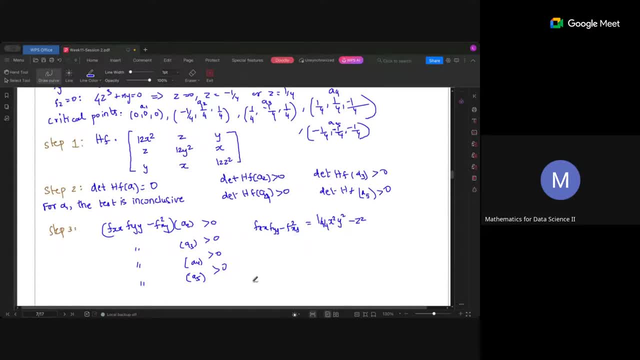 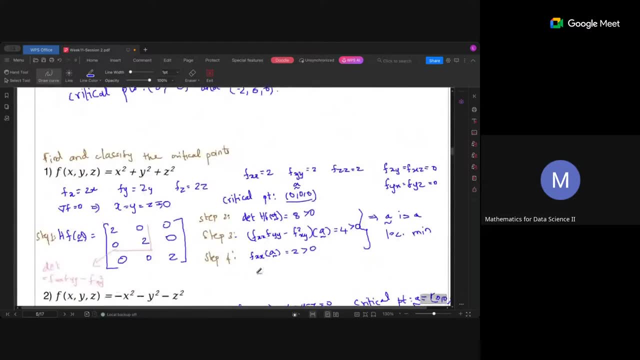 It is going to be positive only. So if all of them are positive, then what can you say? So you have now Step 3 is not going to come in picture, right, Sorry, case 3. Because here you have both positive, positive. 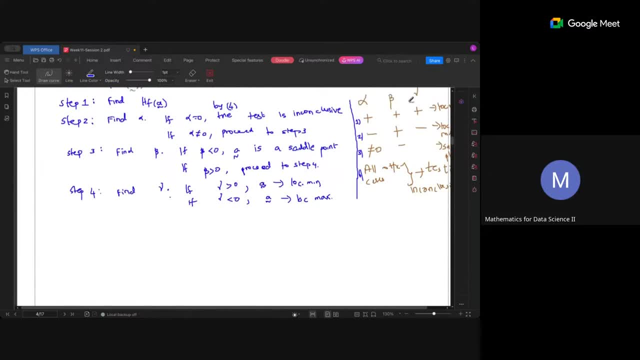 So only thing you have to see is that, whether the last part, gamma, is also positive. So what is the last part, gamma, fxx at a tilde. So now, what is fxx at a tilde? You have to calculate, Calculate and tell me what is fxx at a tilde for a1,, a2, a3, a4?? 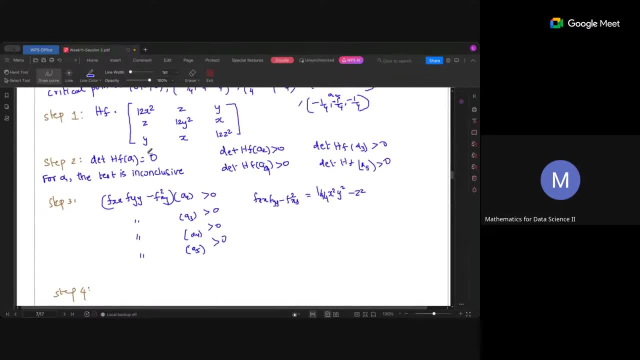 3. What fxx? fxx is 12x squared. So you have Again. it is going to be the same square, same sign, because it is 3 by 4. Again square, Yeah, So a2 or a3, all are going to be same sign. 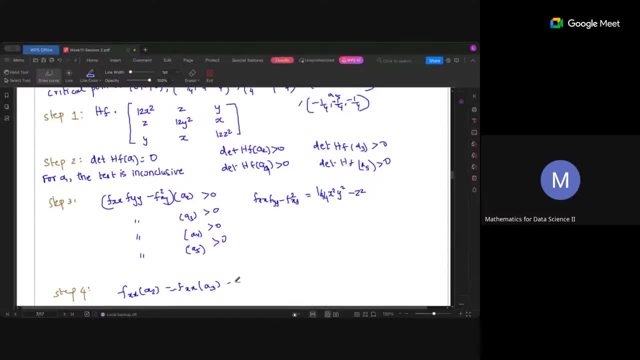 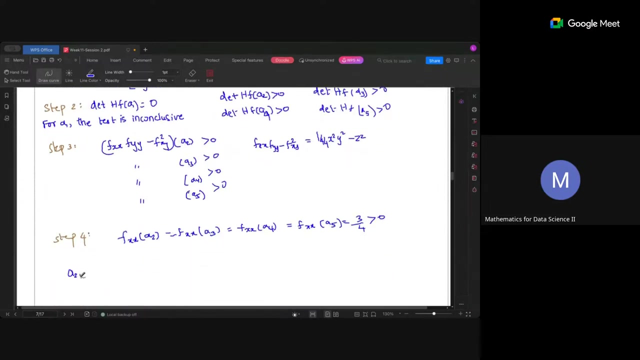 In fact, same value, Right? Yes, ma'am. So fxx at a3. 4, fxx at a5 is exactly equal to 3b4. And this is also positive. So what can you conclude about all the points a2, a3, a4, a5?? 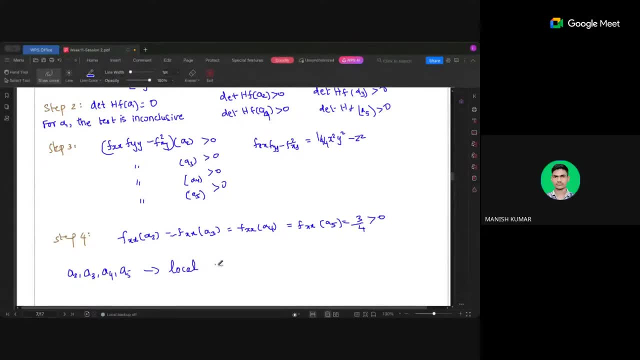 They are local minimum, Minimum. All these are local minimums, Minimum, Right, Okay, So when you have multiple critical points, you have to do the same procedure, but you have to do it for each of these points. Okay, That's all. 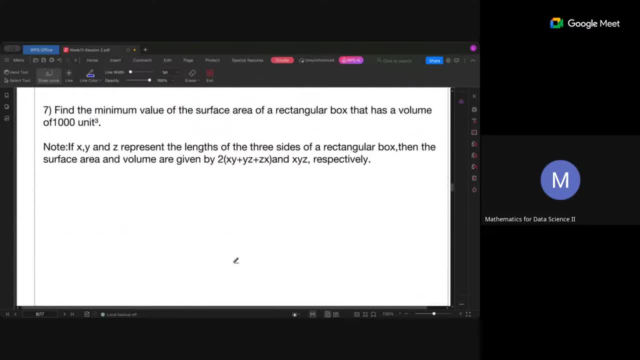 Okay, So now let us do this problem here, So the same problem which we have done so far. we are now having it in a Given in a different way, Slightly in a different way, Okay, So now read the question first of all, everyone. 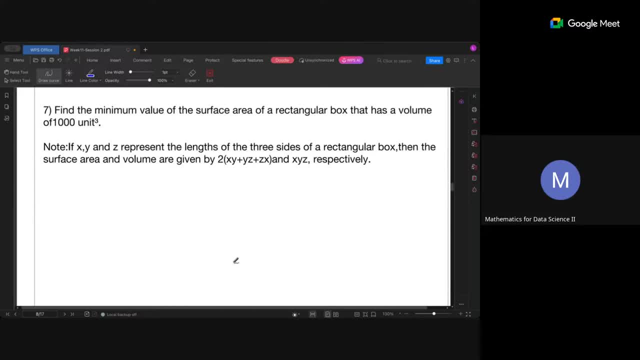 Just take two minutes to understand the question. So what is the function we are considering here? Can you tell me? Can you tell me X, Y, Z? Be careful: You are finding the minimum value For the surface area. so which function represents the surface area? 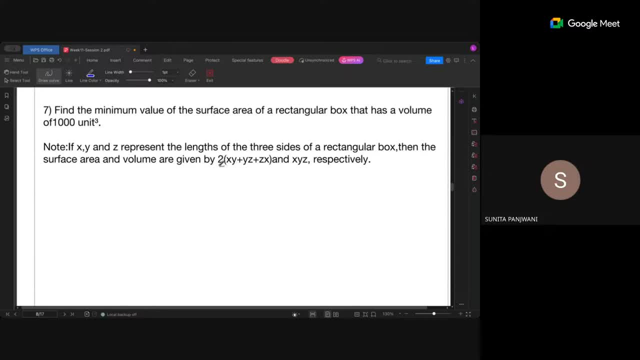 2XY plus YZ. Twice of X, Y plus YZ plus X. So this is what is representing the surface area. It's already given in the note Right. So you see that the surface area. let's call S of X, Y, Z. 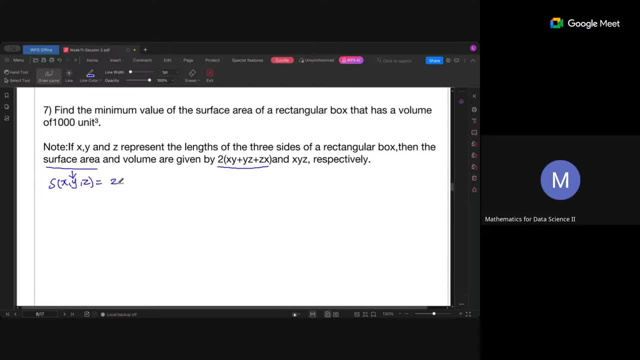 So this is your surface area. It is given as two times of X, Y plus YZ plus ZX. So now we are going to find the minimum value for this. It means we are going to find and classify the critical points for this. 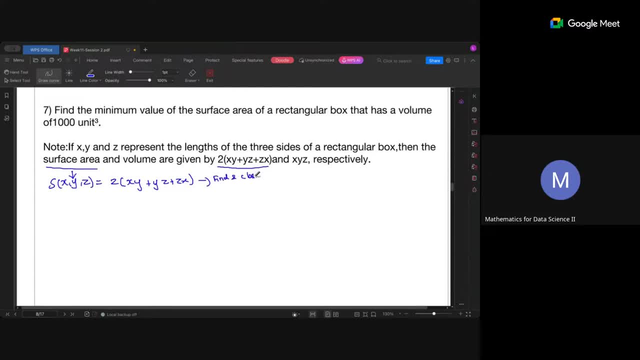 We are going to find and classify critical points for this function. What other information is given? The rectangular box has a volume of 1000 unit. What does that mean? What is the formula for volume? X Y Z. X Y Z is equal to 1000.. 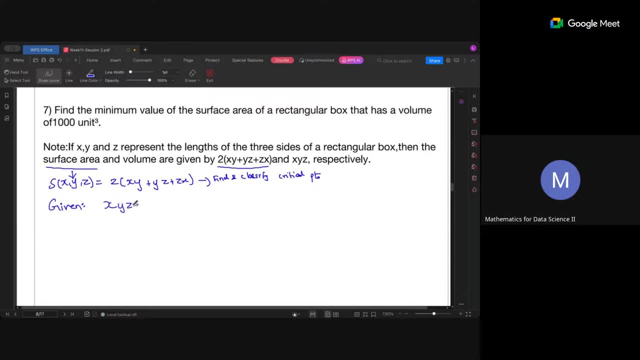 Yes, It is given that X, Y, Z is equal to 1000.. Okay, So now from this, let us try to calculate the critical points. Now for finding the critical points, you have to find what is the gradient of S. 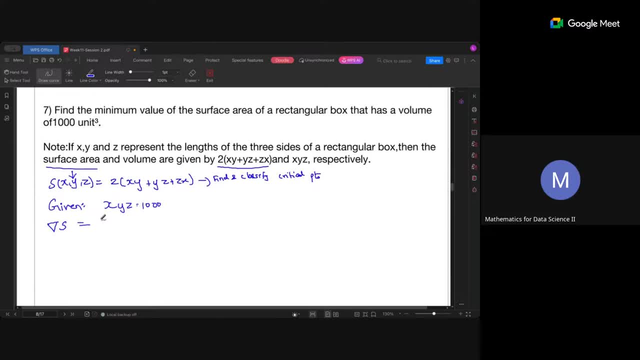 So what is SX? So maybe from this you can reduce one variable So using this given. So if you replace, maybe that with you can replace actually any any one variable. So if you are replacing that with thousand by X, Y, then what happens to your S? S of X, Y, Z becomes two times of X, Y plus Y, Z, Y into 1000 by X. 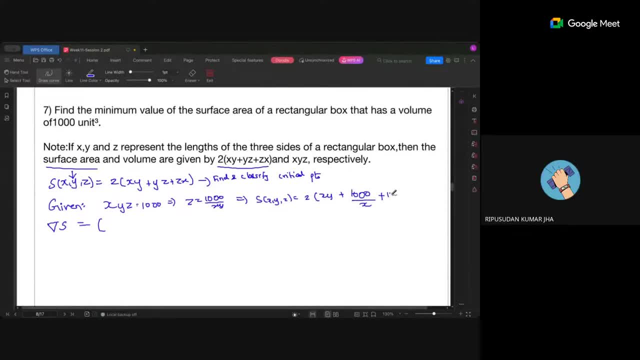 It's simply thousand by X, Right, And then Plus thousand by Y, So this step is not required. Straight away, you write: Okay, So now let us find LX from this. So now, what is what is your SX? What is your SX? 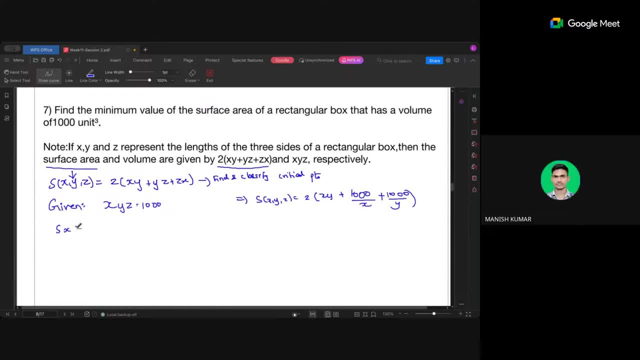 Minus thousand by X. so first you have two times of y and then you have minus thousand by x square, minus thousand by x square. so you will have a two here that will get cancelled with this two, okay. similarly, what is s y, what is s y two? x minus thousand by y square. x minus thousand by y square. 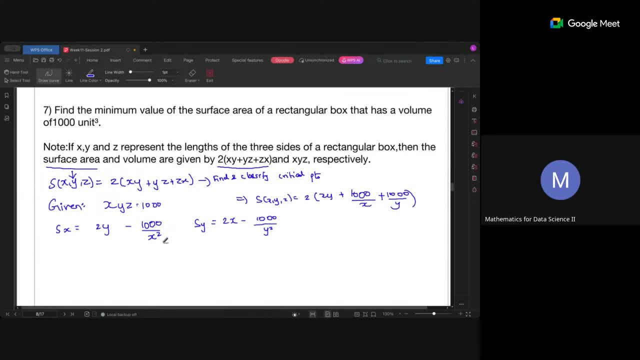 all, right now, if this s x is equal to zero, what was? what is that you are getting? so if s x is equal to zero, you get two x squared y, and then you have minus thousand by y square minus thousand by y square minus thousand is equal to zero, which gives you: 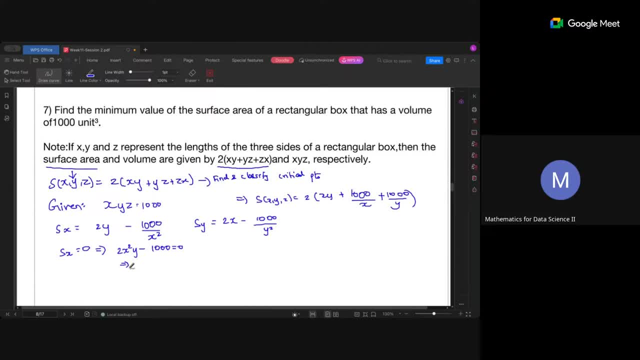 x squared y is equal to 500, so there is a, so this two, um, one by x is here, so one by x means you will have. so is this two getting cancelled? did we do it correctly, or is the two still there? so you have one by x. so what is the derivative of one by x with respect to x? 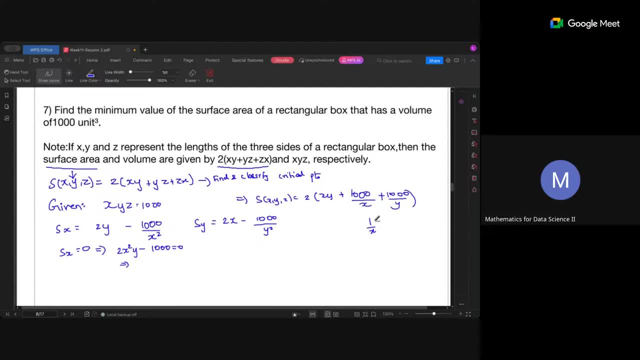 it's minus two by x, squared right. yes, so there is a two here as well, not in the denominator, in the numerator only. we are getting the two, so we are having a two here as well. so this is actually two thousand here and here, correct? yeah, yes, ma'am. 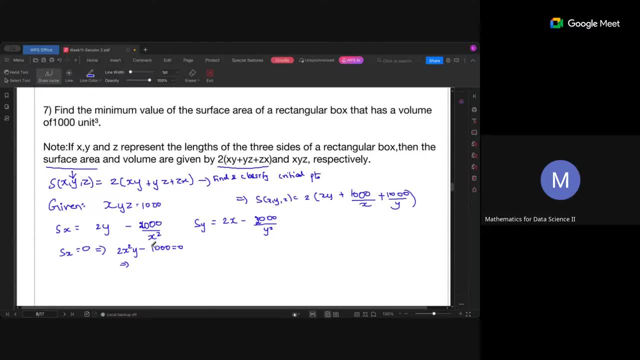 yeah, so then you have: yeah, so now x squared y is equal to thousand. similarly, s y is equal to zero, will give you two x y squared minus two thousand, equal to zero, which means x- y square is equal to thousand. okay, so now you have: x square y is thousand, x y square is thousand. so this is: 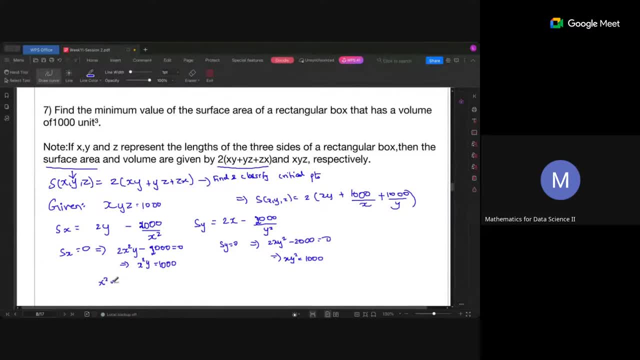 any. now now, χ ut means x square, y is equal to x- y square, correct. now what does this mean now? what is this mean? square y minus x y square is equal to 0. now, taking the x and y commonly, what is left? x minus y- y. 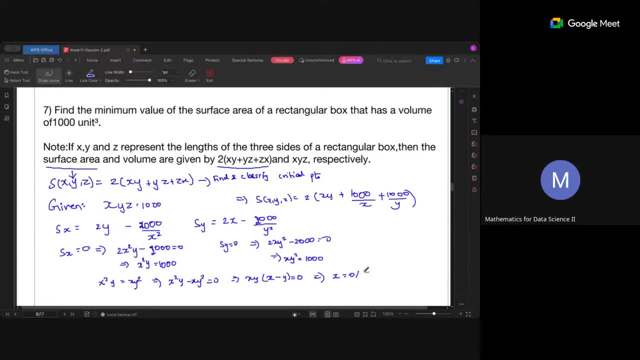 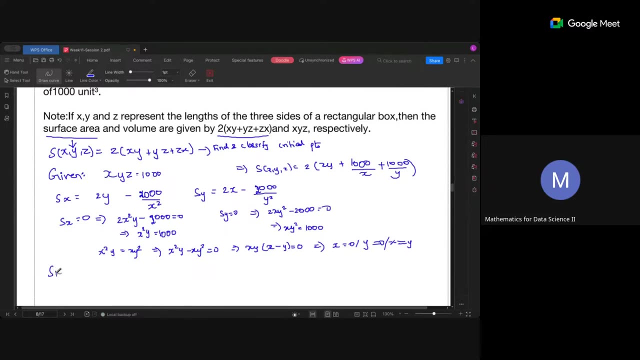 y equal to zero, or x equal to y, x equal to y, y. all right now. is it possible that either x or y is zero, because you have x, y, z is thousand? since no, x, y, z is equal to thousand, x equal to zero or y is equal to zero is not possible. 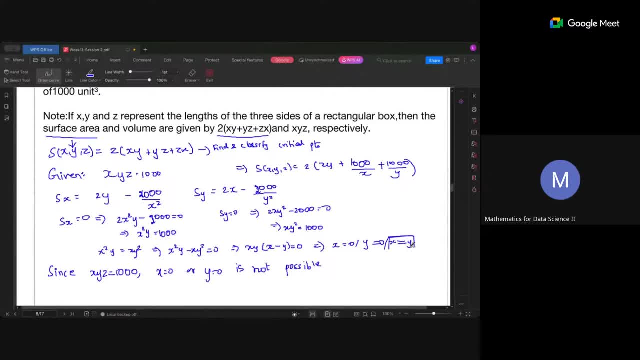 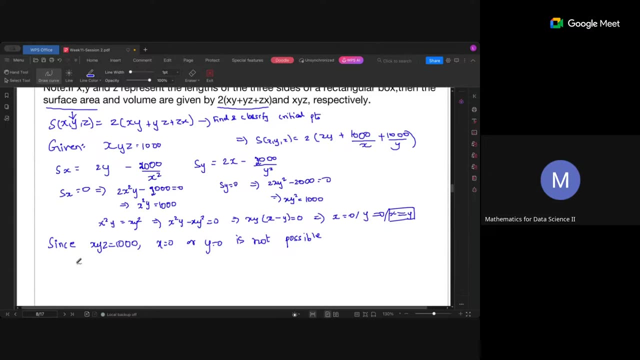 so what is the only case? we are left with x. we are only left with, yeah, we are only left with: x is equal to y. okay, now from here? now, what is that we can tell? now, x square y is equal to thousand. now, if x is equal to y, what do you get? 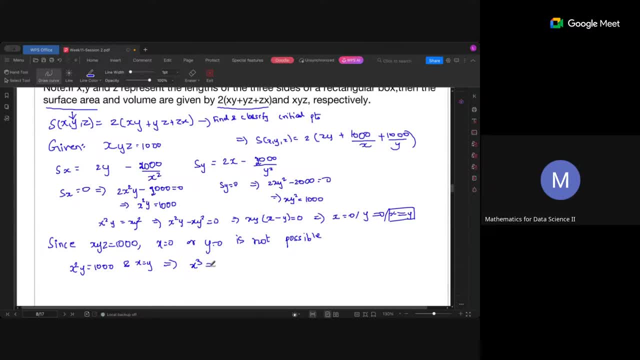 so what do you get? x cube is equal to thousand. so if x cube is equal to thousand, then what do you get? if x is equal to 10 and x is equal to y? so this implies: okay, now z is equal to. now you know that z is equal to thousand by x- y. so what is your z then? 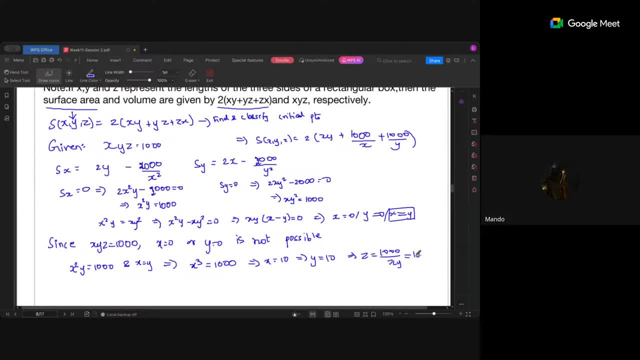 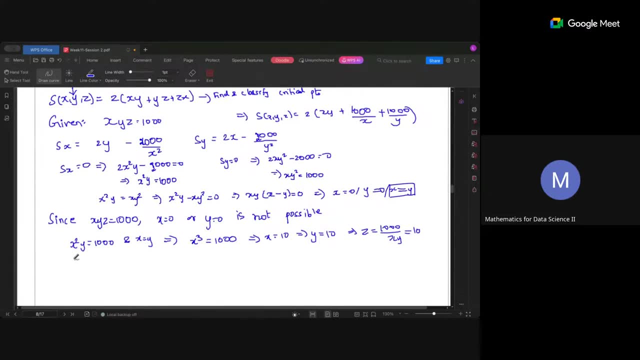 also 10. right, so your x, y, z, all are 10. okay, now, what is your hessian test? saying so, first of all, now, this is a critical point for us. right now, this is a critical point for us: 10, 10, 10, 10 comma, 10 comma 10 is a critical point for this function: s. or, if you are just 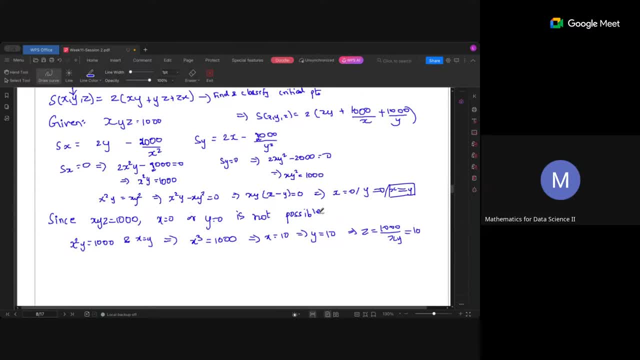 considering it as a function of two variables, x and y, then 10 comma 10 is a critical point for this. here I can remove the z, okay, considering as a function of two variables, So considering it as a function of two variables. so for this only 10 comma 10 is a critical point. 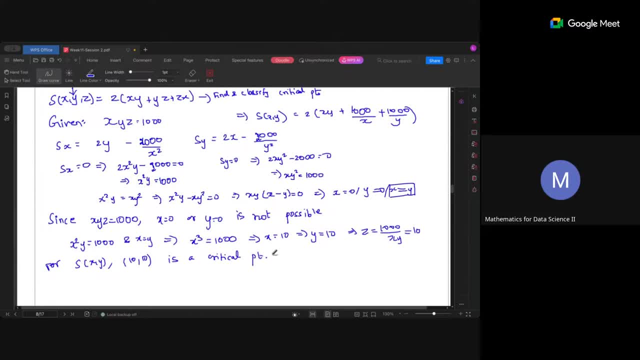 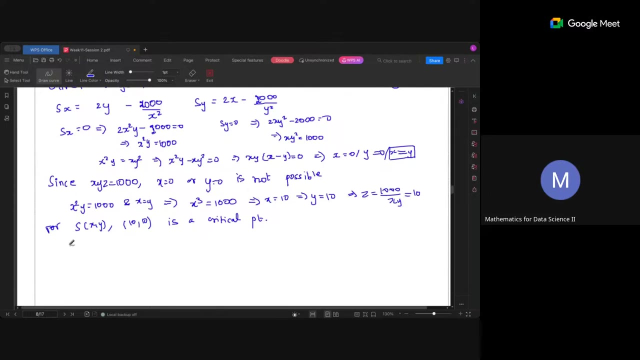 okay. So now this is a critical point Now for functions of two variables. how do you find the classify, the critical points? You have to anyway find the Hessian matrix. What is your Hessian matrix? So for that you need to know what is SXX. 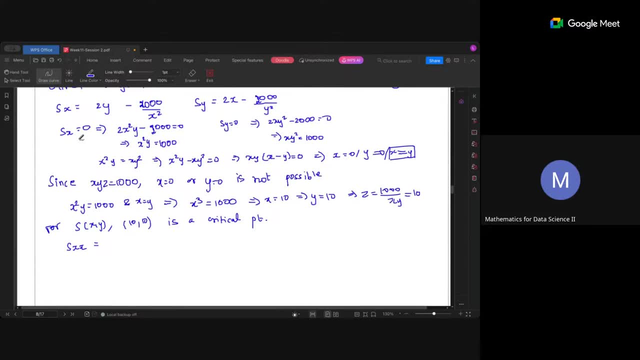 SXY and XY. So what is SXX? So this is your SX. What is SXX? The first term becomes 0.. What happens to the second term? So 6,000 by X cube Minus 2,, 2,000 by X power 3,, which is 4,000 by X cube, correct? 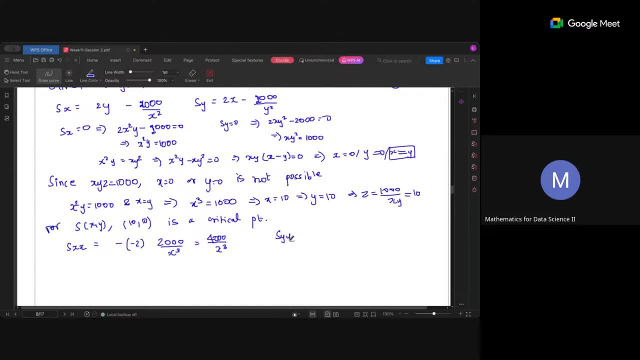 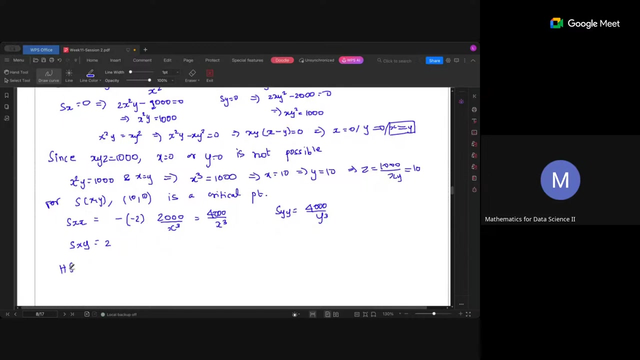 Yes. And what is SYY? Similarly, 4,000 by Y cube. right Now. what is the value of SXY? 2, right. How many is this? 2, right. So now, what is your Hessian matrix? HF? 4,000 by X cube. 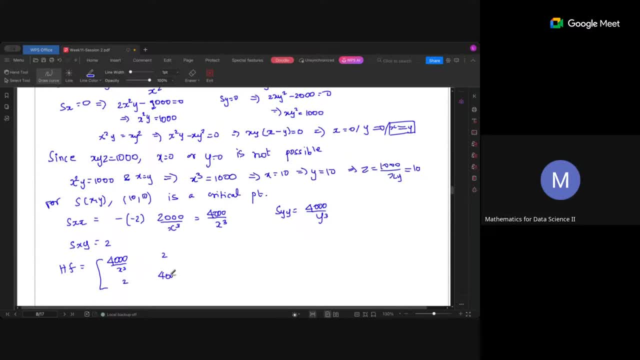 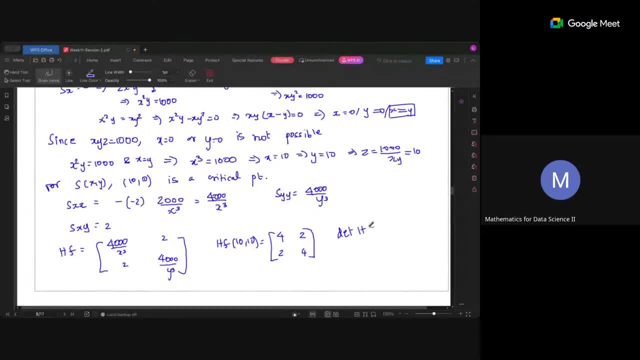 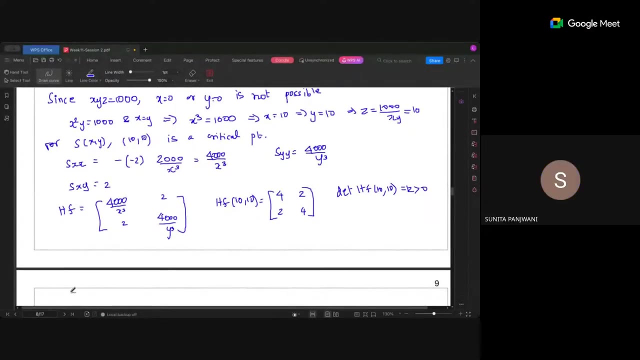 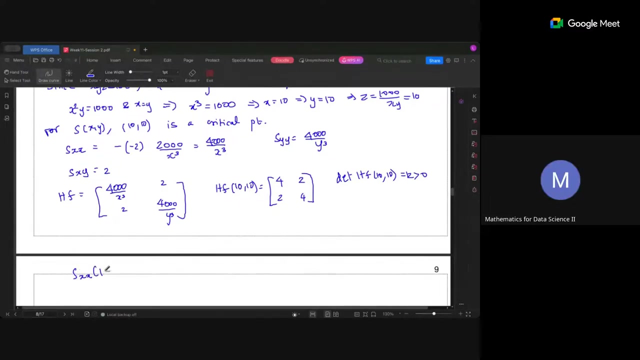 is the determinant of this? matrix 12, which is positive. okay, so now what is the next thing we have to find? we have to find fxx, sxx at a tilt. so what is the value? sxx at a tilt is again just 4, which is positive. so now, both of these are positive. what does this mean? 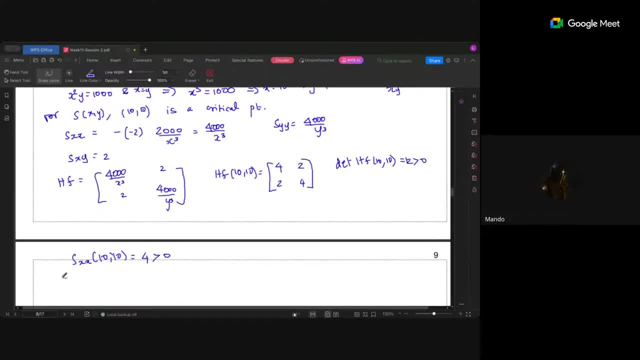 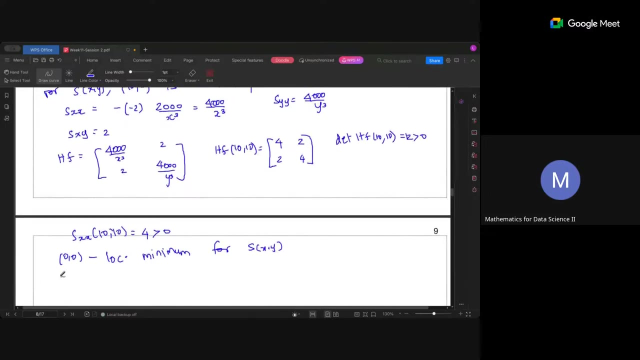 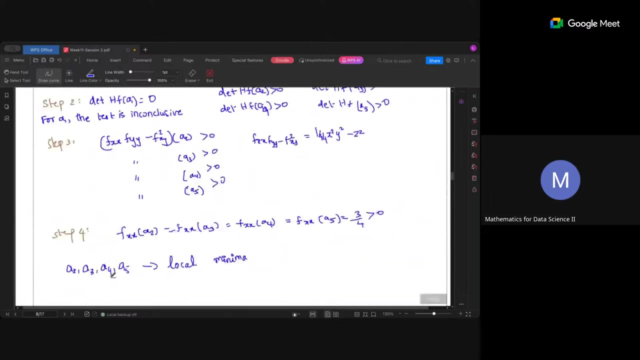 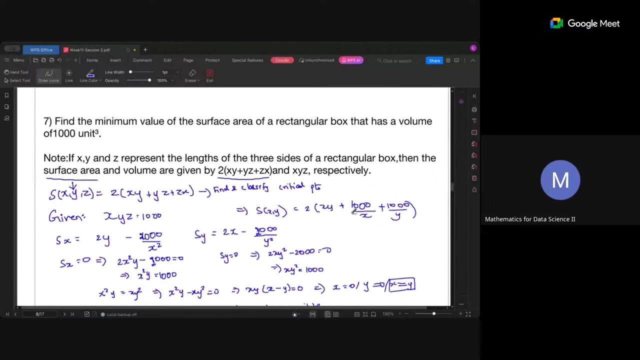 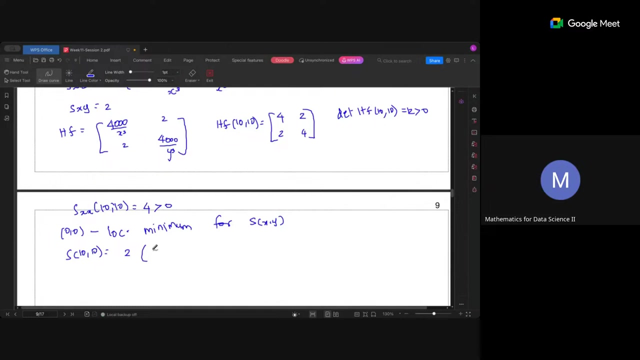 it's local local minimum. 0, 0 is a local minimum for s of x comma y. so now, what is the value of s of 10 comma 10? that is, that will give you the minimum value. right. what is the minimum value? 0, 0 is what they are asking. so we need to calculate what is s of 10 comma 10. so if you put 10, 10, 10 here, what is that? you are getting 2 times of hundred plus. 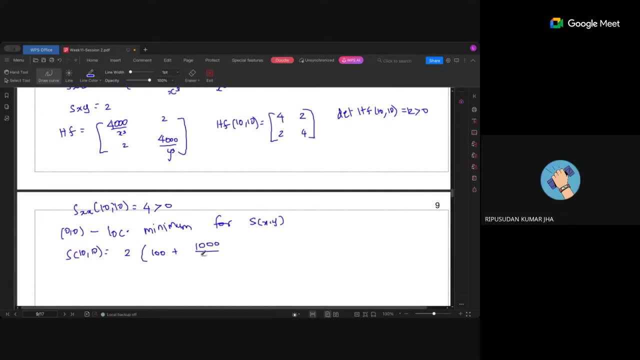 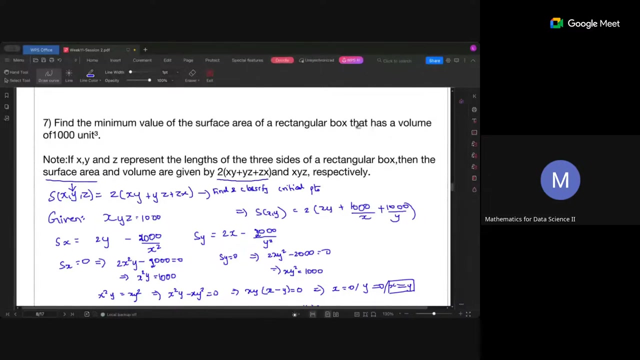 1000 divided by 10 and 1000 divided by another 10. so when you simplify 2 times of hundred plus hundred plus hundred, so what is your answer? hundred, six hundred. so the minimum value of the surface area of your this box rectangular box, has 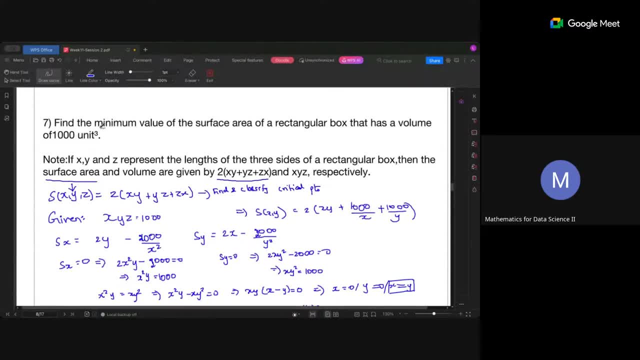 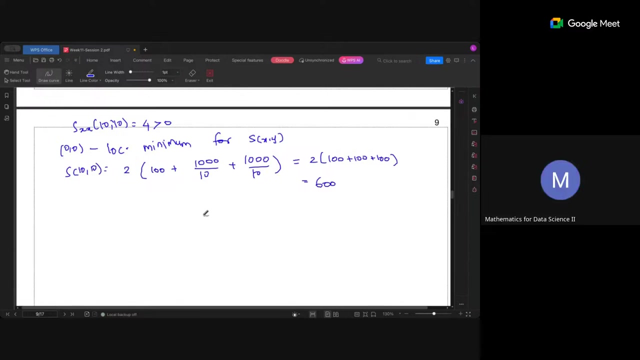 a value volume of a thousand unit cube. so what is the minimum value of the surface area? 600 units. okay, so this is the answer. is that clear? yes, sir, how did we get the answer? okay, okay, so instead of considering it as a function of two variables using the given info, three variables using the given way, 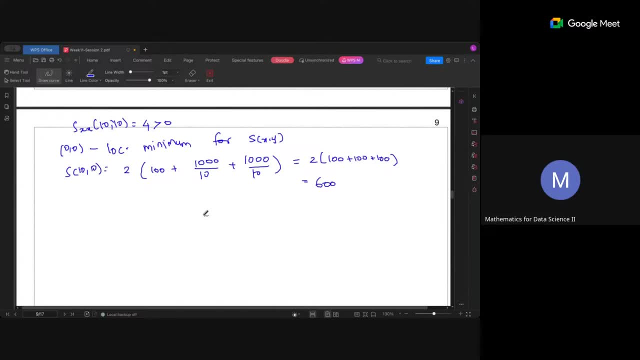 information. we reduced it to a function of two variable to simplify our process. that's all okay. consider a function: f of x comma y comma z, given information this way, if a is the hessian matrix of f of x, comma, y comma z, at this point we have to find: 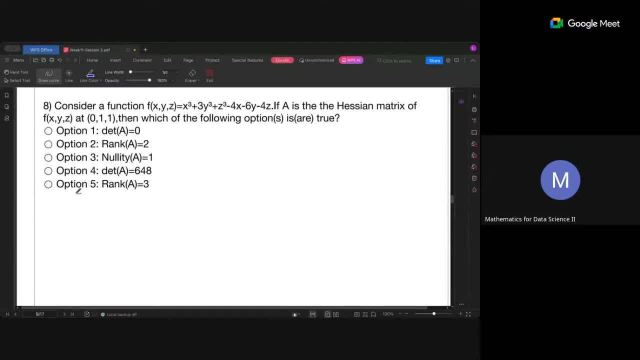 these things. so we have to basically find what is the hessian matrix. so first let us write what is fx. what is fx for this function? three, three x, four minus four? and what is fy? nine, nine y squared minus six. and what is fz? three, x squared square three, three, q square, yeah, nine is four. now what is fxx? 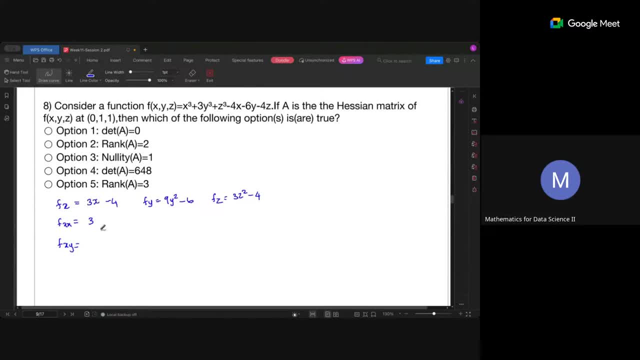 okay, and what is fxy zero? and what is fxz zero? now, what is fy1? well, and what is fyz? and what is fzz? uh, is this sufficient to construct the hessian matrix? uh, yes, yeah, so hf is 318y 6x那么 недóxие hfť18y6z. 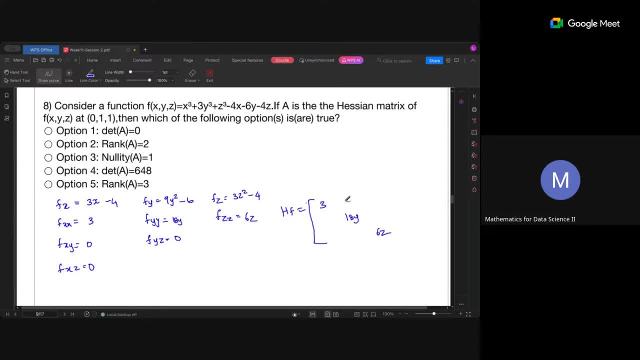 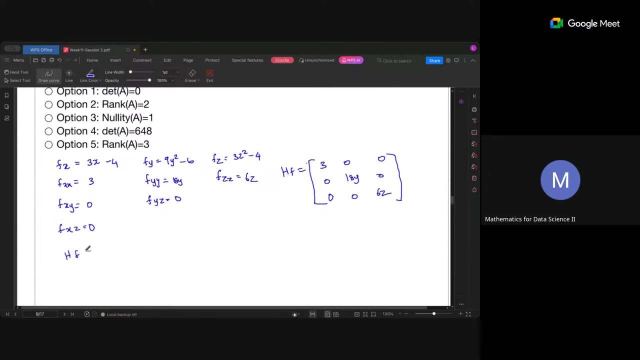 and then you have, and then you have: X, Y is 0, X Z is 0, Y Z is 0. okay, now, what is the Hessian matrix? at 0 comma 1 comma 1. so now, what is the determinant of this matrix? calculate and tell me. 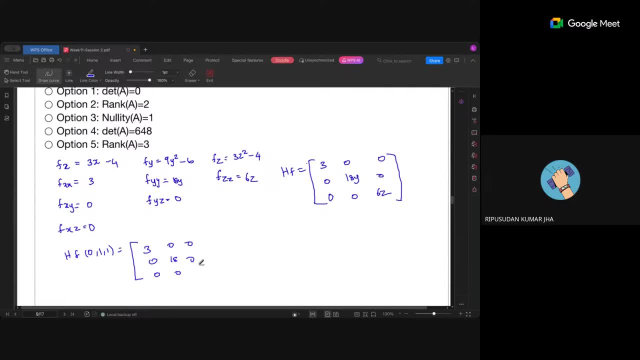 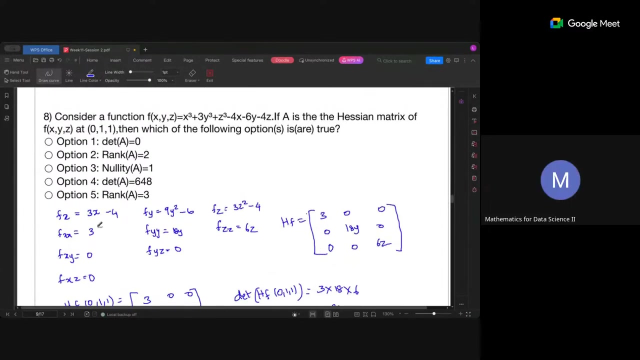 six, four, eight. so determinant of HF at 0 comma, 1 comma 1, it is a diagonal matrix. so how do you calculate the determinant? multiply the diagonals 18 into 18, 324, remember, FX is 3, X is square, right I think? oh yeah, here I missed a square. so 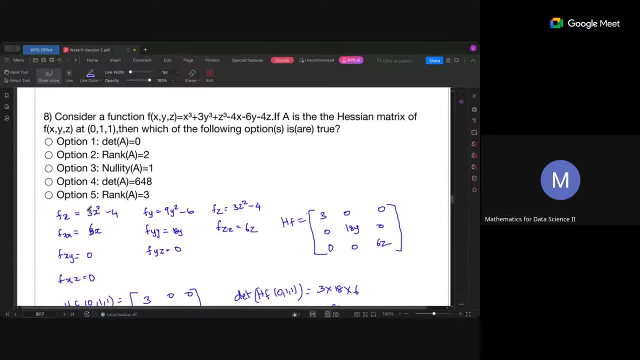 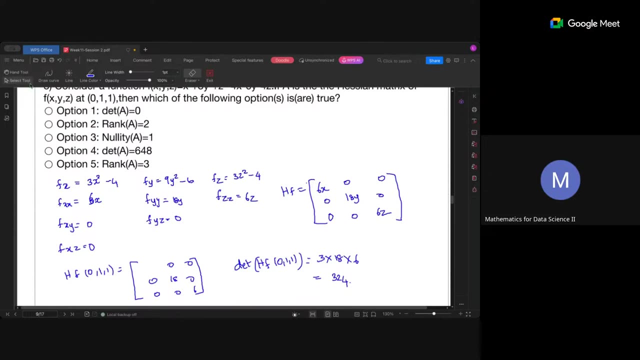 here it is then 6, 6. right? FX X is 6 X. sorry, here it is 6, 6. so if it is 6 X, then at 0 comma 1, comma 1, this value is becoming zero. see how one small mistake is affecting the anterix. so there, stagnant is. 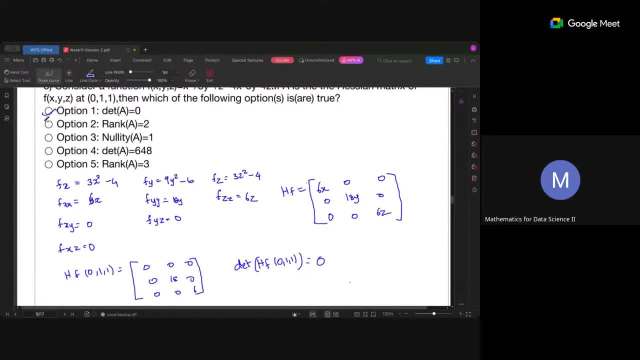 zero. so option 1 is correct. what about the rank 2? so for diagonal matrices, how do you calculate the rank? number of non-zero elements. positive number of not not one molecule. regular number, qd matrix. number of non zero element. positive number of not necessarily negative elements. positive number of nonzero elements. positive number of not necessarily 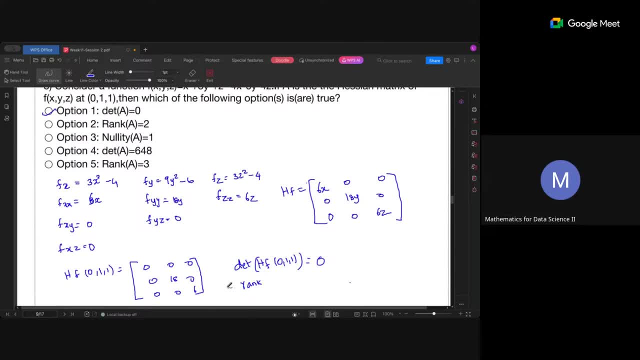 positive. it can be positive or negative, so just see how many number of non-zero diagonals you have. that is the rank of the matrix. okay, for diagonal matrices. so rank of a is 2. this is the answer. if rank is 2, what should be the nullity for the 3 by 3 matrix? 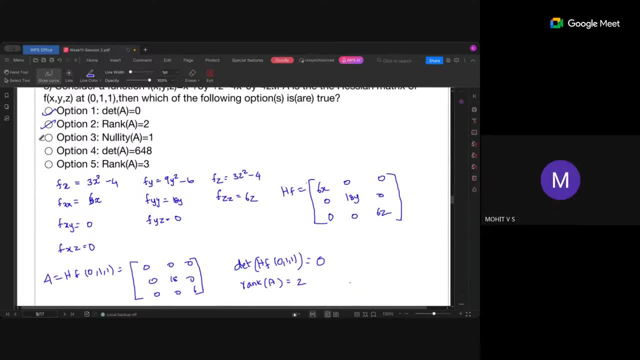 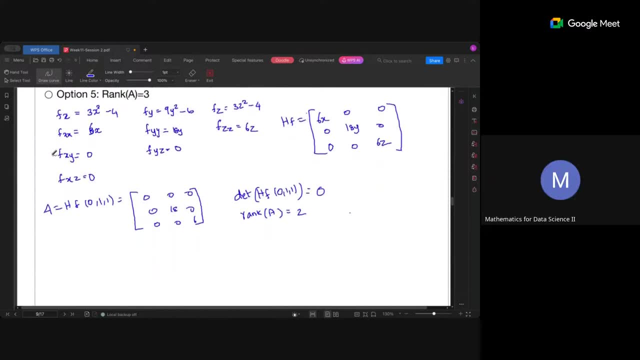 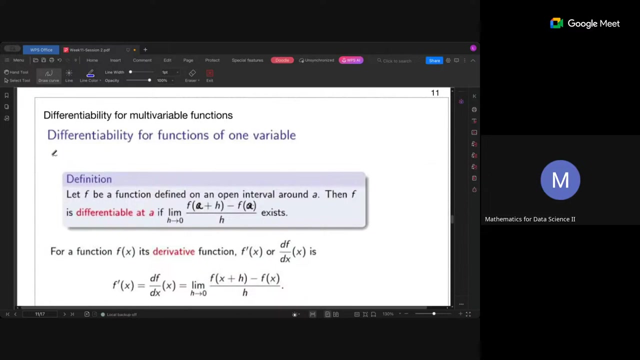 yeah, okay, very straightforward question, only okay. so what is after this? we are almost done with this unit. just this last definition is there. but don't worry too much about this definition. this is just for knowing purpose only. you don't have to worry about problems from this differentiability of four multivariates. 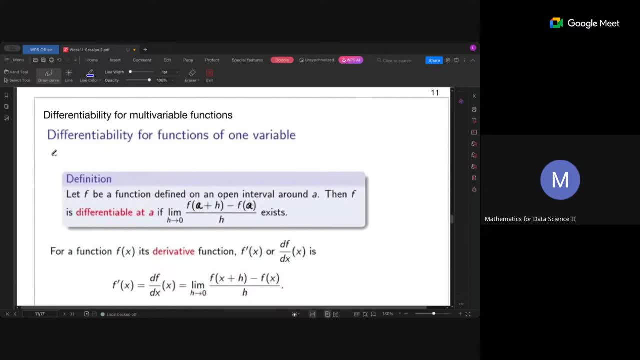 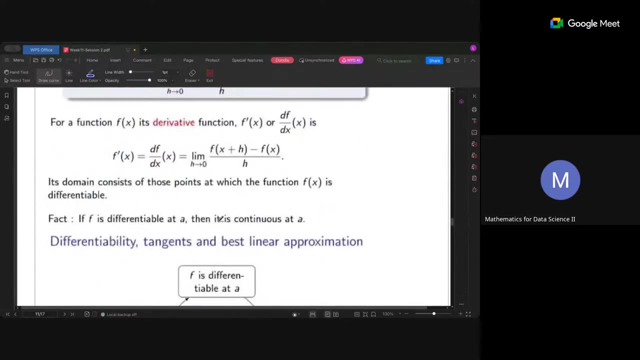 okay, so what is differentiability? first of all, for one variable function. you know that you say a function is differentiable at a if this limit exists, right. so limit h goes to 0. f of a plus h, minus f of a by h exists. okay. and what do you know in? 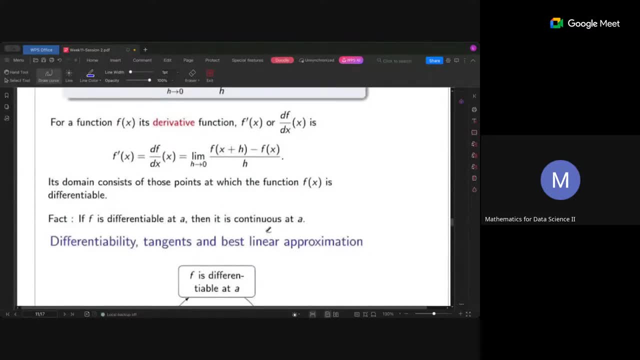 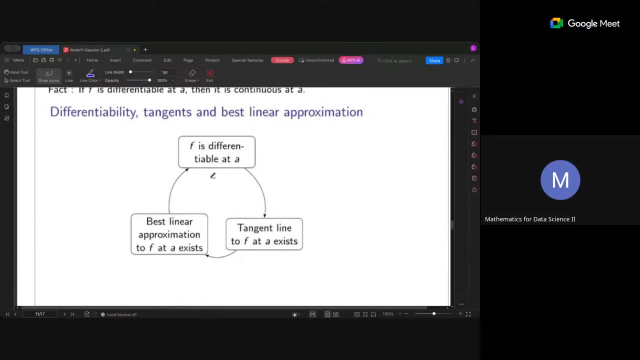 general, if f is differentiable, then you say that f is continuous at a. so this is what you basically study about: differentiability of one variable function. now what you also see for differentiability of one variable function is that. so if you see that one function is differentiable at a, then it means that the tangent line of f at that point 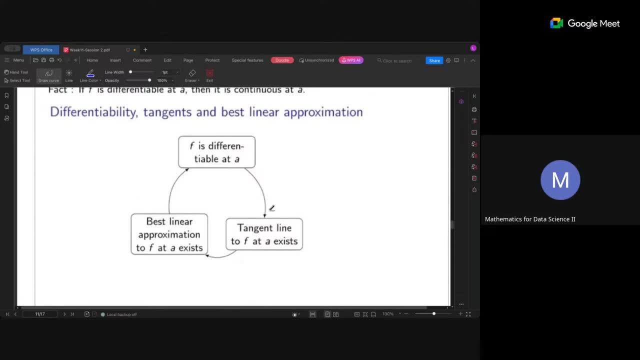 exists. okay, and we also have seen, even in a multivariable case, tangent and best linear approximation are just the same. they are not at all different, even for multivariable functions. right, so the same is the case for one variable function as well. okay, so the tangent and the 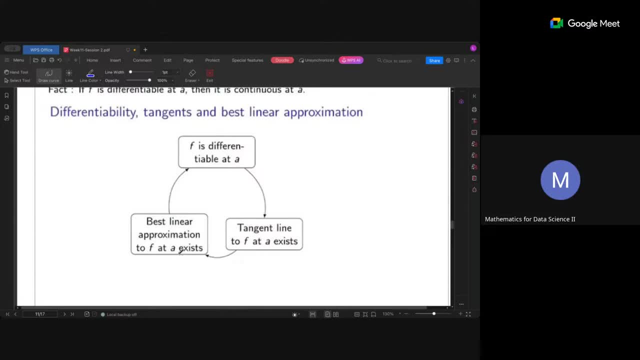 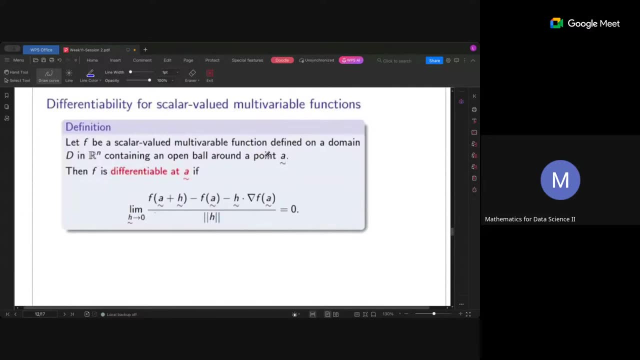 daqui, variable functions are exactly the same. now, how do we get the differentiability for this, uh, multivariable function? how do we get this definition? so now, just let us observe what is happening in the case of one variable. okay, fine, so now what is the definition given to us? the definition given to us is: f is differentiable at a positive. 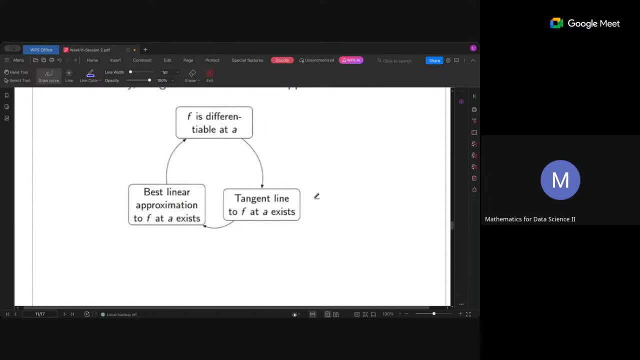 height. so there is never any difference between one and the other variable function. now the definition given to us is in can say in general, this is: and struggled to find theumb, favops is veryaph これ. F is differentiable at A. What does mean by F is differentiable at A? 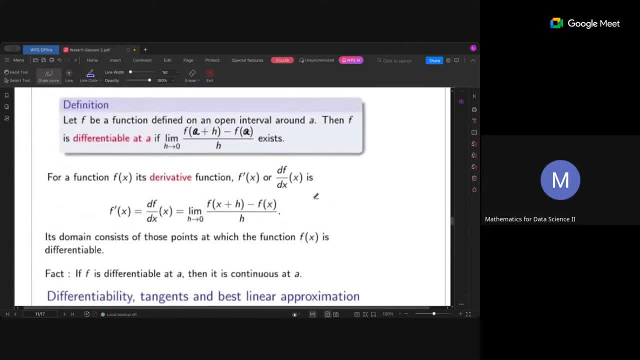 From this above definition itself. you see, This is what is given to you, right? So you have limit. H goes to 0.. F of A plus H minus F of A by H is 0.. So this is what F dash of A. 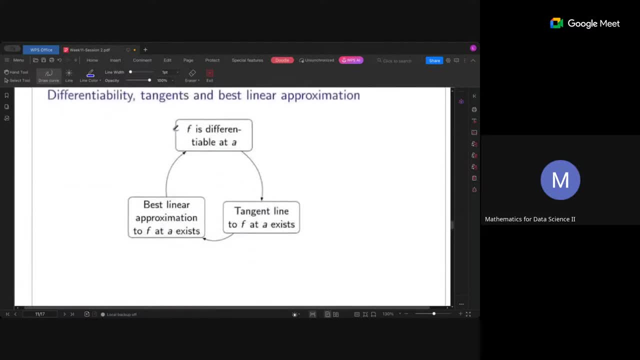 F dash of A is equal to this, So let me just write the same here. So F dash of A is limit H. H goes to 0.. F of A plus H minus F of A by H. Okay, Now we can rewrite it as: 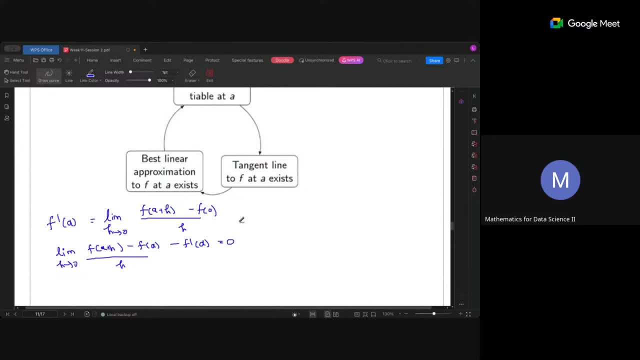 Correct, This is okay. I have just brought this to the other side, Is that okay? Now I want to bring this inside the limit And also bring the common denominator as H. How do I do that? How do I do that? 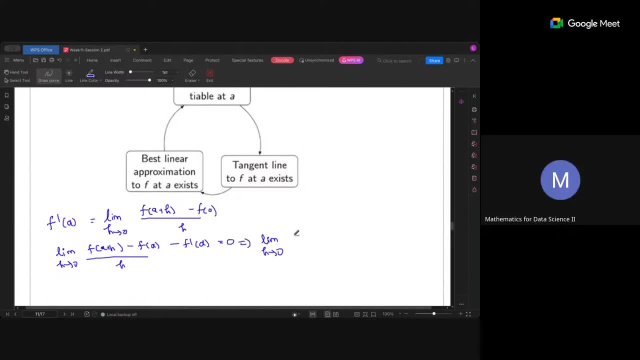 Multiplying it by H, Multiplying and dividing it by H. So you get F of A plus H minus F of A minus F H times F dash of A F of A whole divided by H. Okay, So this is 0. 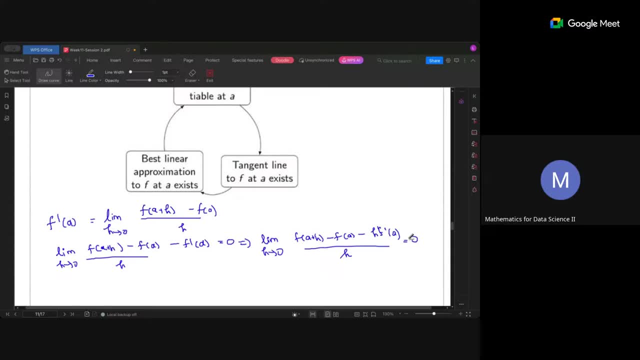 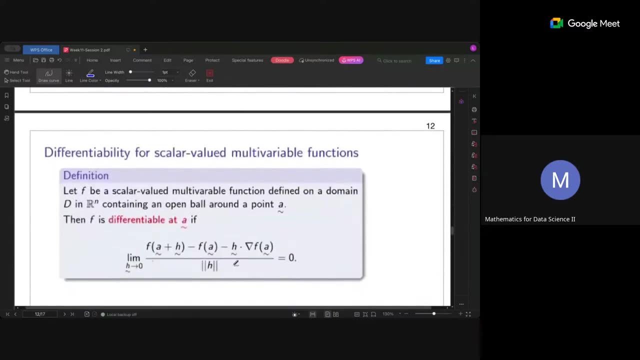 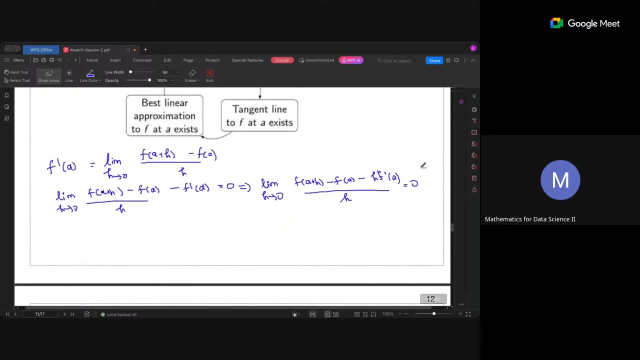 Okay, Up to this is it fine. Yeah, Yes, Okay. So now let us compare it with what is given here. Limit H goes to 0. F of A plus H minus F of A minus H times. Here we have H into F dash of A. 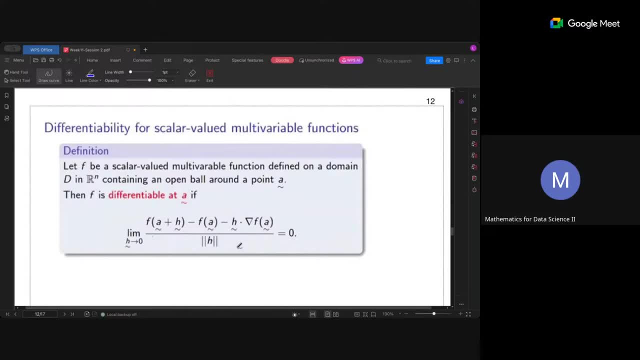 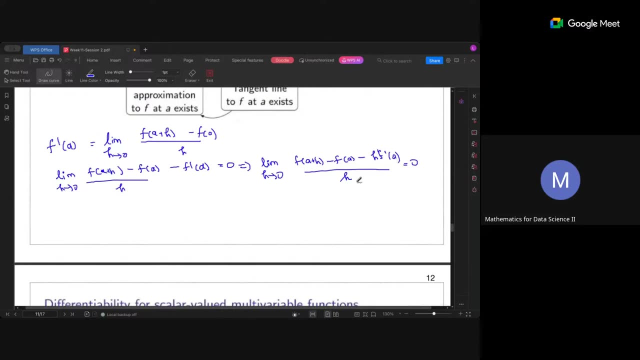 Here we have the dot product of H with the gradient function Dot A, And instead of just H here, because all these are just real numbers. just putting H does not make any problem here, But if you just put H here, so all these are now scalars. 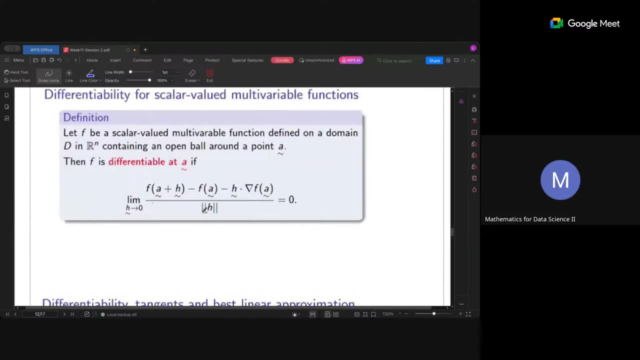 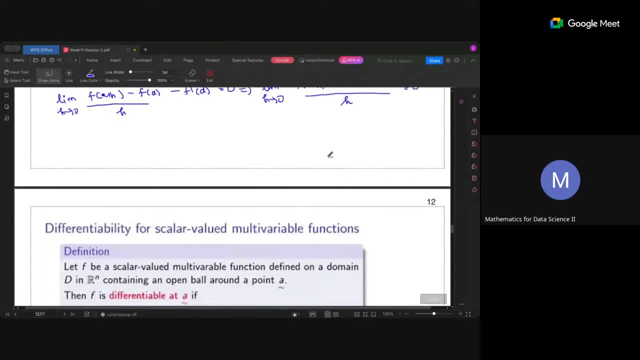 And this will be a vector. H is something like an N variable, right? So you need to consider the norm here. So you see a similar thing we are getting here, Okay. So this equation don't think it is some alien equation. 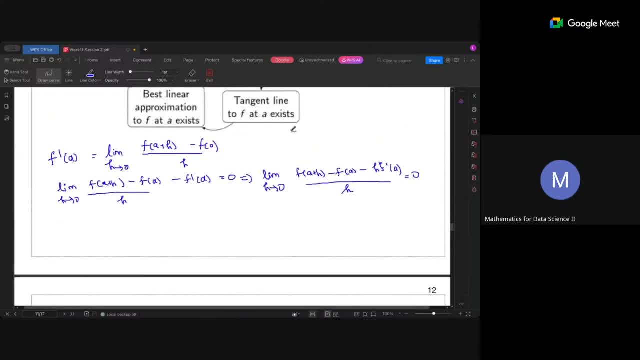 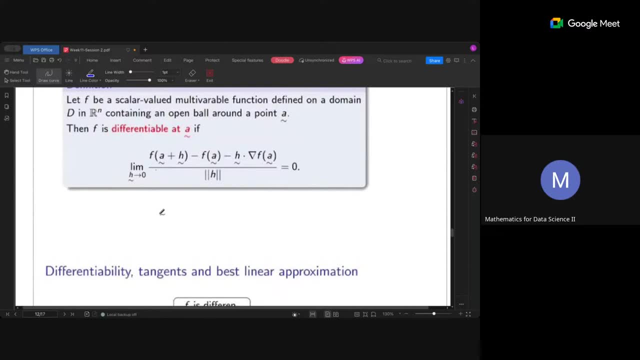 It is something You can relate from the basic definition of differentiability. Okay, So this is what is exactly: F is differentiable at A, So this is much, much stronger than what is you see for partial derivative or directional derivative. 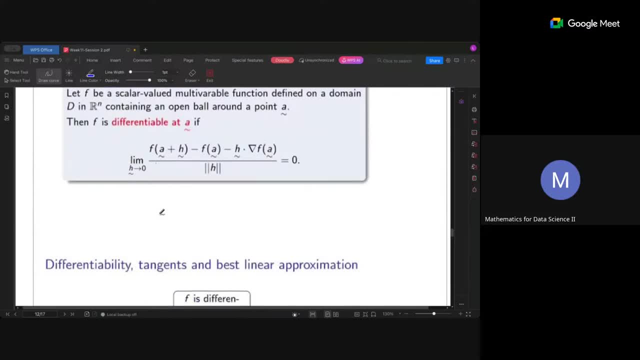 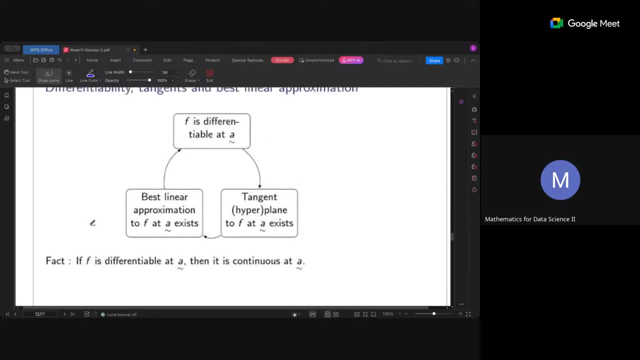 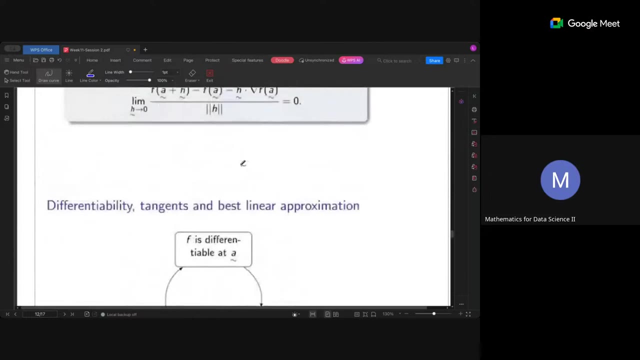 This is much stronger than that. Now, this guarantees you the continuity at A. If F is differentiable at A, then it is continuous at A And you also have all this equality. So this is just something you should know. Don't worry too much about this.